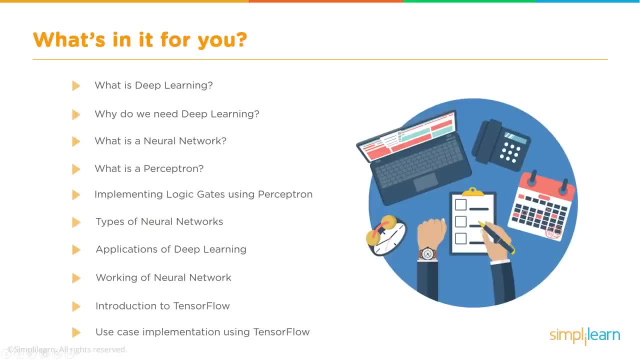 So that's the way, a little bit under the hood, how it works. So what are we going to do? In this tutorial, we will see what is deep learning and what do we need for deep learning, And one of the main components of deep learning is neural networks. 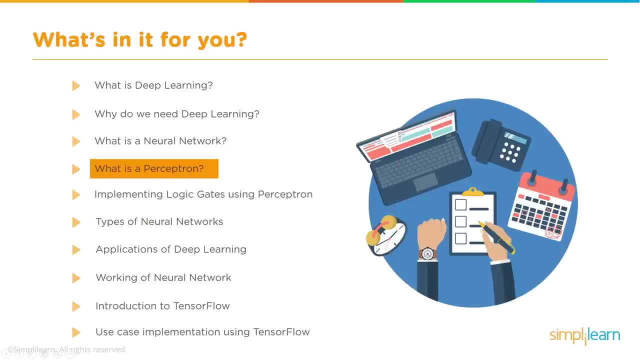 We will see what is neural network, what is a perceptron and how to implement logic gates like AND OR, NOR and so on using perceptrons, The different types of neural networks and then applications of deep learning, And we will also see how neural networks works. 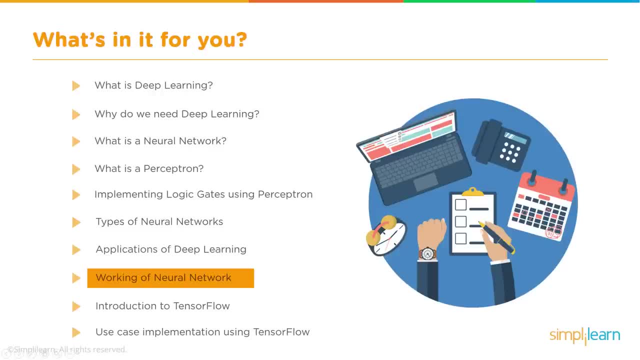 So how do we do the training of neural networks, networks, and at the end, we will end up with a small demo code which will take you through intensive flow. now, in order to implement deep learning code, there are multiple libraries or development environments that are available, and 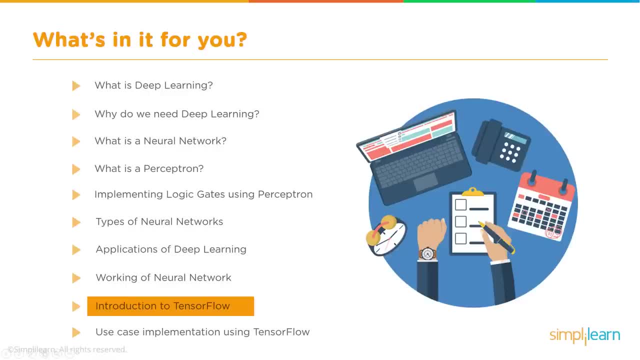 TensorFlow is one of them. so the focus at the end of this would be on how to use TensorFlow to write a piece of code using Python as a programming language, and we will take up an example, which is a very common one, which is like the hello world of deep learning: the handwriting number recognition, which is 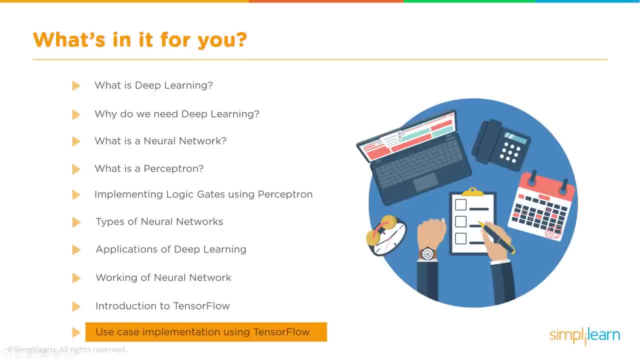 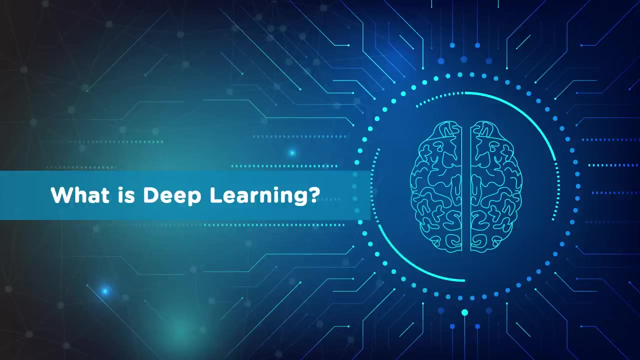 a MNIST, commonly known as MNIST database. so we will take a look at MNIST database and how we can train a neural network to recognize handwritten numbers. so that's what you will see in this particular video. so let's get started. what is deep learning? deep learning is like 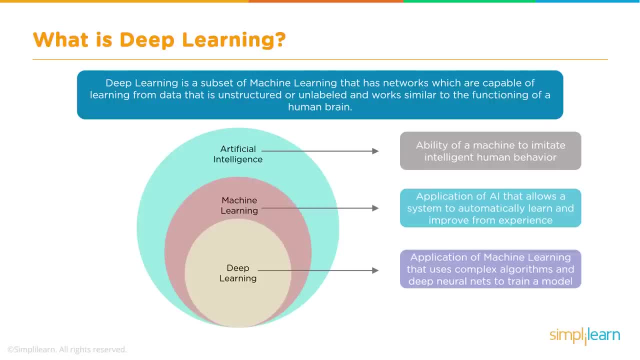 a deep learning is like a subset of what is known as a high-level concept called artificial intelligence. you must be already familiar, must have heard about this term, artificial intelligence. so artificial intelligence is like the high-level concept, if you will. and in order to implement artificial intelligence applications, we 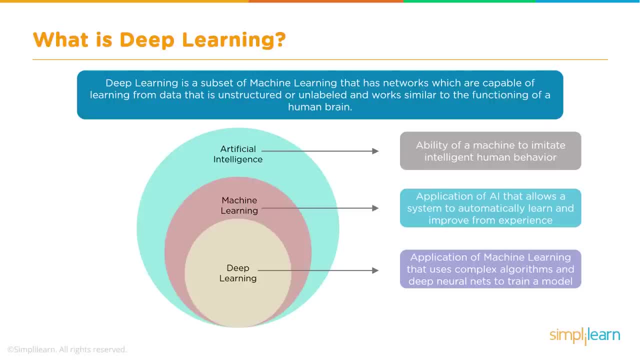 use what is known as machine learning and within machine learning, a subset of machine learning is deep learning. machine learning is a little bit more generic concept and deep learning is one type of machine learning. if you will- and we will see a little later and maybe the following slides a little bit more in: 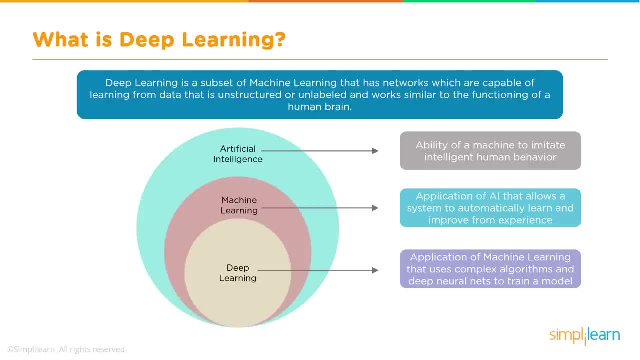 detail how deep learning is different from traditional machine learning. but to start with, we can mention here that deep learning uses. one of the differentiators between deep learning and traditional machine learning is that deep learning uses neural networks, and we will talk about what are neural networks and how we can implement it. 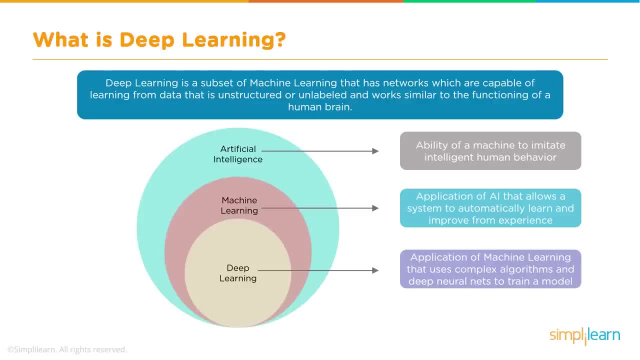 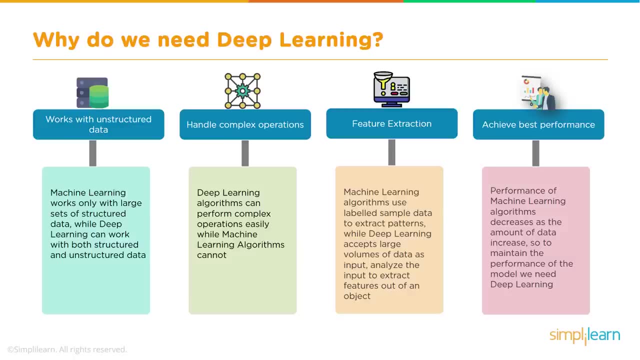 neural networks and so on and so forth as a part of this tutorial. so a little deeper into deep learning. deep learning primarily involves working with complicated, unstructured data. compared to traditional machine learning with where we normally use structured data, in deep learning the data would be primarily images or voice or maybe text file. so and it is large amount of data. 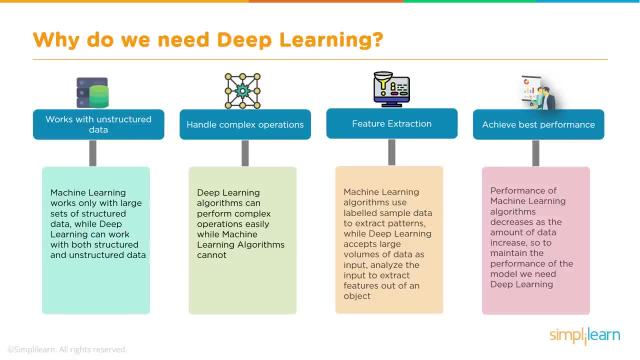 as well, and deep learning can handle complex operations. it involves complex operations and the other difference between traditional machine learning and deep learning is that the feature extraction happens pretty much automatically. in traditional machine learning, feature engineering is done manually. the data scientists- we data scientists- have to do feature. 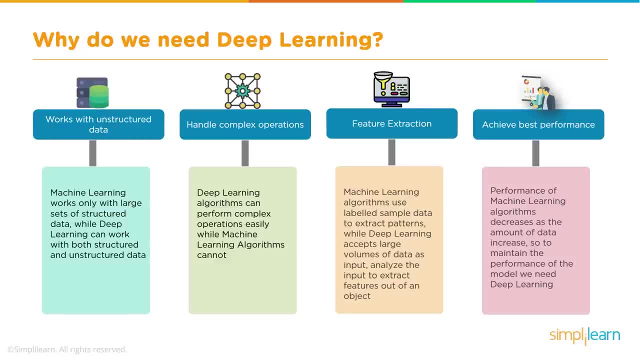 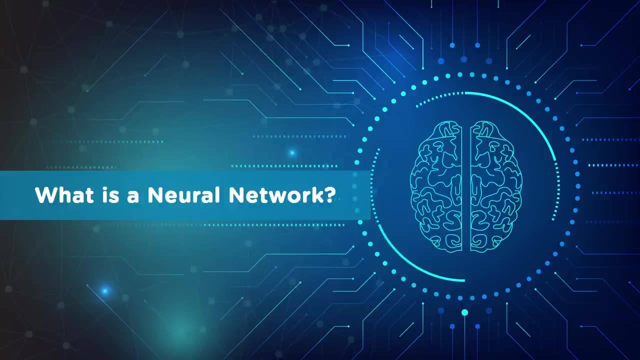 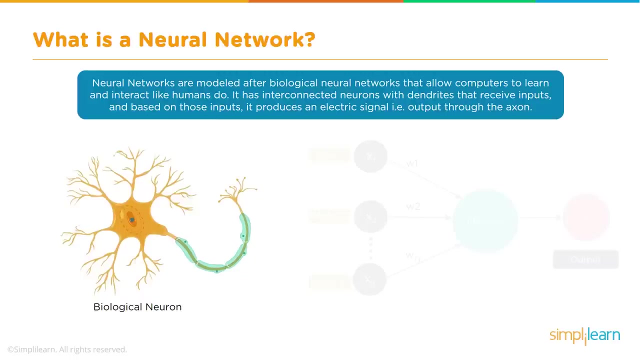 engineering feature extraction, but in deep learning that happens automatically and, of course, deep learning for large amounts of data, complicated, unstructured data. deep learning gives very good performance. now, as I mentioned, one of the secret sources of deep learning is neural networks. let's see what neural networks is. neural networks is based on our biological 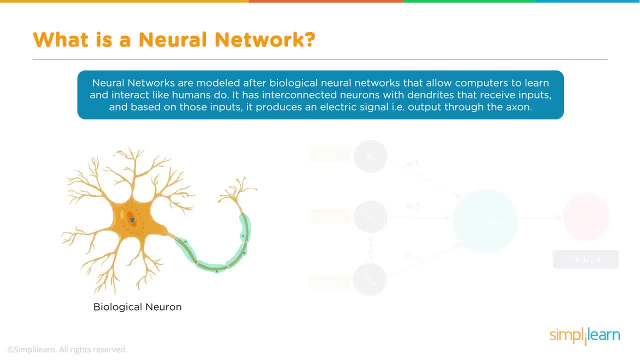 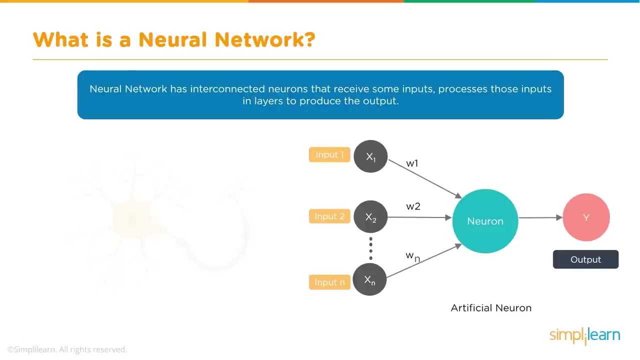 neurons. the whole concept of deep learning and artificial intelligence is based on human brain, and human brain consists of billions of tiny stuff called neurons, and this is how a biological neuron looks, and this is how an artificial neuron looks. so neural networks is like a simulation of our human brain. human brain has billions of biological neurons. 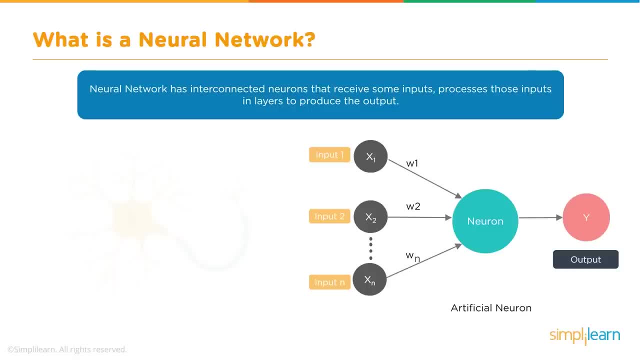 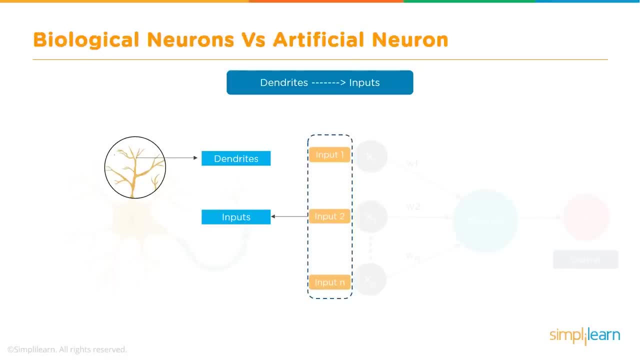 and we are trying to simulate the human brain using artificial neurons. this is how a biological neuron looks: it has dendrites and the corresponding component with an artificial neural network is or an artificial neuron. are the inputs? they receive the inputs through dendrites, and then there is the 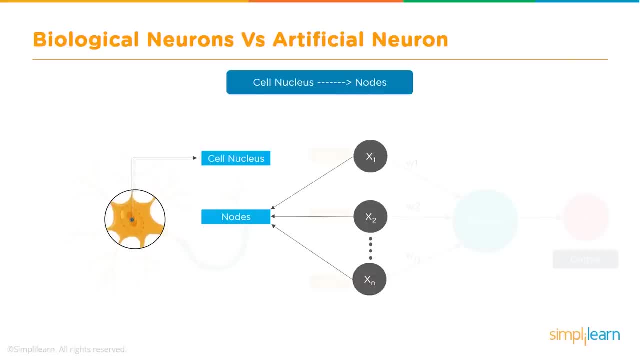 cell nucleus which is basically the processing unit. in a way. so in artificial neuron also, there is a piece which is an equivalent of this cell nucleus and based on the weights and biases we will see what exactly weights and biases are. as we move, the input gets processed and that results in an output, in a biological 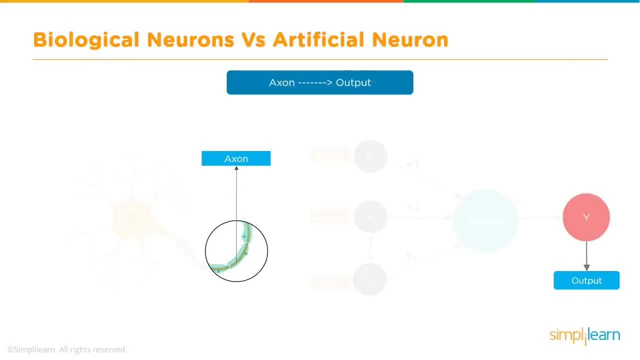 neuron, the output is sent through a synapse and in an artificial neuron there is an equivalent of that in the form of an output, and biological neurons are also interconnected. so there are billions of neurons which are interconnected. in the same way, artificial neurons are also interconnected. so this output of this neuron will be fed as an 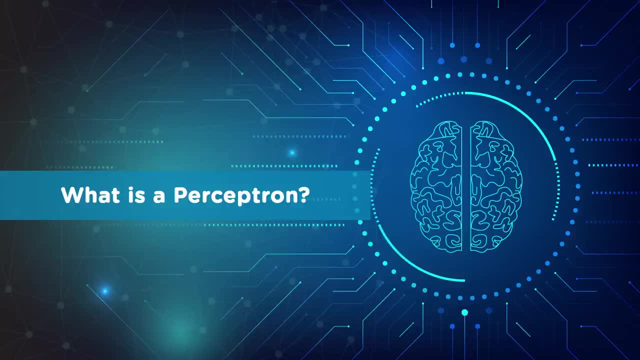 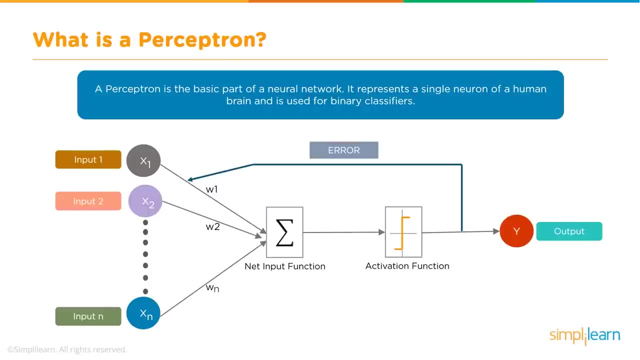 input to another neuron, and so on. now in neural network, one of the very basic units is a perceptron. so what is a perceptron? a perceptron can be considered as one of the fundamental units of neural networks. it can consist at least one neuron, but sometimes it can be more than one neuron. but you can create a. 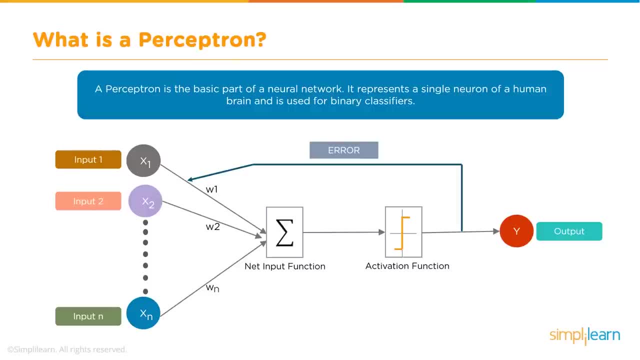 perceptron with a single neuron and it can be used to perform certain functions. it can be used as a basic binary classifier. it can be trained to do some basic binary classification. and this is how a basic perceptron looks like. and this is nothing but a neuron. you have inputs x1, x2, x to xn, and there is a summation function and then there is 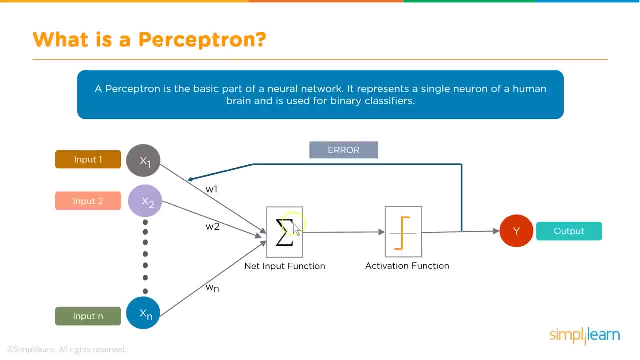 what is known as an activation function and, based on this input, what is known as the weighted sum. the activation function either gets, gives an output like a zero or a one. so we say the neuron is either activated or not. so that's the way it works. so you get the inputs. these inputs are each. 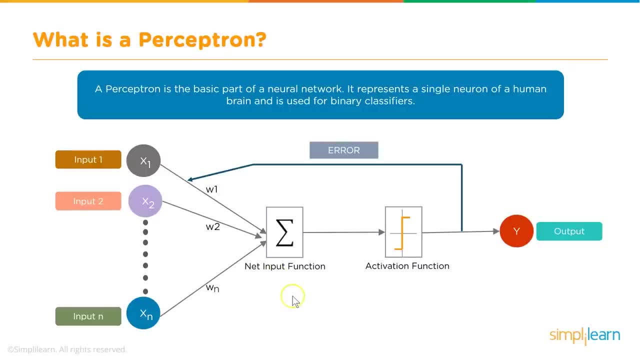 of the inputs are multiplied by a weight and there is a bias that gets added and that whole thing is fed to an activation function and then that results in an output. and if the output is correct it is accepted. it is wrong, if there is an error, then that error is fed back and the neuron then adjusts the weights and biases to. 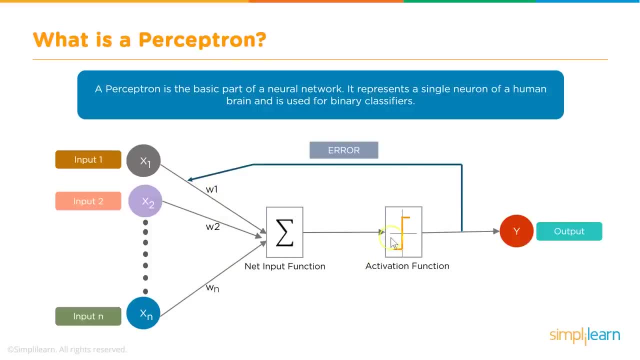 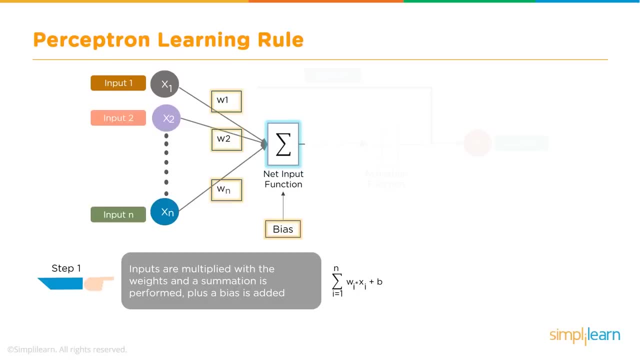 give a new output, and so on and so forth. so that's what is known as the training process of a neuron or a neural network. there's a concept called perceptron learning. so perceptron learning is again one of the very basic learning processes. the way it works is somewhat like this. so you have 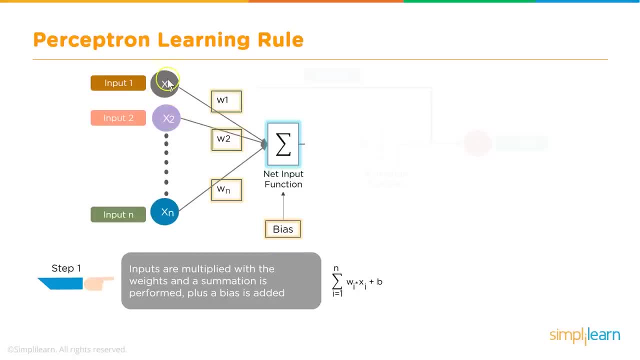 all these inputs, like x1 to xn, and each of these inputs is multiplied by a weight and then that sum. this is the formula or the equation, so that sum wi xi Sigma of that, which is the sum of all these, product of x and w, is added up and then a bias is added to that. the bias is not dependent on. 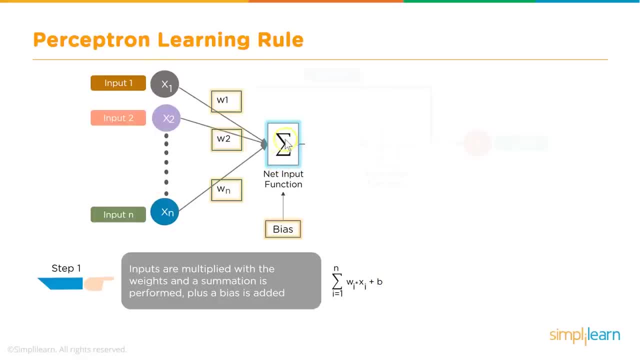 the but or the input values, but the bias is common for one neuron. however, the bias value keeps changing during the training process. once the training is completed, the values of these weights- w1, w2 and so on- and the value of the bias gets fixed. so that is basically the whole training. 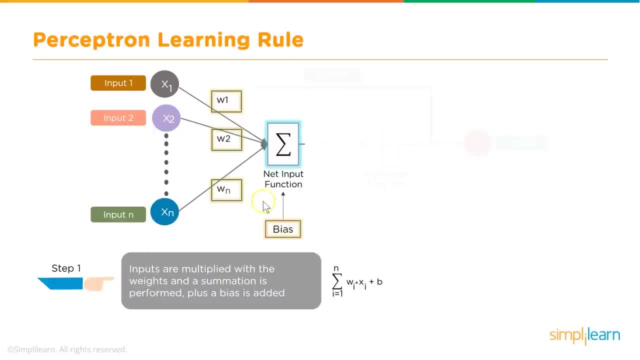 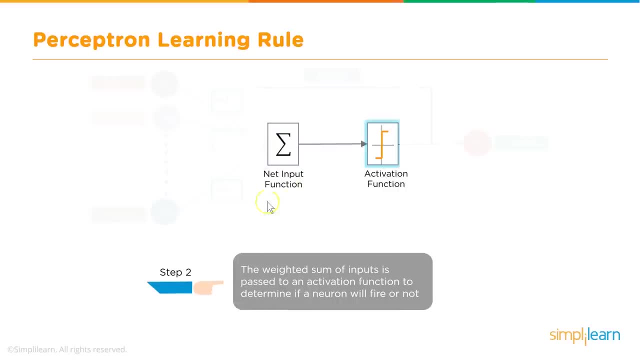 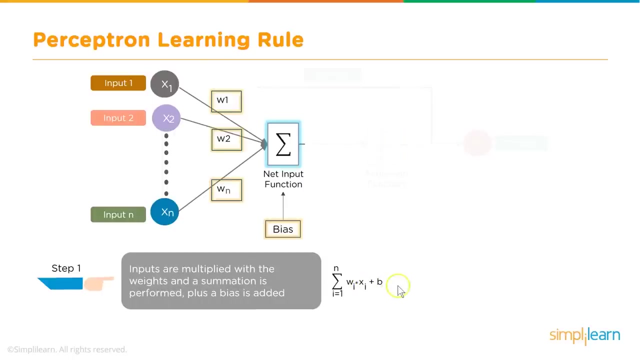 process, and that is what is known as the perceptron training. so the weights and biases keep changing till you get the accurate output, and the summation is of course passed through the activation function. as you see here, this wi xi summation plus b is passed through activation function and then the neuron gets either fired, 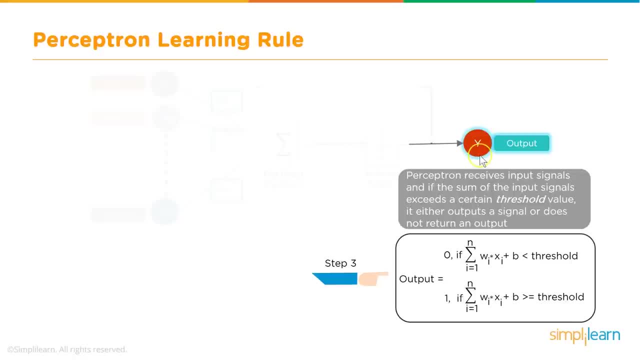 or not, and based on that, there will be an output. that output is compared with the actual or expected value, which is also known as labeled information. this is the process of supervised learning. so the error is already known and that is compared, and thereby we know if there is an error or not, and 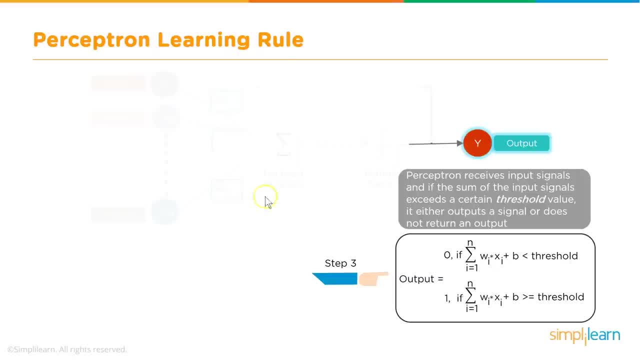 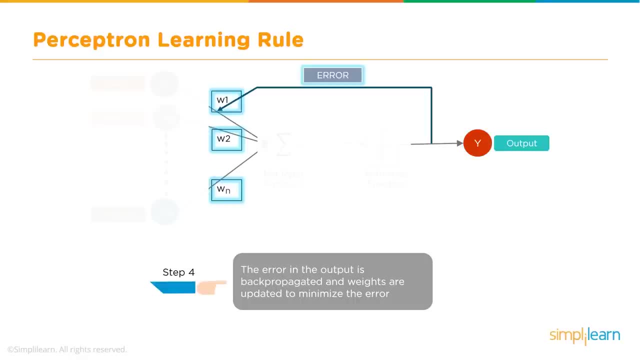 if there is an error, the error is fed back and the weights and biases are updated accordingly. till the error is reduced to the minimum. so this iterative process is known as perceptron learning or perceptron learning rule, and this error needs to be minimized. so, till the error is minimized, this 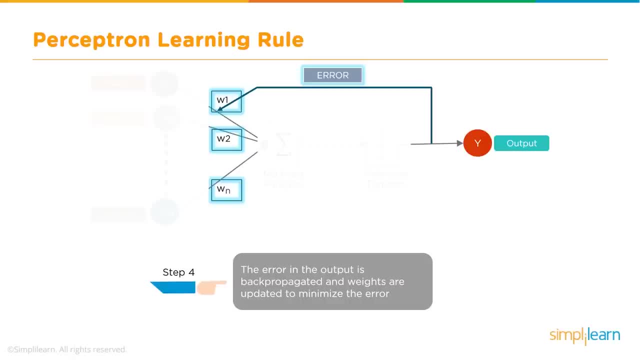 weights and biases keep changing, and that is what is the training process. so the whole idea is to update the weights and the bias of the perceptron till the error is minimized. the error need not be zero, the error may not ever reach zero, but the idea is to keep changing these weights and bias. 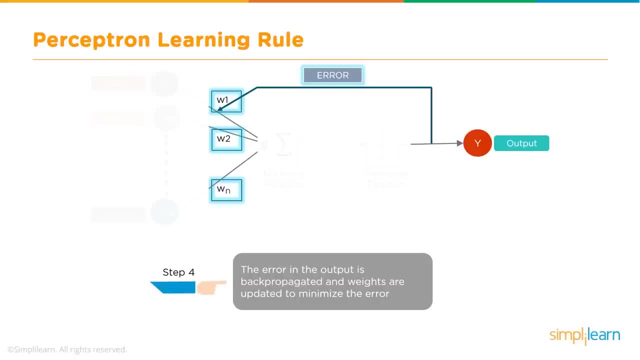 so that the error is minimum, the minimum possible that it can have. so this whole process is an iterative process and this is the iteration continues till. either the error is zero, which is, uh, unlikely situation, or it is the minimum possible within these given conditions. now in 1943, two scientists, Warren 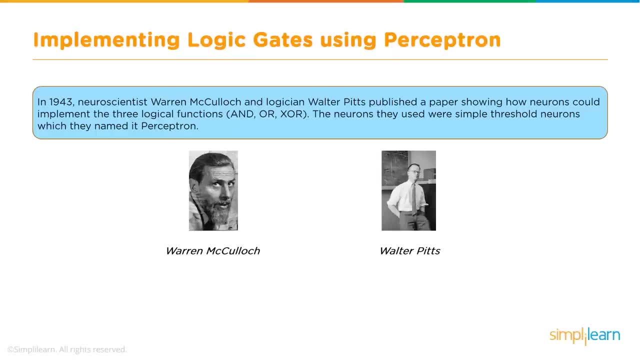 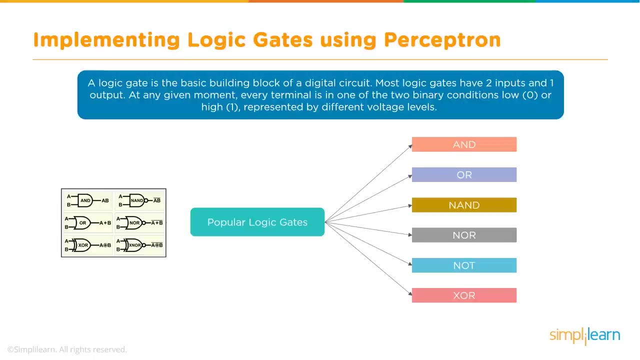 McCulloch and Walter Pitts came up with an experiment where they were able to implement the logical functions like and, or, and nor using neurons, and that was a significant breakthrough in a sense. so they were able to come up with the most common logical gates. they were able to implement some of the most common logical gates, which could take two inputs. 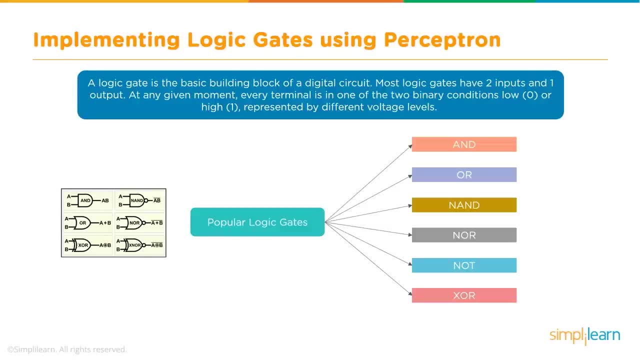 like a and b and then give a corresponding result. so, for example, in case of an and gate, a and B, and then the output is AB. in case of an R gate, it is a plus B, and so on and so forth, and they were able to do this using 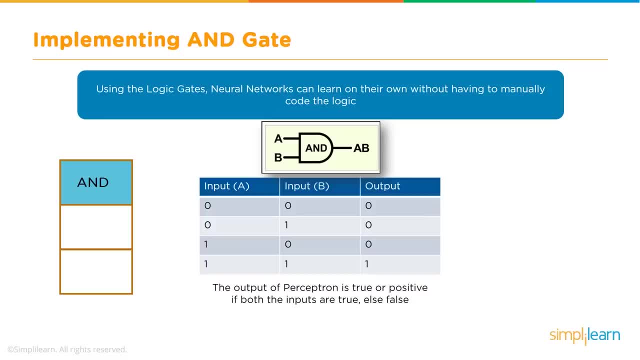 single layer perceptron, now most of these gates. it was possible to use single layer perceptron except for XR and we will see why that is in a little bit. so this is how an and gate works. the inputs a and b, the output should be fired or the neuron should be fired only when both the inputs are one. 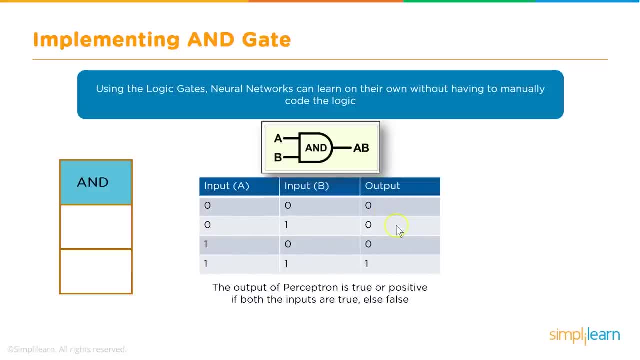 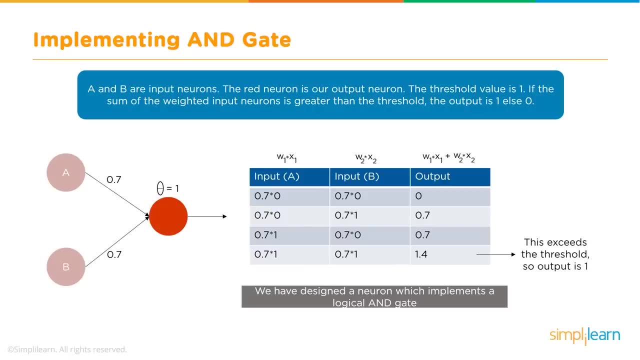 so if you have zero, zero, the output should be zero. for zero one, it is again zero. one zero, again zero, and one one, the output should be one. so how do we implement this with a neuron? so it was found that by changing the values of weights it is possible to achieve this logic. so, for example, if we have equal weights, like 0.7, 0.7, 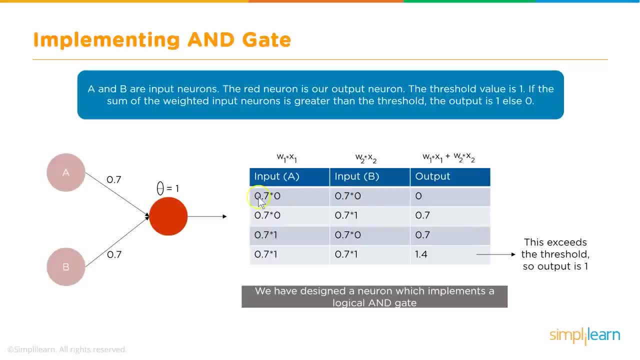 and then if we take the sum of the weighted product, so for example 0.7 into 0 and then 0.7 into 0, will give you 0, and so on and so forth, and in the last case, when both the inputs are one, you 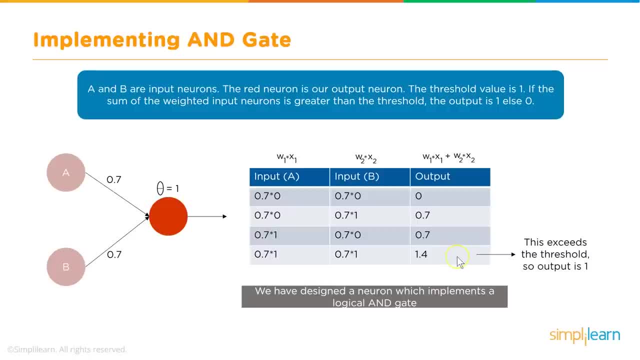 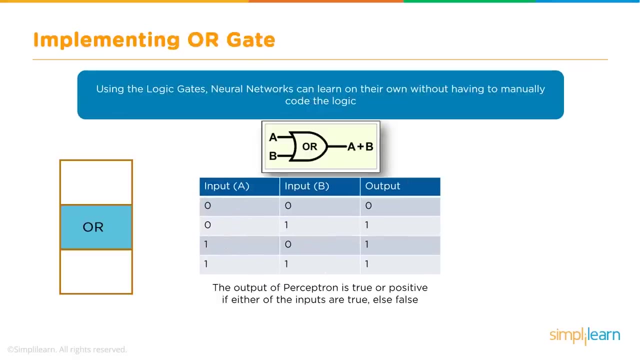 have one, which is the threshold. so only in this case the neuron gets activated and the output is: there is an output. in all the other cases there is no output because the threshold value is one. so this is implementation of an AND gate using a single perceptron or a single neuron. similarly, an 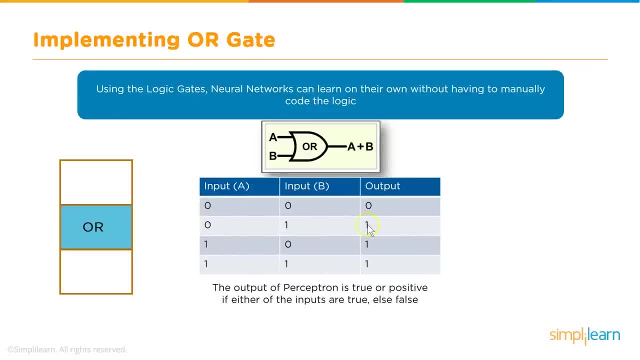 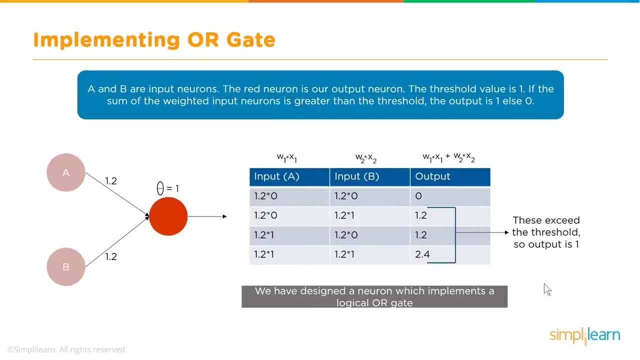 OR gate in order to implement an OR gate. in case of an OR gate, the output will be one if either of these inputs is one, so, for example, zero one will result in one or other. in all the cases it is one, except for zero, zero. so how do we implement this? using a perceptron. once again, if 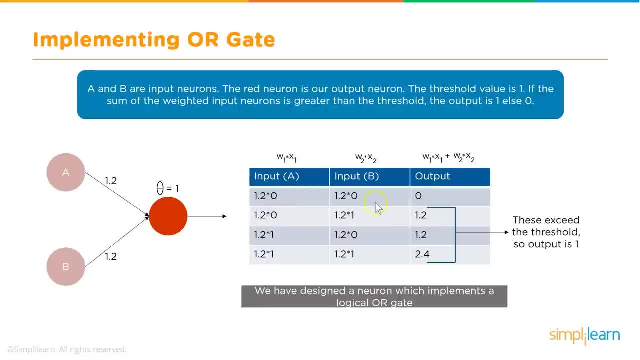 you have a perceptron with weights, for example 1.2. now if you see here, if in the first case, when both are zero, the output is zero, in the second case, when it is zero and one, one point two into zero is zero, and then one point two into one is one, and in the second case, similarly, the output is. 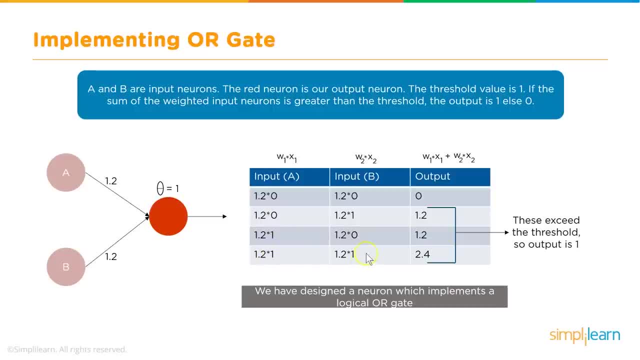 one point two. in this last case, when both the inputs are one, the output is two point four. so during the training process these weights will keep changing and then at one point, where the weights are equal to w1, is equal to 1.2 and w2 is equal to 1.2, the system learns that it gives the correct 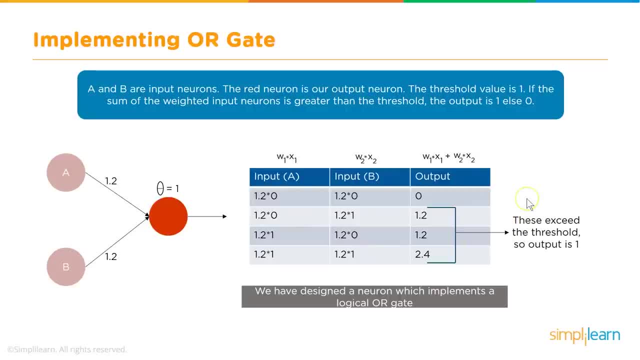 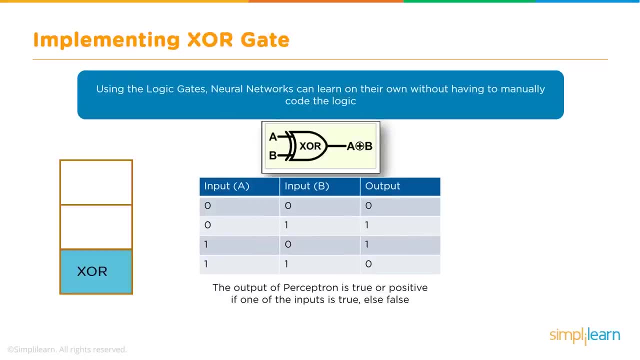 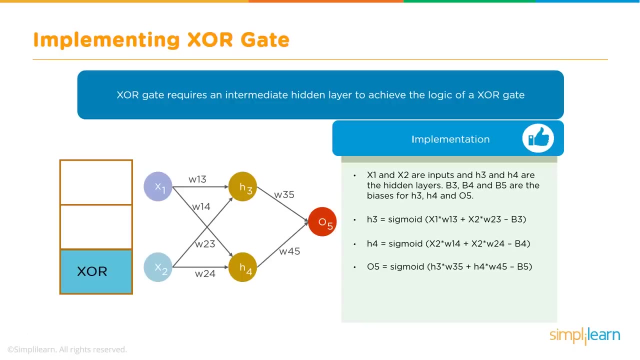 output. so that is implementation of OR gate using a single neuron or a single layer perceptron, now XOR gate. this was one of the challenging ones. they tried to implement an XOR gate with a single level perceptron but it was not possible and therefore in order to implement an XOR. so this was like a roadblock in the progress of a neural network. 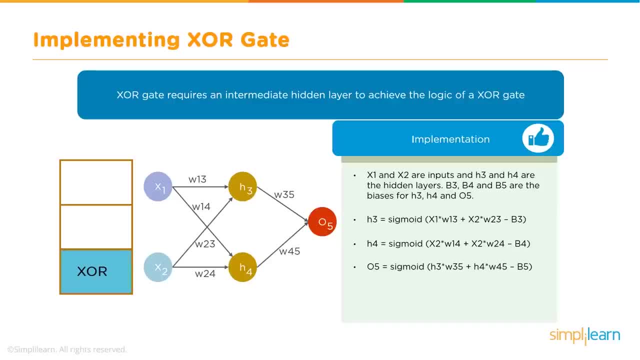 however, subsequently, they realized that this can be implemented. an XOR gate can be implemented using: in these cases, there are two layers instead of a single layer, and this is how you can implement an XOR gate. so you will see that X1 and X2 are the inputs and there is a hidden layer. 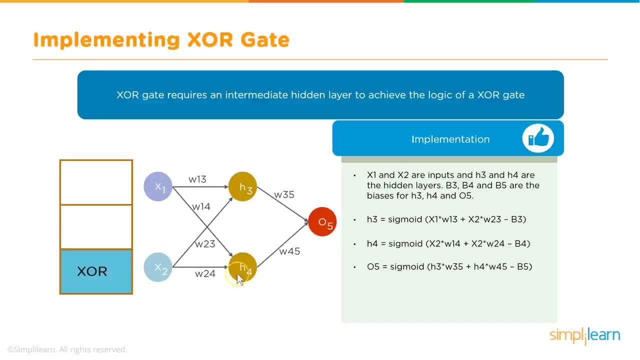 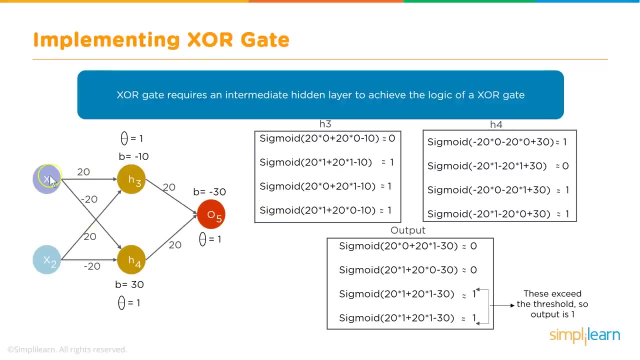 and it is denoted as h3 and h4, and then you take the output of that and feed it to the output at o5 and provide a threshold here. so we will see here that this is the numerical calculation. so the weights are in this case: for x1 it is 20 and minus 20 and once again 20 and minus 20.. 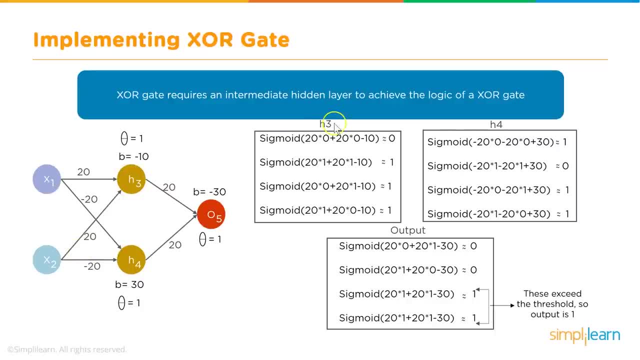 so these inputs are fed into h3 and h4. so you will see here, for h3 the input is 0, 1, 1, 1 and for h4 it is 1 0, 1, 1. and if you now look at the output- final output- where the threshold is taken- 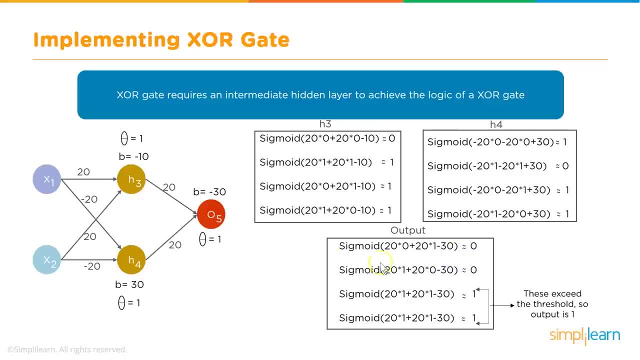 as one. if we use a sigmoid with the threshold one, you will see that in these two cases it is zero and in the last two cases it is one. so this is the implementation of xor. in case of xor, only when one of the inputs is one you will get an output. so that is what we. 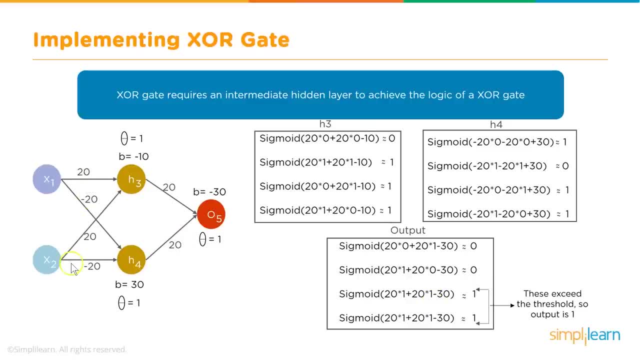 are seeing here, if we have either both the inputs are one or both the inputs are zero, then the output should be zero. so that is what is an exclusive or gate. so it is exclusive because only one of the inputs should be one, and then only you'll get an output of one which is satisfied by 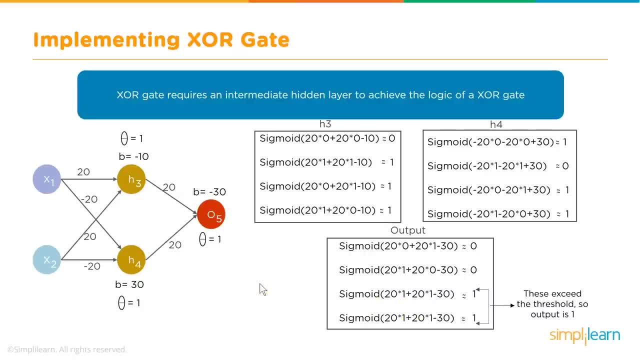 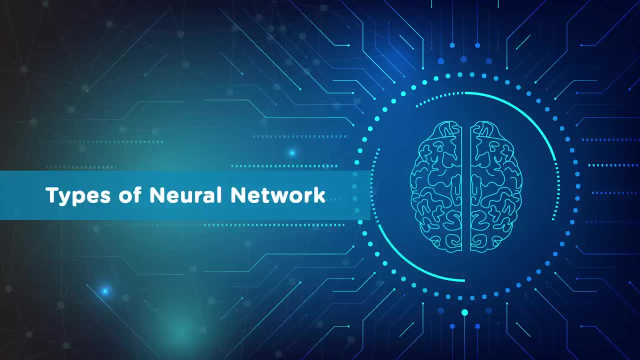 this condition. so this is a special implementation. xor gate is a special implementation of perceptron. now that we got a good idea about perceptron, let's take a look at what is the neural network. so we have seen what is a perceptron. we have seen what is a neuron, so we will see what exactly is a neural network. so 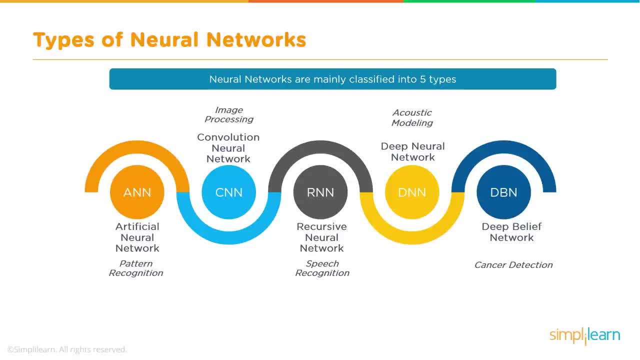 neural network is nothing but a network of these neurons and they are different types of neural networks. there are about five of them. these are artificial neural network, convolutional neural network, then recursive neural network or recurrent neural network, deep neural network and deep belief network. so, and each of these types of neural networks have a special you know they can. 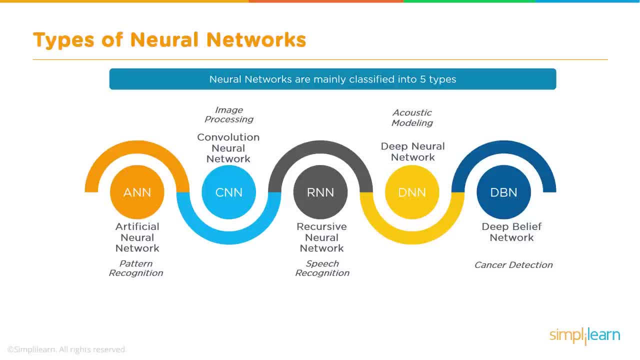 solve special kind of problems. for example, convolutional neural networks are very good at performing image processing and image recognition and so on, whereas rnn are very good for speech recognition and also text analysis and so on. so each type has some special characteristics and they can, they are good at performing certain special kind of 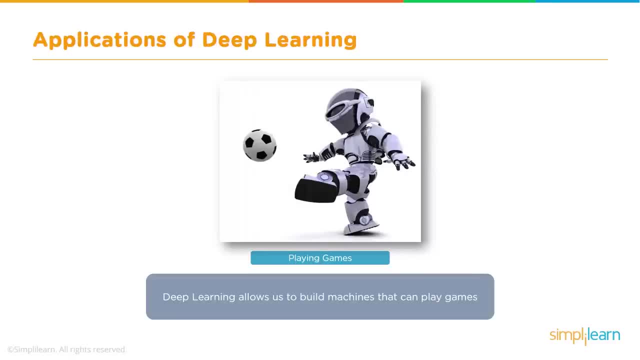 tasks. what are some of the applications of deep learning? deep learning is today used extensively in gaming. you must have heard about alpha go, which is a game created by a startup called deep mind, which got acquired by google, and alpha go is an ai which defeated the human. 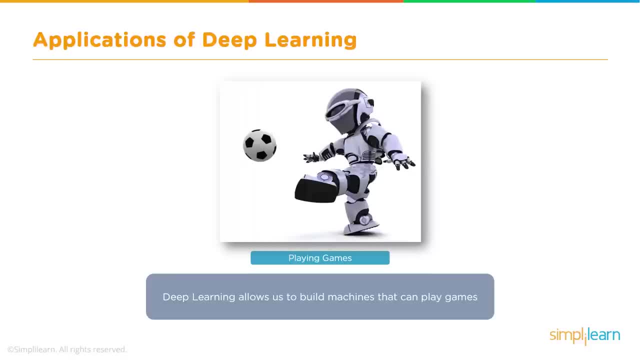 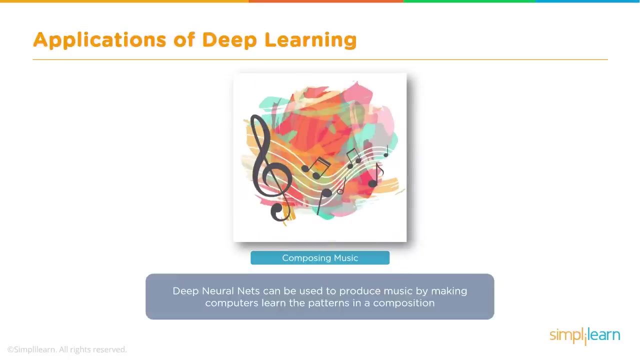 world champion lisa doll in this game of go. so gaming is an area where deep learning is being extensively used and a lot of research happens in the area of gaming as well. in addition to that, nowadays there are neural networks, a special type called generative adversarial networks, which can 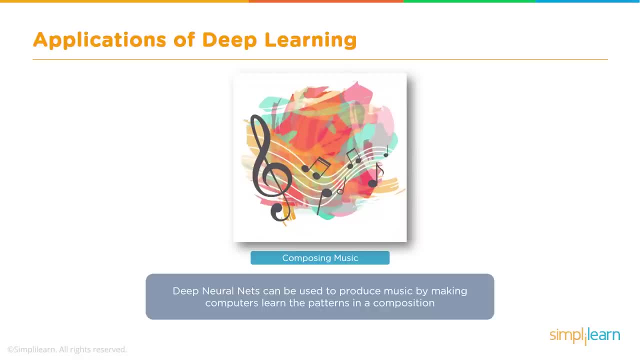 be used for synthesizing either images or music or text and so on, and they can be used to compose music. so the neural network can be trained to compose a certain kind of music. and autonomous cars. you must be familiar with those. you have seen in the movies. you have seen on tv a series of videos. 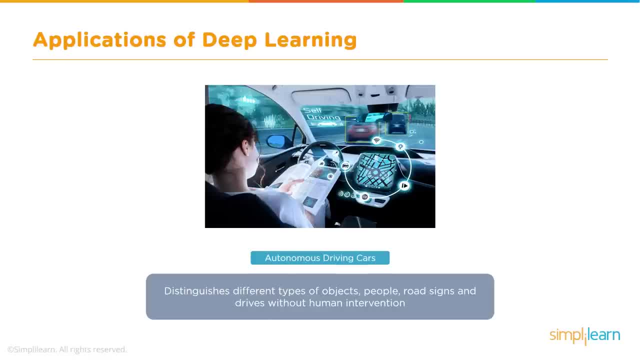 with Google, Google's self-driving car, and today a lot of automotive companies are investing in this space, and deep learning is a core component of this: autonomous cars. the cars are trained to recognize, for example, the road, the lane markings on the road, signals, any objects that are in front, any obstruction, and so 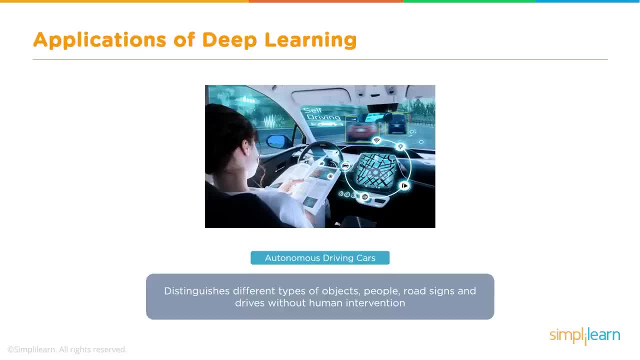 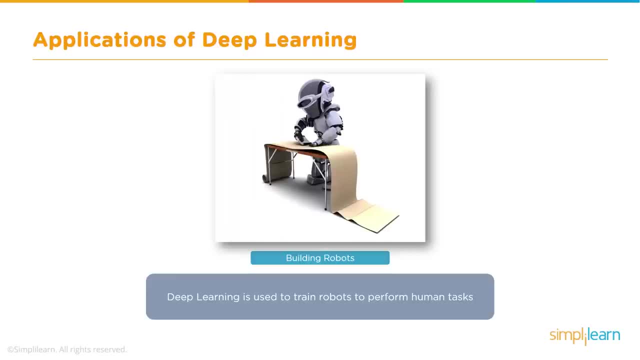 on and so forth. so all this involves deep learning. so that's another major application. and robots: we have seen several robots, including Sophia. you may be familiar with Sophia, who was given a citizenship by Saudi Arabia, and there are several such robots which are very human like and the underlying technology. 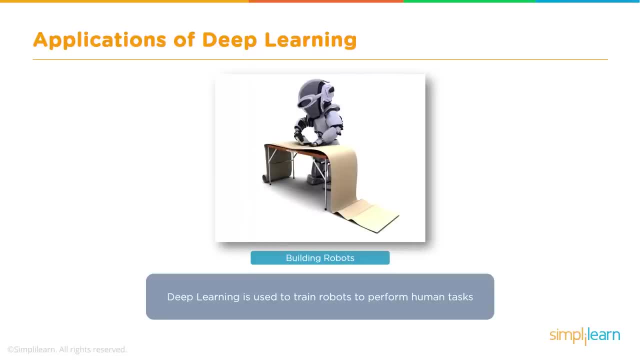 in many of these robots is deep learning. medical diagnostics and health care is another major area where deep learning is being used, and within healthcare diagnostics, diagnostics- again- there are multiple areas where deep learning and image recognition, image processing, can be used, for example, for cancer detection. as you may be aware, if cancer is 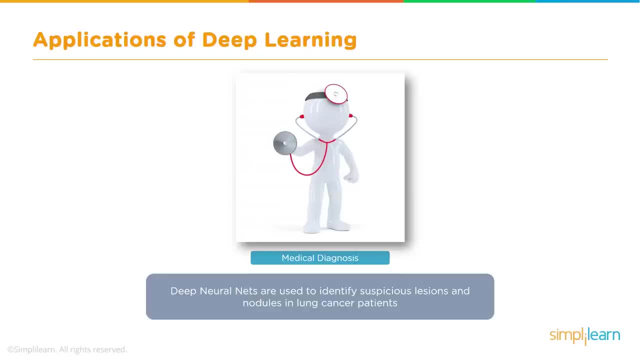 detected early on, it can be cured, and one of the challenges is in the availability of specialists who can diagnose cancer using these diagnostic images and various scans, and and so on and so forth. so the idea is to train neural network to perform some of these activities so that the 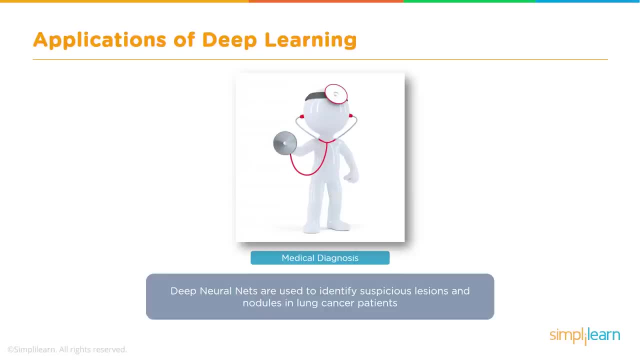 load on the cancer specialist doctors or oncologist comes down, and there is a lot of research happening here and there are already quite a few applications that are claimed to be performing better than human beings in this space can be lung cancer, it could be breast cancer and so on and so forth. so 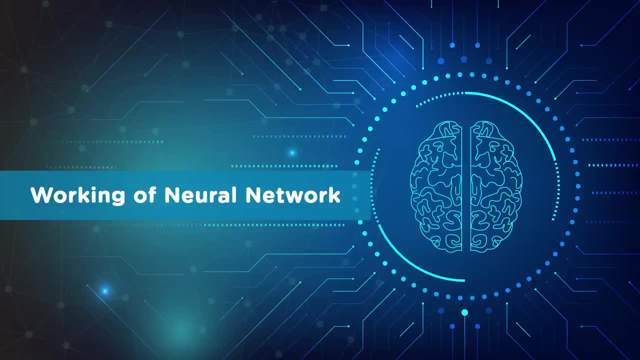 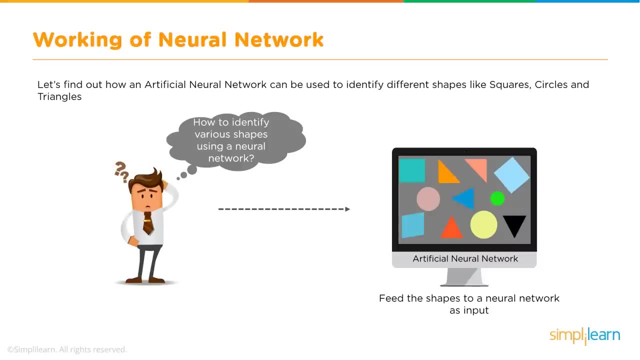 health care is a major area where deep learning is being applied. let's take a look at the inner working of a neural network. so how does an artificial neural network, let's say, identify? can we train a neural network to identify the shapes like squares and circles and triangles when these images are fed? so this is how it works. 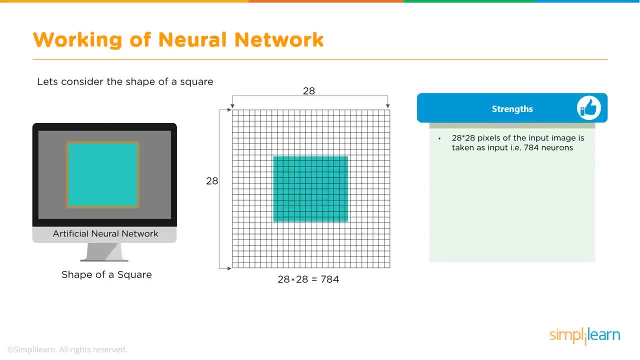 any image is nothing, but it is a digital information of the pixels. so in this particular case, let's say: this is an image of 28 by 28 pixel, and this is an image of a square. there is a certain way in which the pixels are lit up, and so these pixels have a certain value. 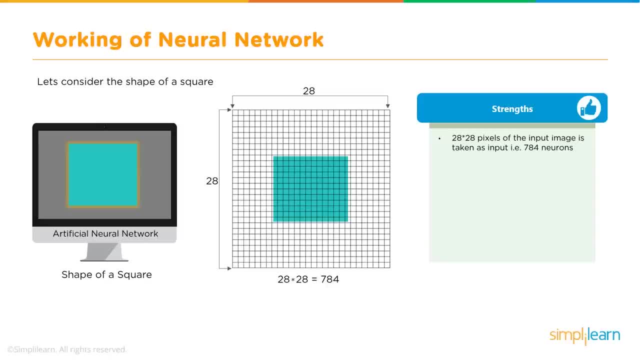 maybe from 0 to 256, and 0 indicates that it is black or it is dark and 256 indicates it is completely, it is white or lit up. so that is like an indication or a measure of the how the pixel are lit up. and so this is an image is, let's say, consisting of information of 784 pixels. 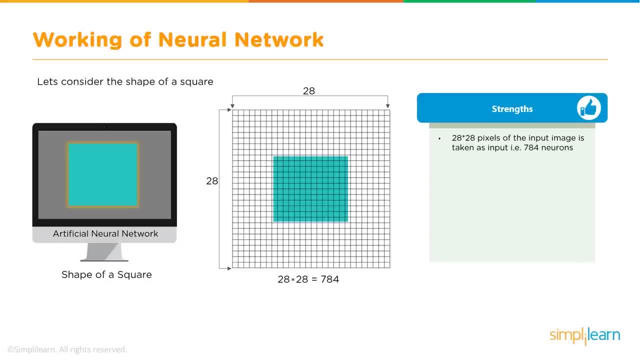 so all the information, what is inside this image, can be kind of compressed into this 784 pixels. the way each of these pixels is lit up provides information about what exactly is the image. so we can train neural networks to use that information and identify the images. so let's take a look how this works. so each neuron the value if it is close to one. that 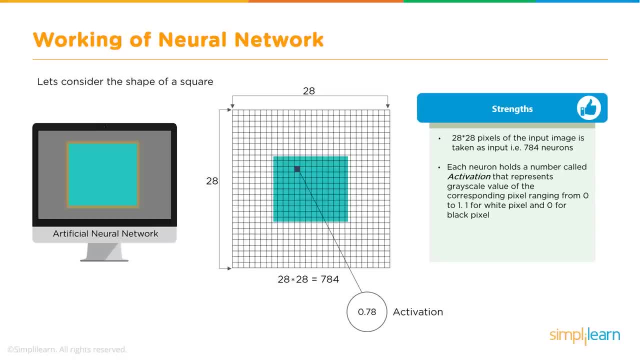 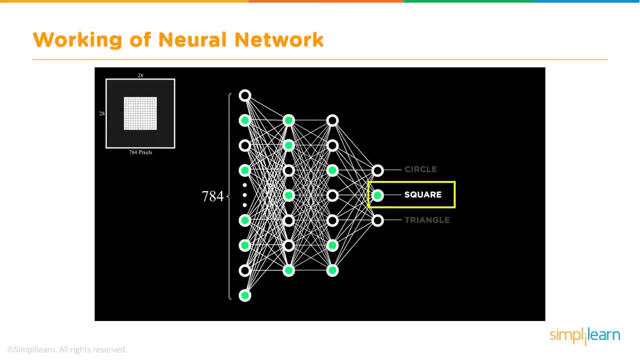 means it is white, whereas if it is close to zero, that means it is black. now, this is a an animation of how this whole thing works. so these pixels. one of the ways of doing it is we can flatten this image and take this complete 784 pixels and 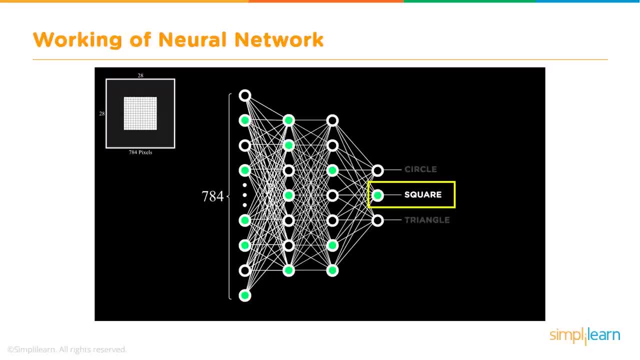 that as input to our neural network. the neural network can consist of probably several layers. there can be a few hidden layers and then there is an input layer and an output layer. now the input layer. take the 784 pixels as input, the values of each of these pixels and 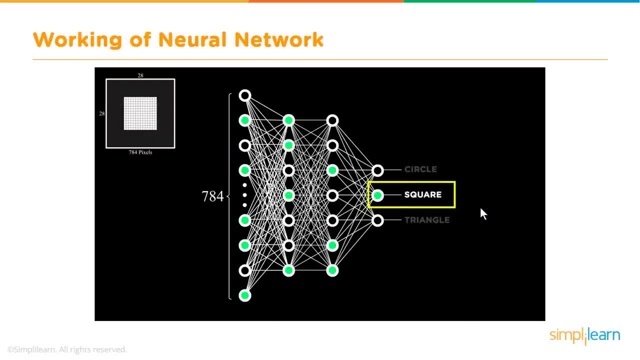 then you get an output which can be of three types or three classes. one can be a square, a circle or a triangle. now, during the training process there will be initially, obviously, you feed this image and it will probably say it's a circle or it will say it's a triangle. so, as a part of the 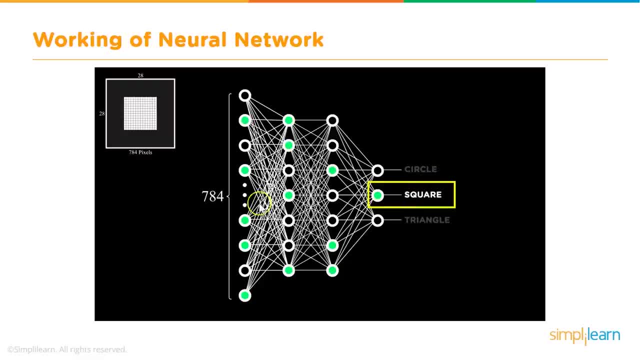 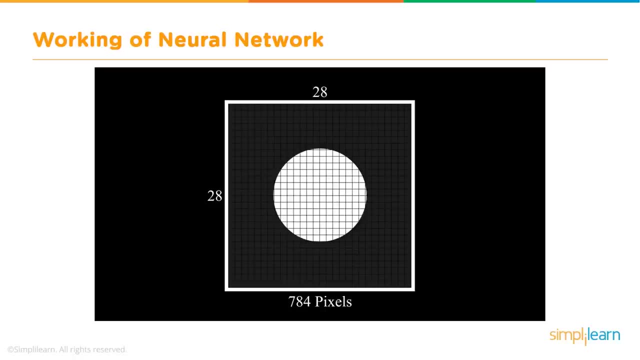 training process. we then send that error back and the weights and the biases of these neurons are adjusted till it correctly identifies that this is a square. that is the whole training mechanism that happens out here. now let's take a look at a circle. same way. so you feed these. 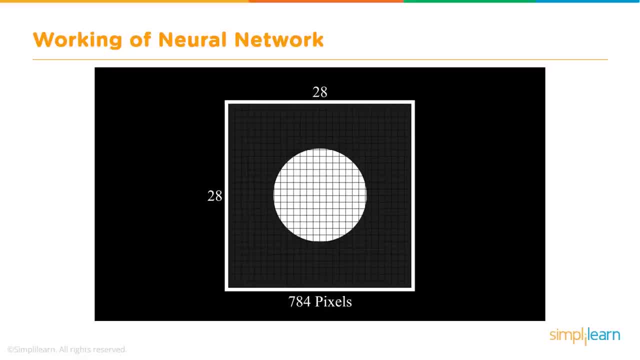 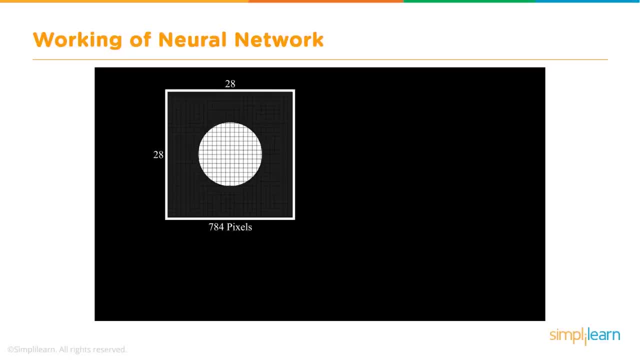 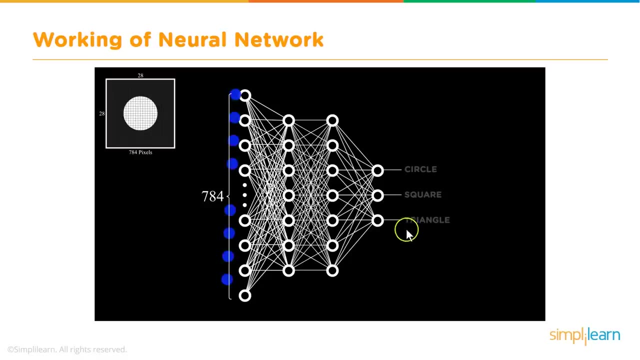 84 pixels. there is a certain pattern in which the pixels are lit up and the neural network is trained to identify that pattern and during the training process, once again, it would probably initially identify it incorrectly, saying this is a square or a triangle, and then that error. 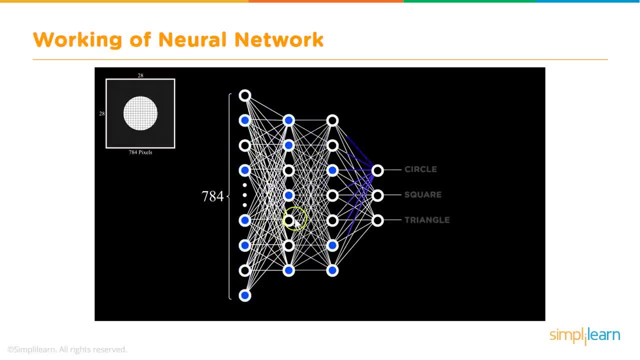 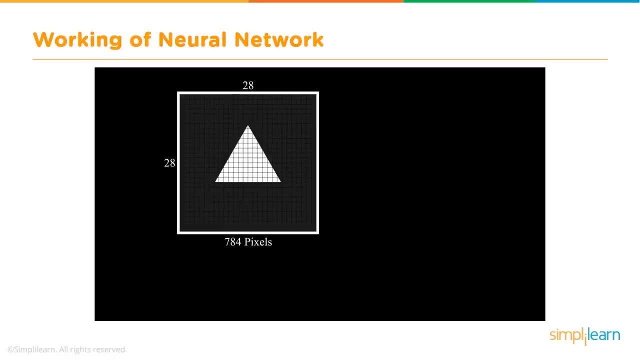 is fed back and the weights and biases are adjusted, finally till it finally gets the image correct. so that is the training process. so now we will take a look at same way: a triangle. so now if you feed another image which is consisting of triangles. so this is the training process. now we 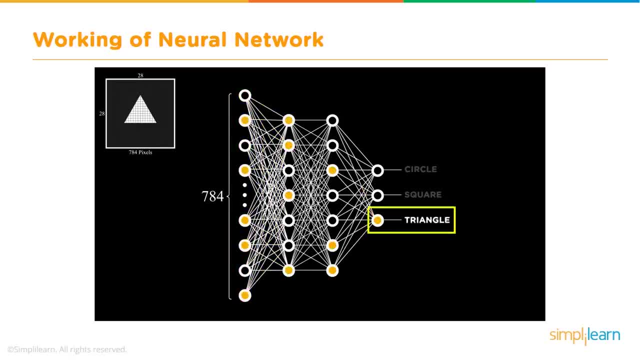 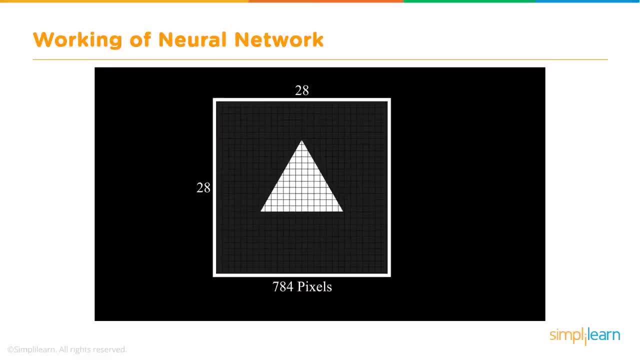 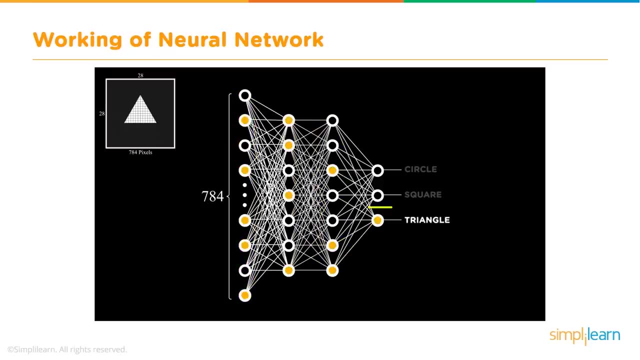 have trained our neural network to classify these images into a triangle or a circle and a square. so now this neural network can identify these three types of objects. now, if you feed another image and it will be able to identify whether it's a square or a triangle or a circle. now what is important to 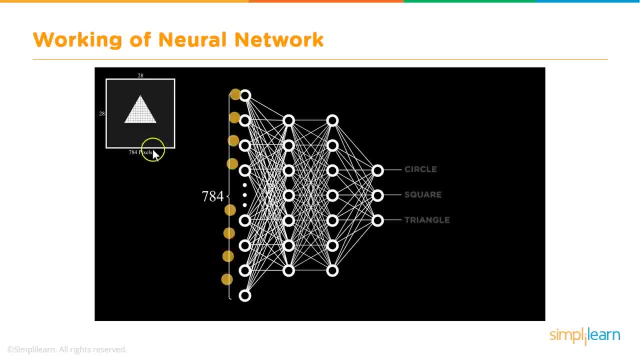 be observed is that when you feed a new image, it is not necessary that the image, or the the triangle, is exactly in this position. now the neural network actually identifies the patterns. so even if the triangle is, let's say, positioned here not exactly in the middle, but maybe at the corner or in the 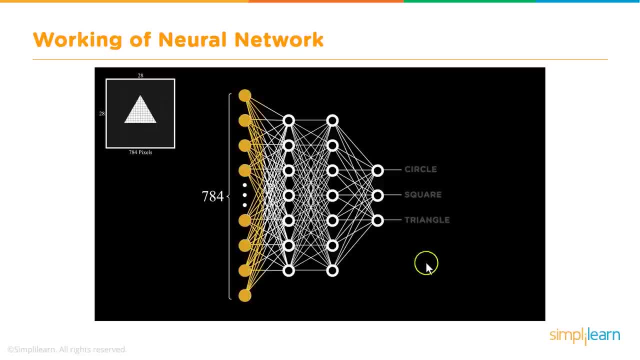 side, it will be able to identify whether it's a square or a triangle or a circle. now what is important to know is that if the new image is not necessarily a square, then it will still identify that it is a triangle, and that is the whole idea behind pattern recognition. so how does this training process? 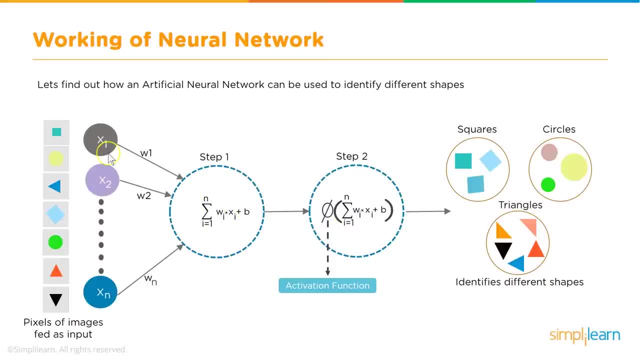 work. this is a quick view of how the training process works. so we have seen that a neuron consists of inputs, it receives inputs and then there is a weighted sum which is nothing but this xi wi summation of that plus the bias, and this is then fed to the activation function and that in 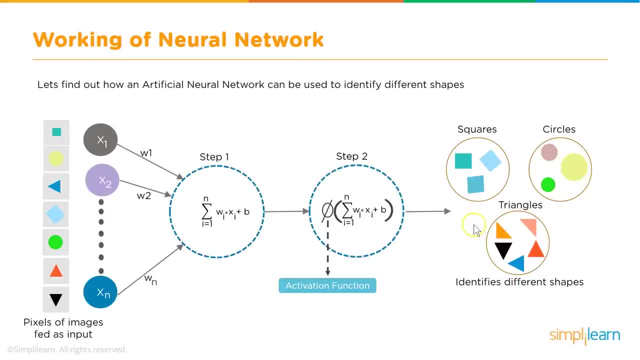 gives us a output now during the training process. initially, obviously, when you feed these images, when you send maybe a square, it will identify it as a triangle, and when you maybe feed a triangle, it will identify as a square, and so on, so that error information is fed back. and initially these: 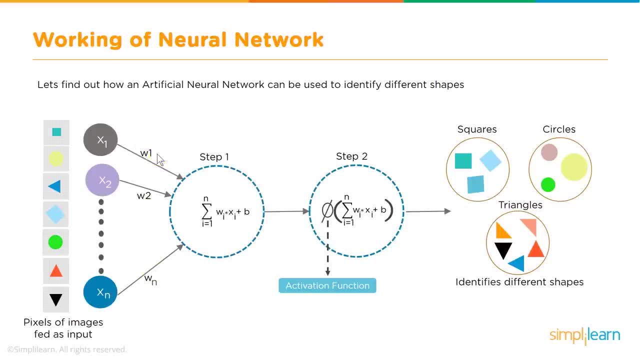 weights can be random. maybe all of them have zero values and then it will slowly keep changing. so the, as a part of the training process, the values of these weights- w1, w2, up to wn- keep changing in such a way that towards the end of the training process, it should be able to identify these images. 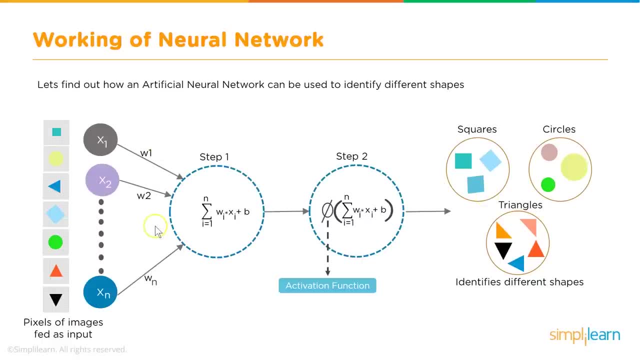 correctly. so till then, the weights are adjusted, and that is known as the training process. so, and these weights are numeric values, it could be 0.5, 0.25, 0.35 and so on, it could be positive or it could be negative, and the value that is coming here is the pixel value, as we have. 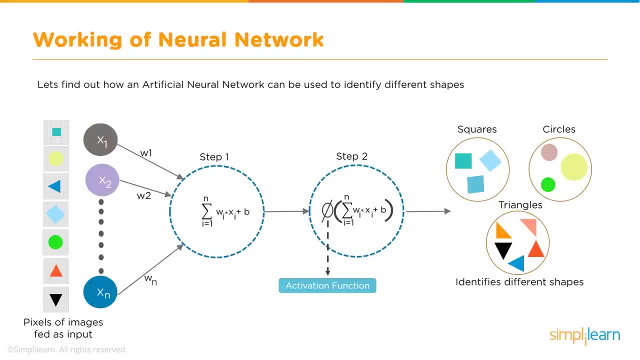 seen in the training process. so, as a part of the training process, the values of these weights are seen. it can be anything between 0 to 1. you can scale it between 0 to 1 or 0 to 256, whichever way, 0 being black and 256 being white, and then all the other colors in between. so that is the input. so 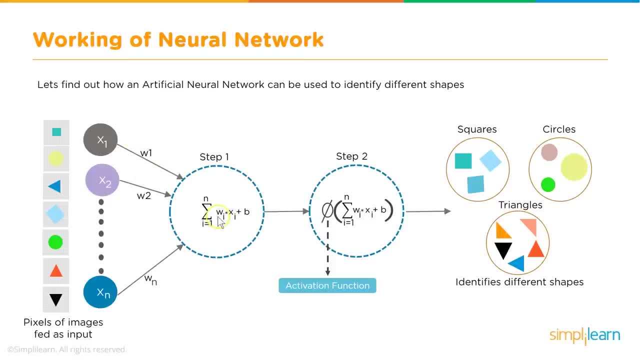 these are numerical values. this multiplication, or the product wi xi, is a numerical value and the bias is also a numerical value. we need to keep in mind that the bias is fixed for a neuron. it doesn't change with the inputs, whereas the weights are one per input. so that is one important. 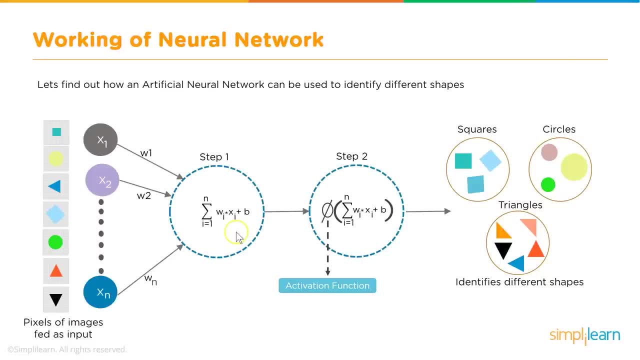 point to be noted. so, but the bias also keeps changing. initially it will again have a random value, but as a part of the training process, the weights, the values of the weights w1, w2, wn and the value of b will change and ultimately, once the training process is complete, these values are fixed. 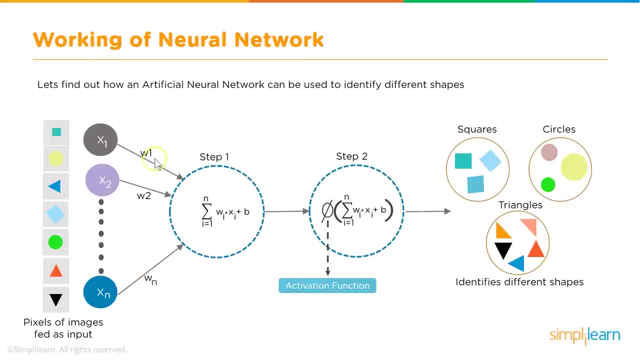 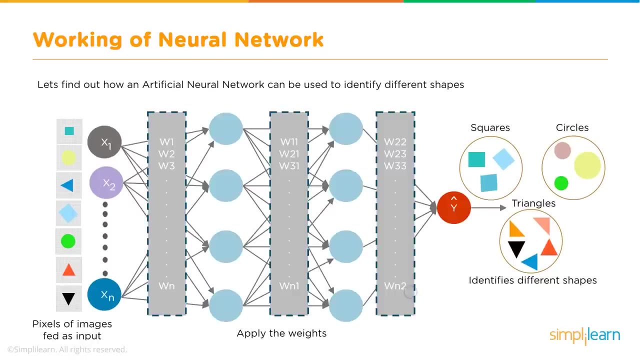 for this particular neuron: w1, w2 up to wn and plus the value of the b is also fixed for this particular neuron, and in this way there will be multiple neurons and each there may be multiple levels of neurons here, and that's the way the training process works. so this is another example of multi-layer. so there are two hidden. 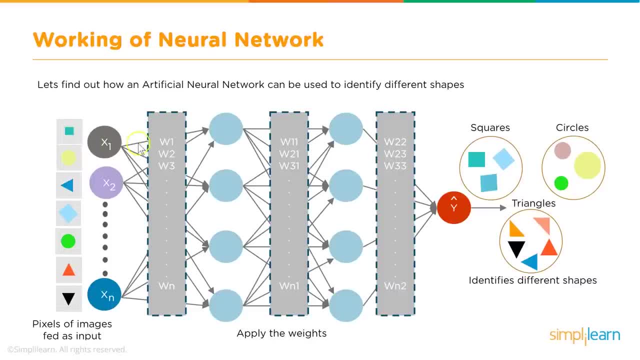 layers in between and then you have the input layer values coming from the input layer, then it goes through multiple layers, hidden layers, and then there is an output layer and, as you can see, there are weights and biases for each of these neurons in each layer and all of. 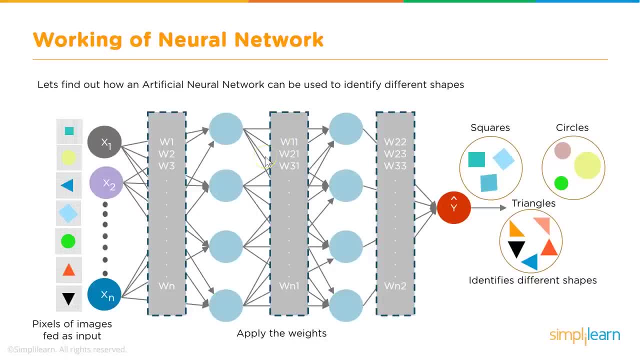 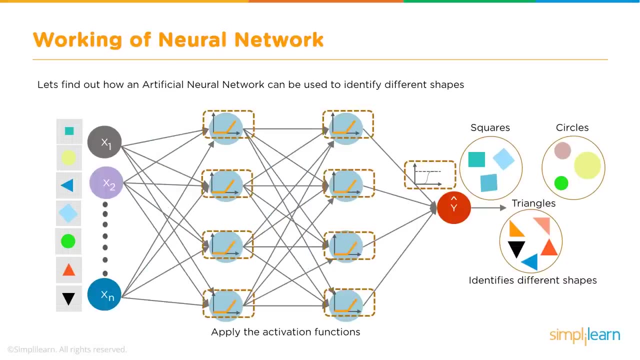 them gets keeps changing during the training process and at the end of the training process. all these weights have a certain value, and that is a trained model, and those values will be fixed once the training is completed. all right, then there is something known as activation function. neural networks consists of. one of the components in neural networks is activation function, and 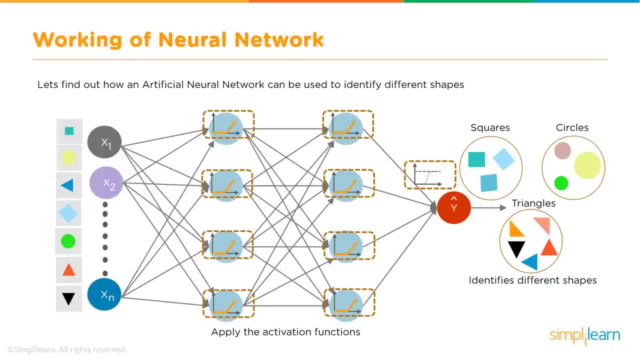 every neuron has an activation function and there are different types of activation functions that are used in the activation function. it could be a relu, it could be sigmoid, and so on and so forth, and the activation function is what decides whether a neuron should be fired or not. so 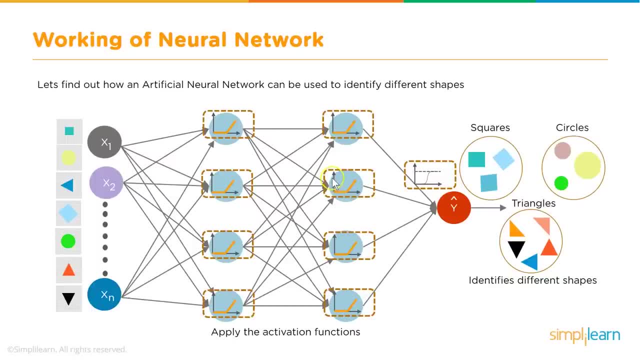 whether the output should be 0 or 1 is decided by the activation function, and the activation function in turn takes the input, which is the weighted sum- remember we talked about wi xi plus b. that weighted sum is fed as a input to the activation function, and then the output can be. 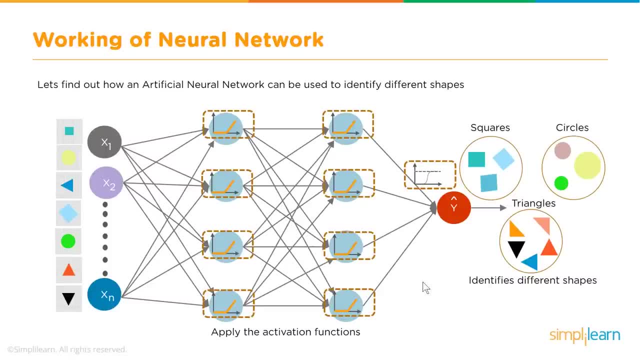 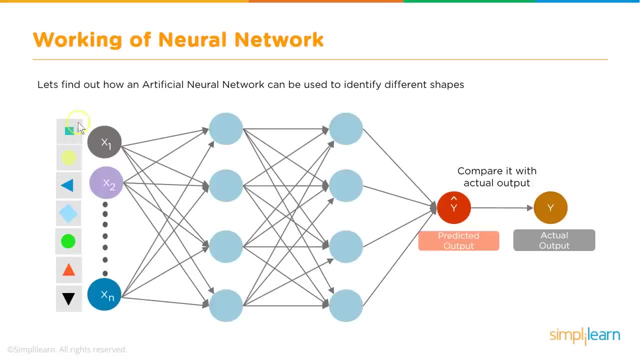 either a 0 or a 1.. So there are some types of activation functions which are covered in an earlier video you might want to watch. all right, so as a part of the training process, we feed the inputs- the labeled data or the training data- and then it gives an output which is the predicted output by 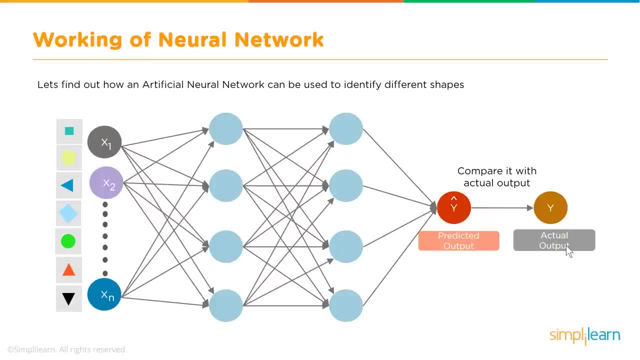 the network which we indicate as y hat, and then there is a labeled data, because we, for supervised learning, we already know what should be the output. so that is the actual output. and in the initial process, Before the training is complete, Obviously there will be error. So that is measured by what is known as a cost function. So the difference 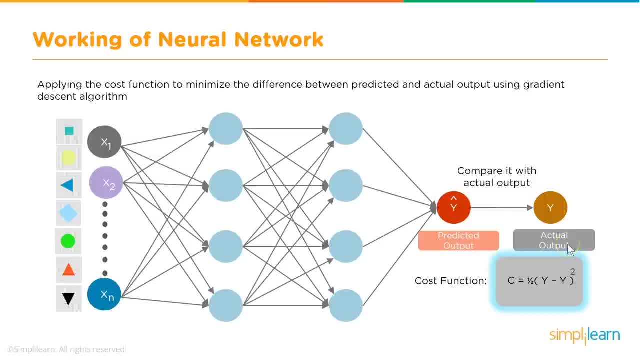 between the predicted output and the actual output is the error, And the cost function can be defined in different ways. There are different types of cost functions, So in this case it is like the average of the squares of the error. So, and then all the errors are added, which can: 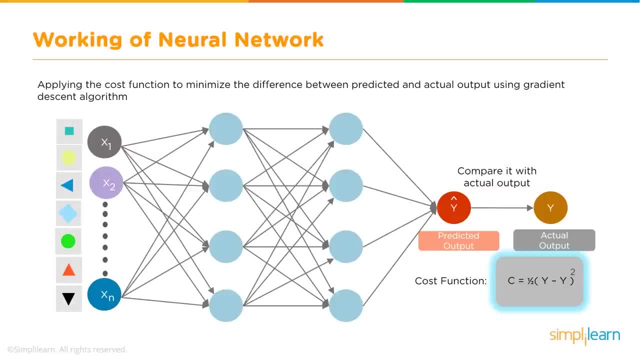 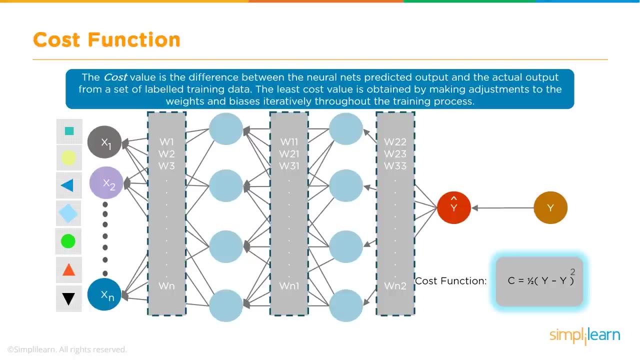 sometimes be called as sum of squares, sum of square errors or SSE, And that is then fed as a feedback in what is known as backward propagation or back propagation, And that helps in the network adjusting the weights and biases, And so the weights and biases get updated till this value. 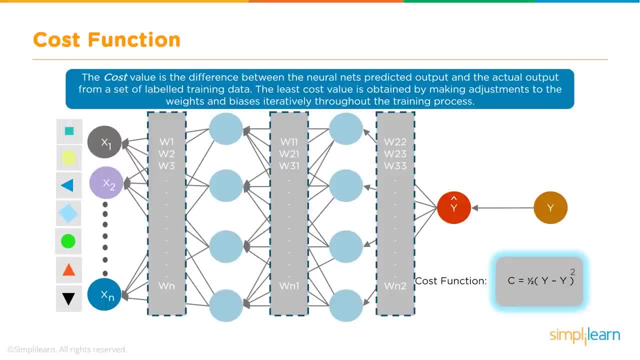 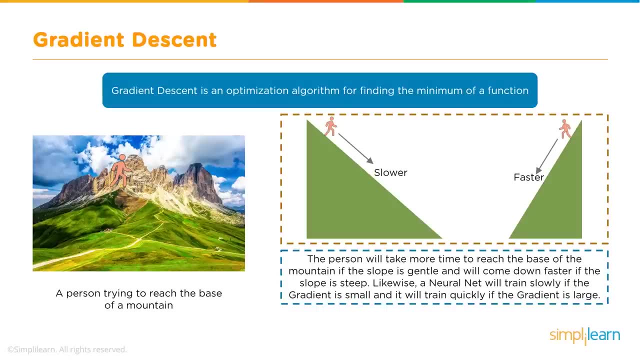 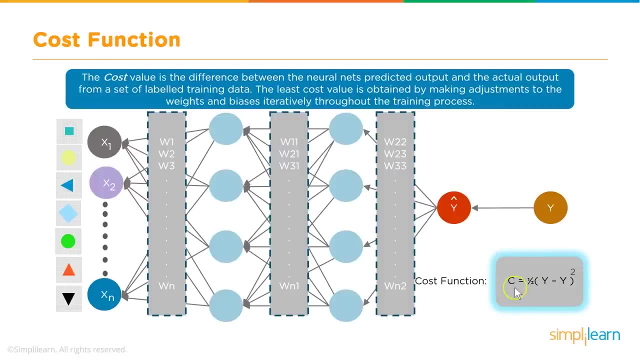 the error value or the cost function is minimum. Now there is a optimization technique which is used here, called gradient descent optimization, And this algorithm works in a way that the error, which is the cost function, needs to be minimized. So there's a lot of mathematics that goes behind this. For example, 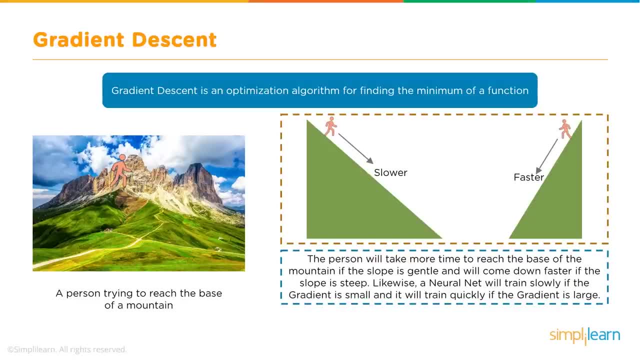 they find the local minima on the global minima, using differentiation and so on and so forth. But the idea is this: So, as a training process, as a part of training, the whole idea is to bring down the error, which is like, let's say, this is the function, the cost function. at certain levels it is very high the cost value. 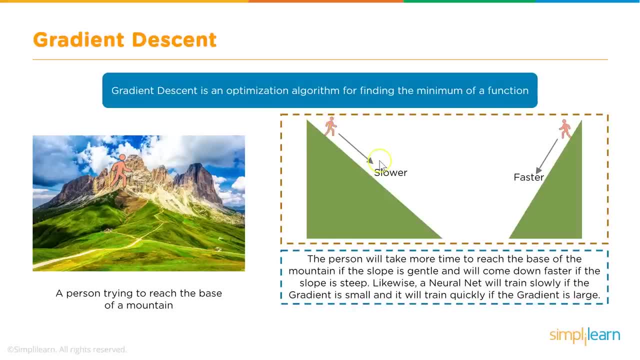 of the cost function. the output of the cost function is very high, So the weights have to be adjusted in such a way- and also the bias, of course- that the cost function is minimized. So there is this optimization technique called gradient descent that is used, And this is known as the learning rate. Now, gradient descent you need to. 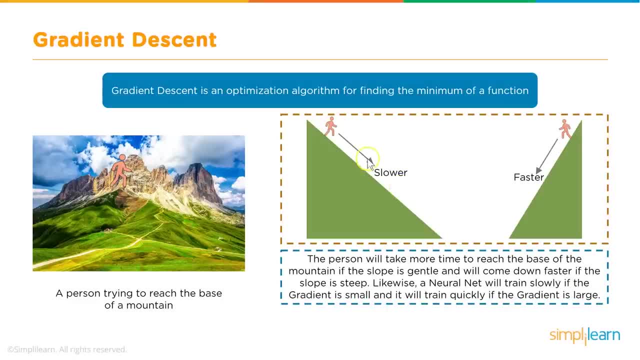 specify what should be the learning rate. and the learning rate should be optimal, because if you have a very high learning rate, then the optimization will not converge because at some point it will cross over to the side. on the other hand, if you have very low learning rate, then it might take forever to convert. so you 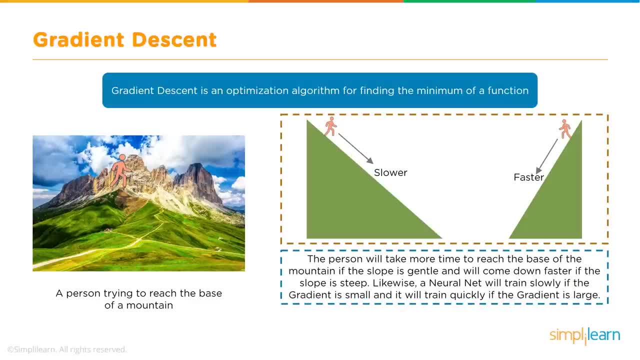 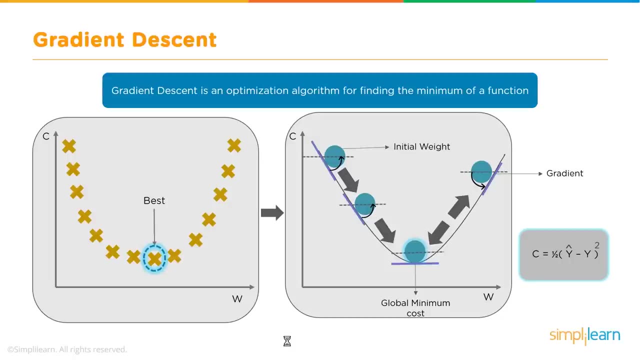 need to come up with the optimum value of the learning rate, and once that is done, using the gradient descent optimization, the error function is reduced and that's like the end of the training process. alright, so this is another view of gradient descent. so this is how it looks. this is your cost. 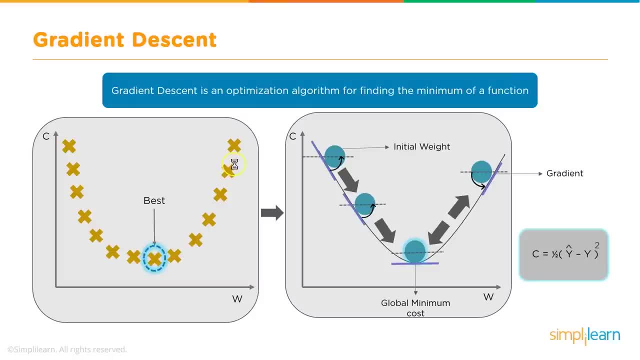 function, the output of the cost function, and that has to be minimized using gradient descent algorithm and these are like the parameters, and weight could be one of them. so initially we start with certain random values, so cost will be high, and then the weights keep changing and in such a way that the cost function needs to come down and at some 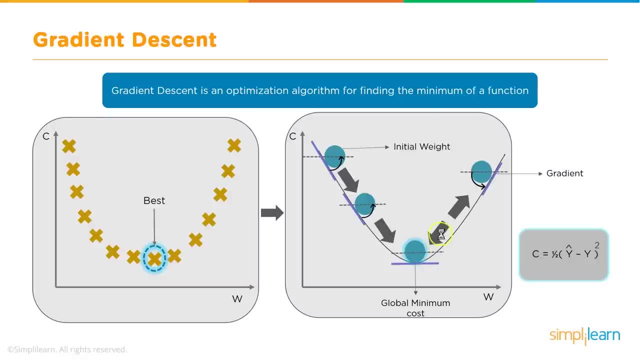 point it may reach the minimum value and then it may increase. so that is where the gradient descent algorithm decides that, okay, it has reached a minimum value and it will kind of try to stay here. this is known as the global minima. now, sometimes these curves may not be just for explanation purpose. this has been 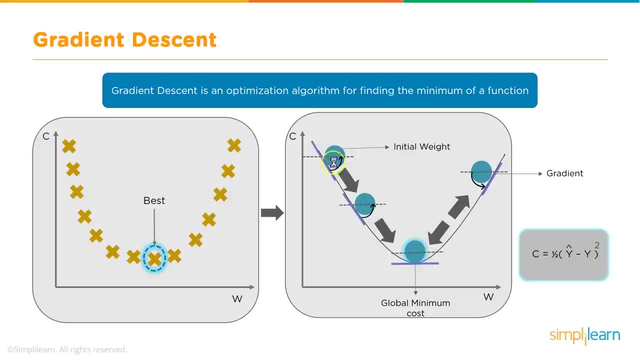 drawn in a nice way, but sometimes these curves can be pretty erratic. there can be some local minima here and then there is a peak, and then and so on. so the whole idea of gradient descent optimization is to identify the global minima and to find the weights and the bias at that. 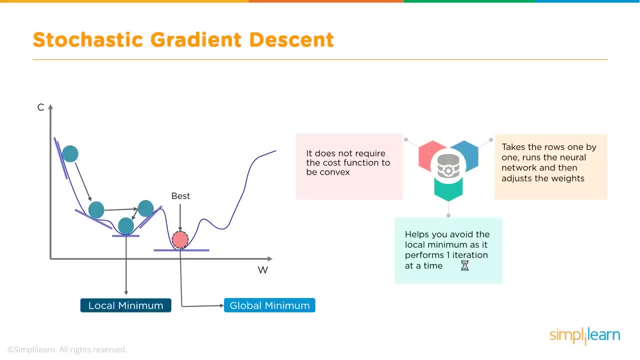 particular point. so that's what is gradient descent, and then this is another example, so you can have these multiple local minima. so, as you can see, at this point, when it is coming down, it may appear like this is a minimum value, but then it is not. this is actually the global minimum value and the gradient descent. 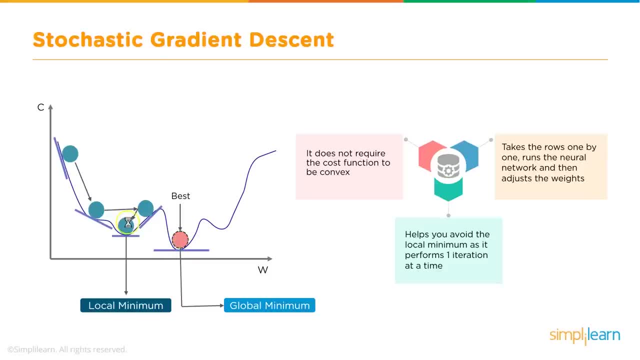 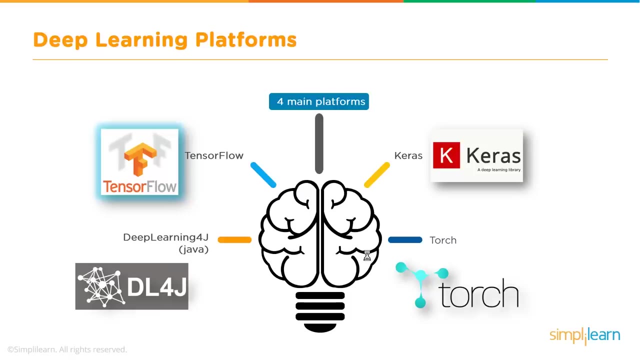 algorithm will make an effort to reach this level and not get stuck at this point. so the algorithm is already there and it knows how to identify this global minimum, and that's what it does during the training process. now, in order to implement deep learning, there are multiple platforms and languages that 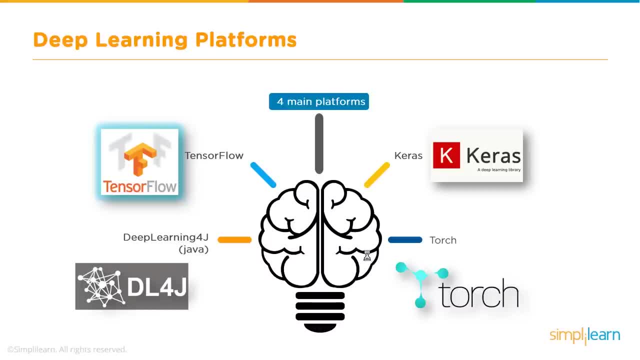 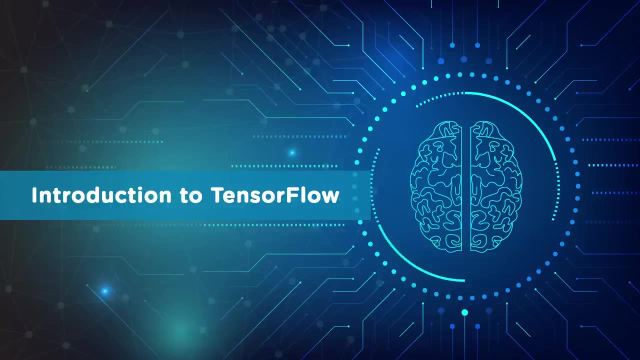 are available, but the most common platform nowadays is tensorflow, and so that's the reason we have this tutorial. we created this tutorial for tensorflow, so we will take you through a quick demo of how to write a tensorflow code using Python, and tensorflow is an open source platform created by Google, so let's just take a. 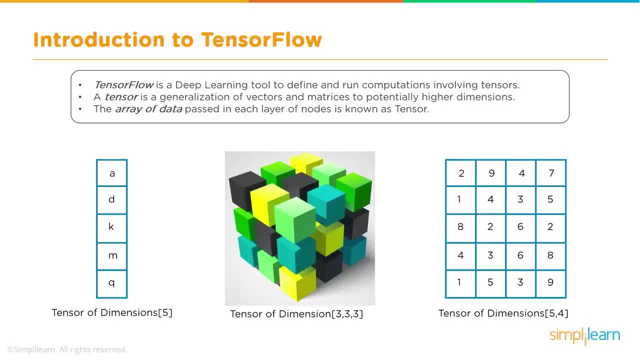 look at the details of tensorflow, and so this is a library, a Python library, so you can use Python or any other languages. it's also supported in other languages like Java and R and so on, but Python is the most common language that is used, so it is a library for. 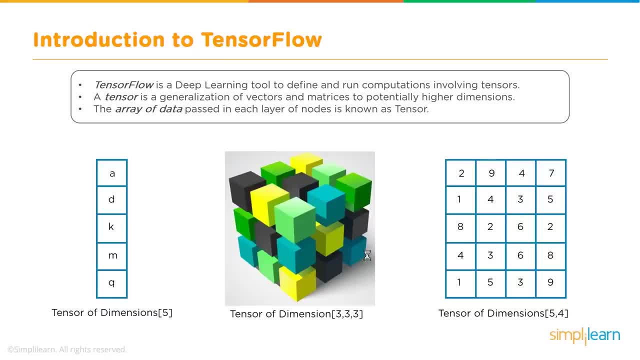 developing deep learning applications, especially using neural networks, and it consists of primarily two parts, if you will. so one is the tensors and then the other is the graphs or the flow. that's the way, the name, that's the reason for this kind of a name called tensorflow. so what are tensors? tensors are like. 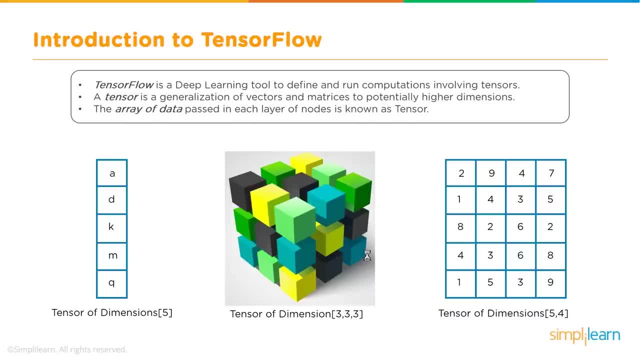 multi-dimensional arrays. well, that's one way of looking at it. so usually you have a one-dimensional array. so first of all you can have what is known as a scalar, which means a number, and then you have a one-dimensional array, something like this, which means this: like a set of numbers. so that is a one-dimensional array. then you can have 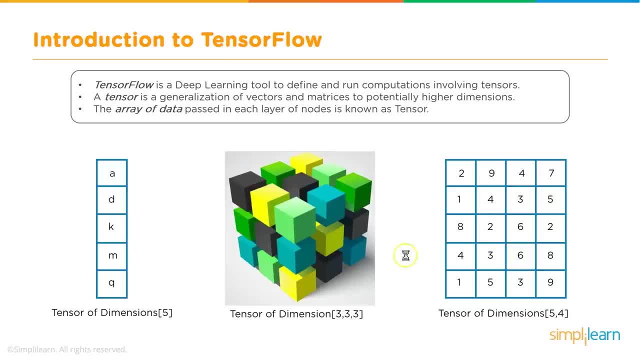 a two-dimensional array which is like a matrix, and beyond that sometimes it gets difficult. so this is a three-dimensional array, but tensorflow can handle many more dimensions, so it can have multi-dimensional arrays. that is the strength of tensor flow and which makes computation, deep learning, computation- much faster, and that's the reason why tensorflow is used. 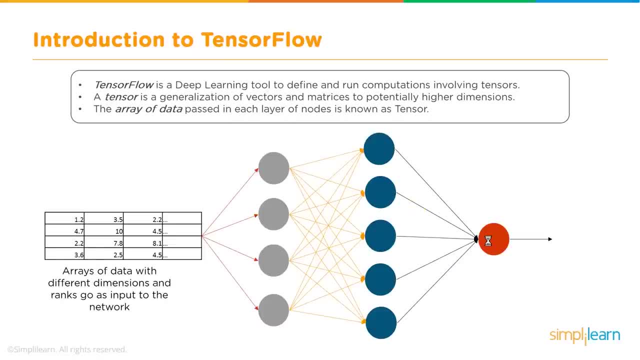 for developing deep learning applications. so tensorflow is a deep-learning tool and this is the way it works. so the data basically flows in the form of tensors, and the way the programming works as well is that you first create a graph of how to execute it and you actually execute that particular graph in the form of what is known as a session. We will see. 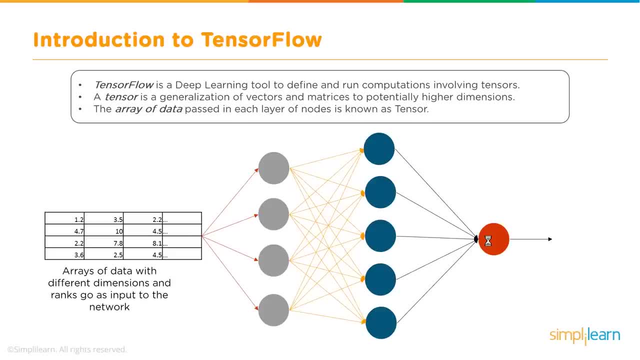 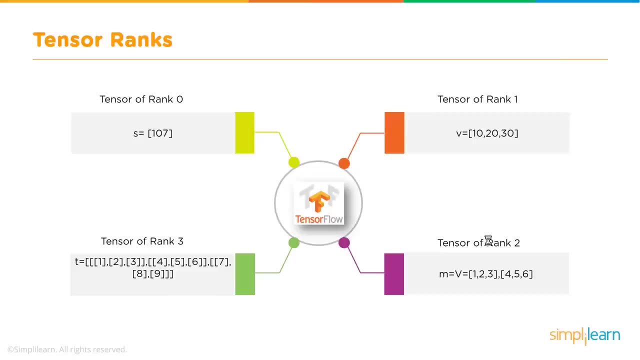 this in the tensor flow code as we move forward. So all the data is managed or manipulated in tensors and then the processing happens using these graphs. There are certain terms called like, for example, ranks of a tensor. The rank of a tensor is like a dimensional dimensionality in 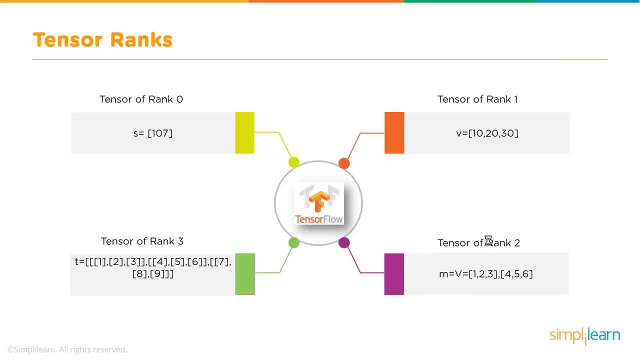 a way. So, for example, if it is scalar, so there is just a number, just one number, the rank is supposed to be zero, and then it can be a one-dimensional vector, in which case the rank is supposed to be one, and then you can have a two-dimensional vector, typically like a matrix. 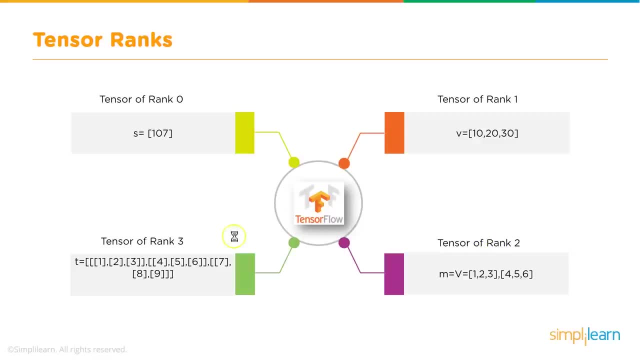 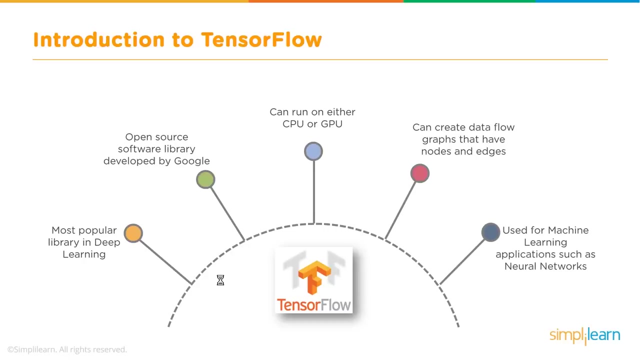 Then in that case we say the rank is two, and then if it is a three-dimensional array, then rank is three and so on, So it can have more than three as well. So it is possible that you can store multi-dimensional arrays in the form of tensors. So what are some of the properties of tensor flow? I think today it is. 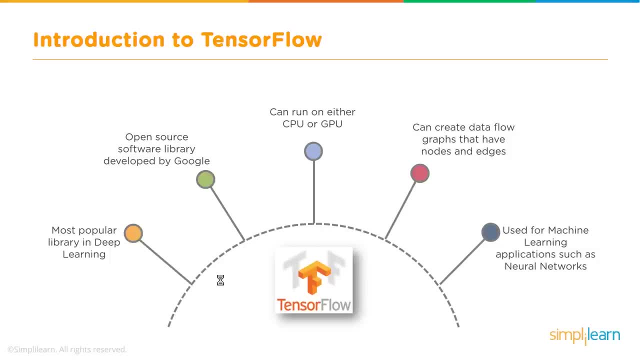 one of the most popular platforms. Tensor flow is the most popular deep learning platform or library. It is open source. it is developed by Google, developed and maintained by Google, but it is open source. One of the most important things about tensor flow is that it can run on. 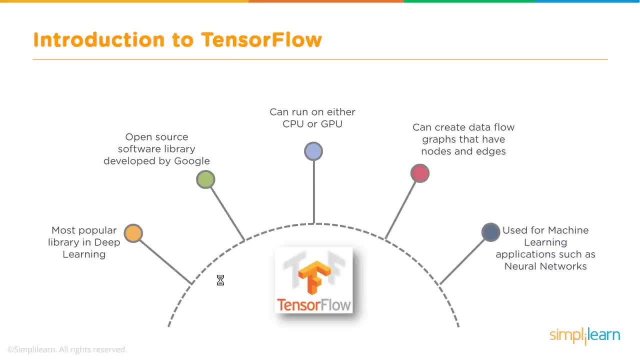 CPUs as well as ZIPs, GPUs. GPU is a graphical processing unit, just like CPU is central processing unit. Now, in earlier days, GPU was used for- primarily for- graphics, and that's how the name has come, and one of the reasons is that it cannot perform generic activities very efficiently like CPU, but it can. 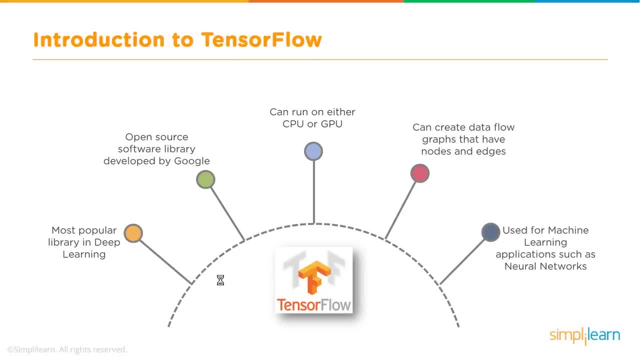 perform iterative actions or computations extremely fast and much faster than a CPU, So they are really good for computational activities. and in deep learning there is a lot of iterative computation that happens so in the form of matrix, multiplication and so on. So GPUs are very well suited for this kind of computation and TensorFlow supports both GPU as well as CPU. 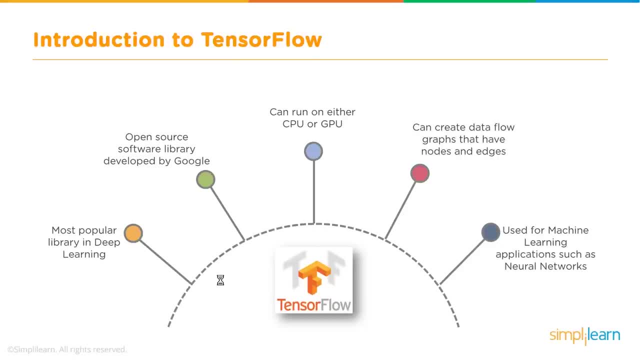 and there's a certain way of writing code in TensorFlow. we will see as we go into the code. and of course TensorFlow can be used for traditional machine learning as well, but then that would be an overkill. but just for understanding the concept of machine learning understanding, it may be a good idea to start writing code for a normal machine learning use. 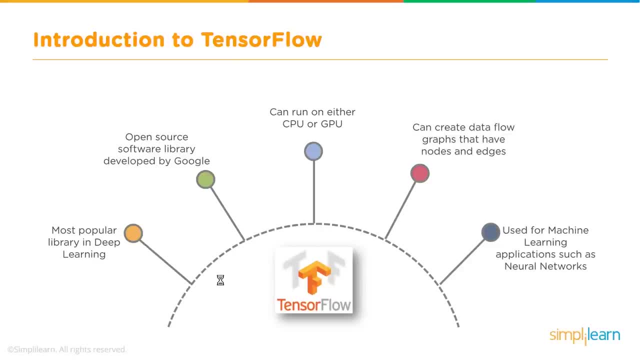 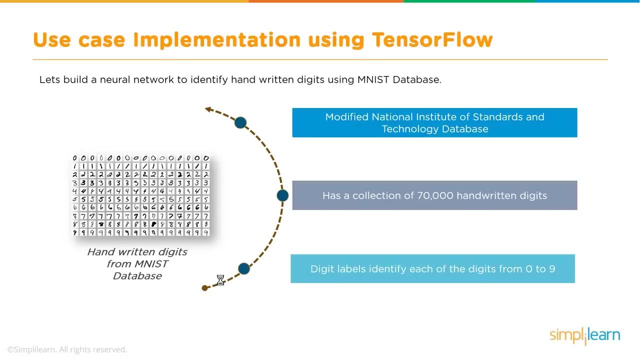 case, so that you get a hang of how TensorFlow code works and then you can move into neural networks. So that is just a suggestion, but if you're already familiar with how TensorFlow works, then probably, yeah, you can go straight into the neural networks part. So in this tutorial we will take the use case. 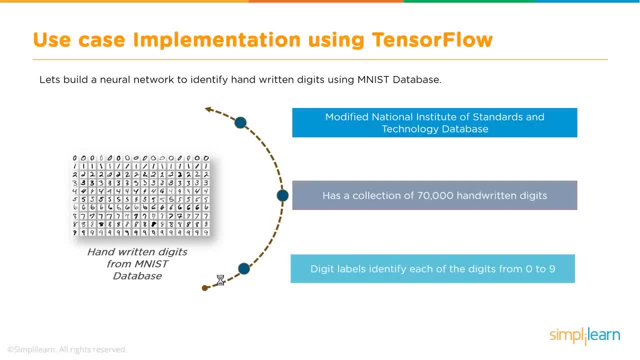 this is like a hello world of deep learning and this is a nice little MNIST database is a nice little database that has images of handwritten digits nicely formatted, because very often in deep learning and neural networks we end up spending a lot of time in preparing the data. 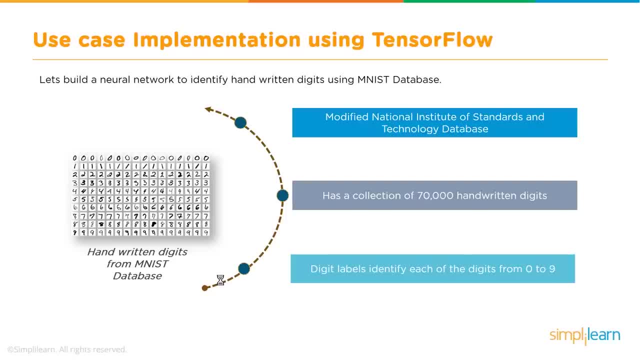 for training and with MNIST database we can avoid that. you already have the data in the right format directly used for training. and MNIST also offers a bunch of built-in utility functions that we can straight away use and call those functions without worrying about writing our own functions. and 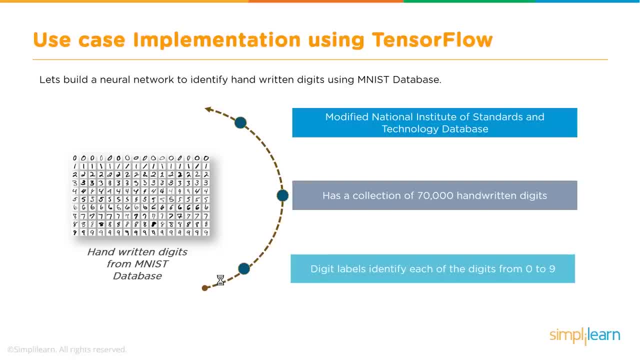 that's one of the reasons why MNIST database is very popular for training purposes. initially, when people want to learn about deep learning and TensorFlow, this is the database that is used and it has a collection of 70 000 handwritten digits and a large part of them are for training. then you have test, just like in any machine learning. 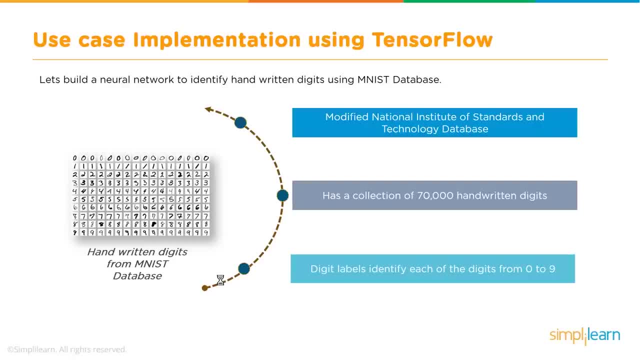 process and then you have validation and all of them are labeled. so you have the images and their label and these images- they look somewhat like this, so they are handwritten images collected from a lot of individuals people have. these are samples written by human beings. they have handwritten these numbers, these numbers. 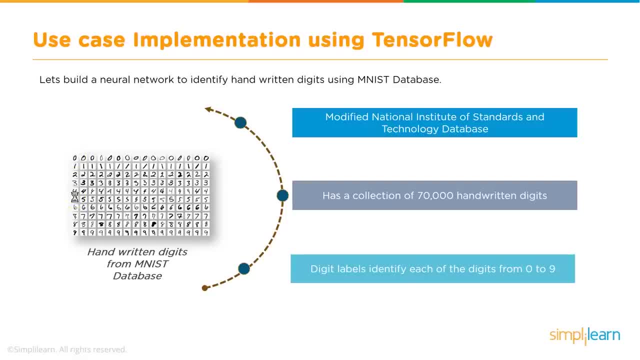 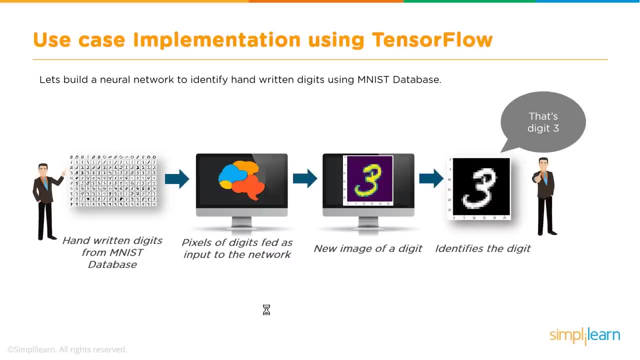 from zero to nine. so people have written these numbers and then the images of those have been taken and formatted in such a way that it is very easy to handle. so that is MNIST database, and the way we are going to implement this in our TensorFlow is we will feed this data especially. 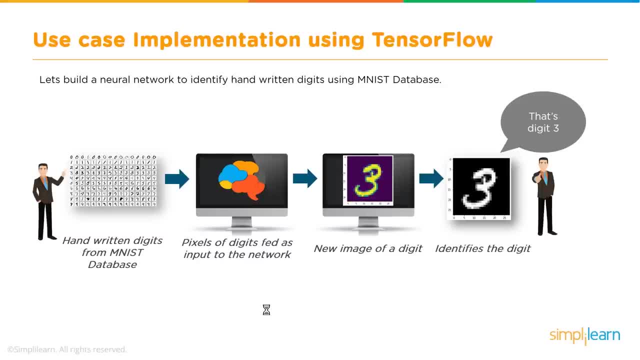 the training data, along with the label information, and the data is basically: these images are stored in the form of the pixel information. as we have seen in one of the previous slides, all the images are nothing but these are pixels. so an image is nothing but an arrangement of pixels and the value. 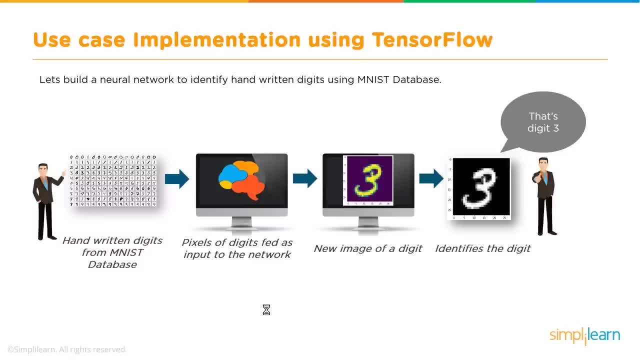 of the pixel. either it is lit up or it is not, or in somewhere in between. that's how the images are stored and that is how they are fed into the neural network and for training. once the network is trained, when you provide a new image, it will be able to. 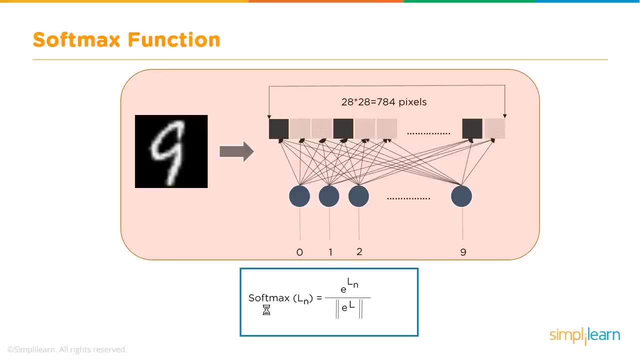 identify within a certain error, of course, and for this we will use one of the simpler neural network configurations called softmax. and, for simplicity, what we will do is we will flatten these pixels. so, instead of taking them in a two-dimensional arrangement, we just flatten them out. so, for example, it starts from here: it is a 28 by 28, so there are 784 pixels, so pixel number. 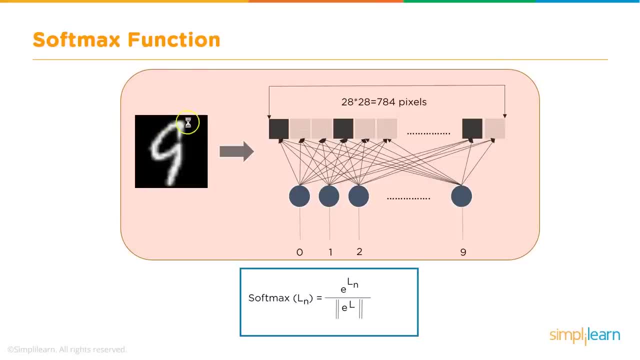 one starts here, it goes all the way up to 28, then 29 starts here and goes up to 56 and so on, and the pixel number 784 is here. so we take all these pixels, flatten them out and feed them like one single line into our neural network, and this is a what is known as a softmax layer. what 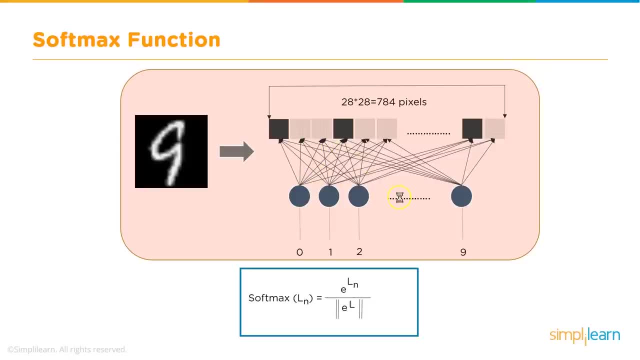 it does is, once it is trained, it will be able to identify what digit this is. so there are in this output layer, there are 10 neurons each signifying a digit, and at any given point of time when you feed an image, only one of these 10 neurons gets activated. so, for example, if 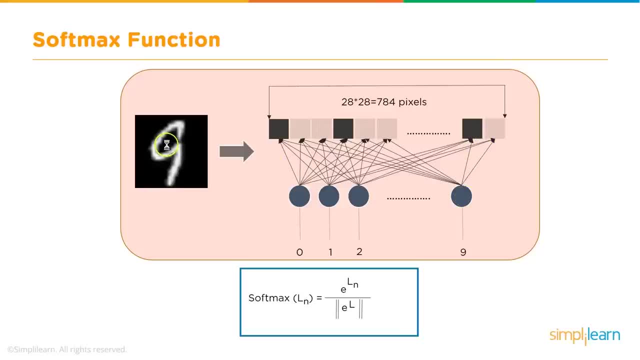 this is strained properly and if you feed a number nine like this, then this particular neuron gets activated, so you get an output from this neuron. let me just use a pen or a laser to show you here. okay, so you're feeding a number nine. let's say this has been trained and 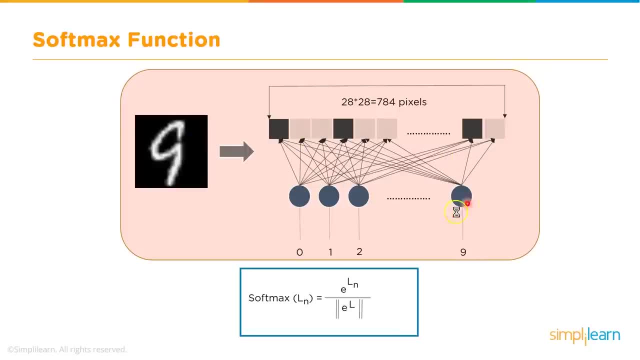 now, if you're feeding a number nine, this will get activated. now let's say, you feed one to the trained network, then this neuron will get activated. if you feed two, this neuron will get activated, and so on. I hope you get the idea. so this is one type of a neural network or an activation function known. 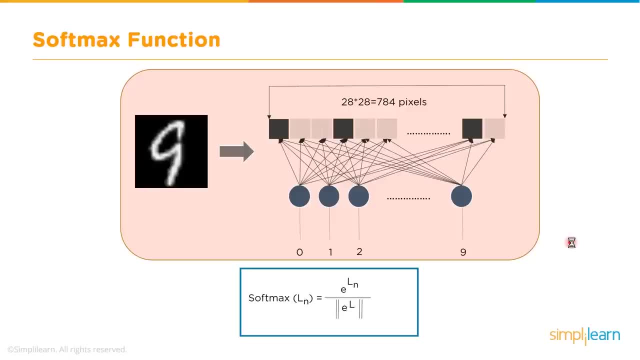 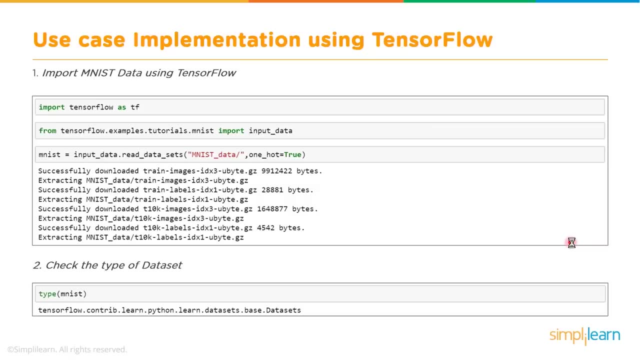 as softmax layer, so that's what we will be using here. this is one of the simpler ones for quick and easy understanding. so this is how the code would look. we will go into our lab environment in the cloud and we will show you there directly, but very quickly. this is how the code looks, and let me run you through briefly here and then we 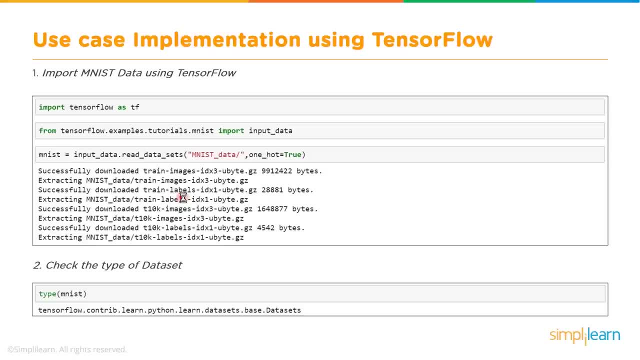 will go into the Jupiter notebook where the actual code is, and we will run that as well. so, as a first step, first of all, we are using python here, and that's why the syntax of the language is python, and the first step is to import the tensorflow library. so, and we, 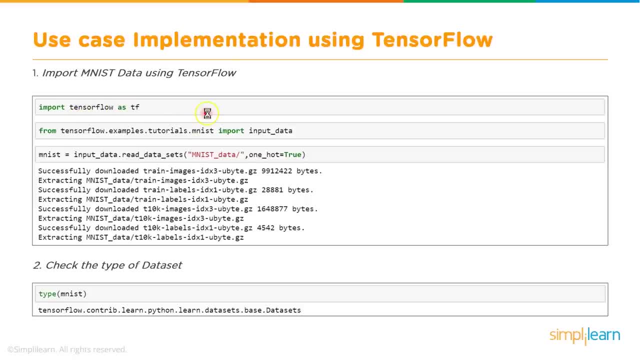 do this by using this line of code saying: import tensorflow as tf. tf is just for convenience, so you can name, give any name and once you do this, tf is, tensorflow is available as an object in the name of tf and then you can run its methods and accesses its attributes and so on and so forth, and mnist. 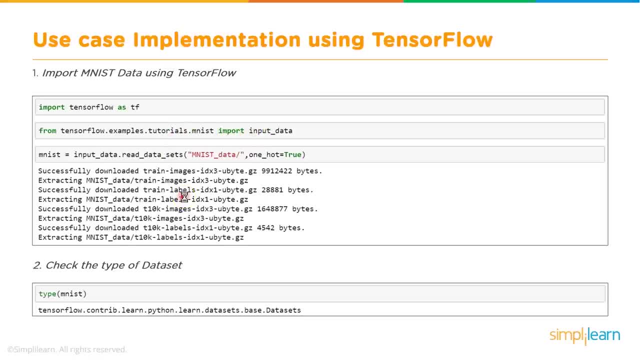 is a integral part of tensorflow, and that's again another reason why we, as a first step, we always use this example, mnist database example. so you just simply import mnist database as well using this line of code and you slightly modify this so that the labels are in this format: what is known? 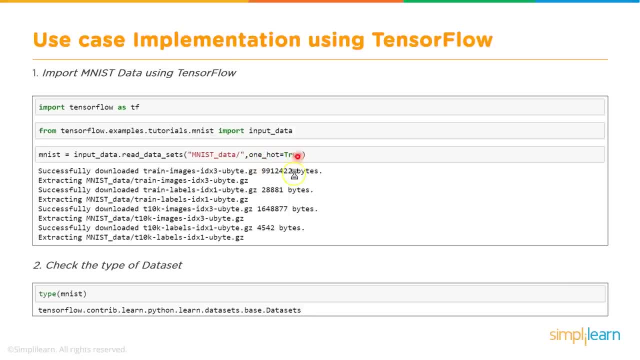 as one hot true, which means that the label information is stored like an array, and let me just use the pen to show what exactly it is. so when you do this one hot true, what happens is each label is stored in the form of an array of 10 digits, and let's say the number is, uh, eight, okay, so in this case, all. 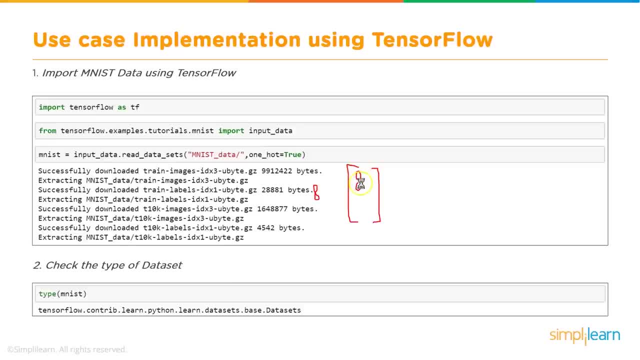 the remaining values. there will be a bunch of zeros, so this is like array. at position zero, this is at position one, position two and so on and so forth. let's say this is position seven, then this is position eight, that will be one because our input is eight, and again position nine. 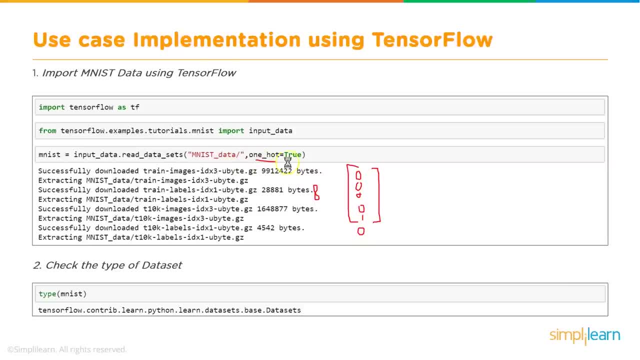 will be zero. okay, so one hot encoding this, one hot encoding true will kind of load the data in such a way that the labels are in such a way that only one of the digits has a value of one and that indicates so based on which digit is one, we know what is the label. so in this case, the eighth. 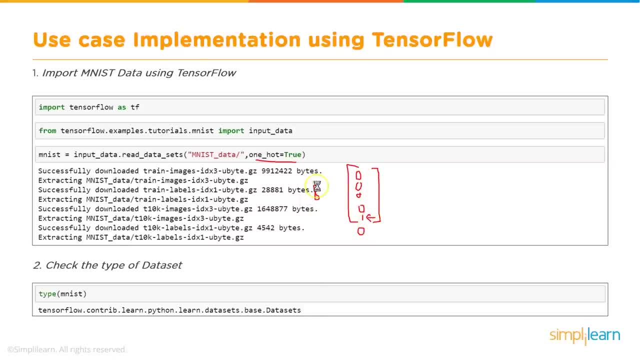 position is one. therefore, we know this sample data. the value is eight. similarly, if you have a two here, let's say, then the labeled information will be somewhat like this: so you have your labels. so you have this as zero: the zeroth position. the first position is also zero. the second position: 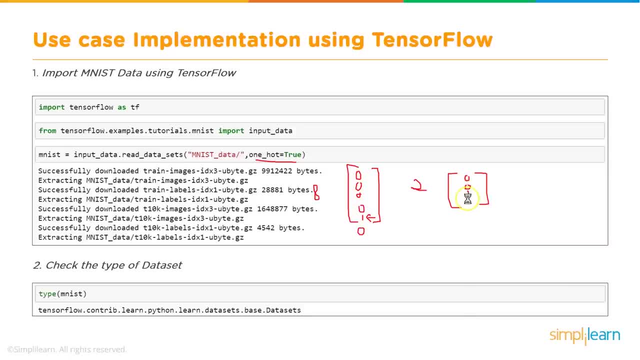 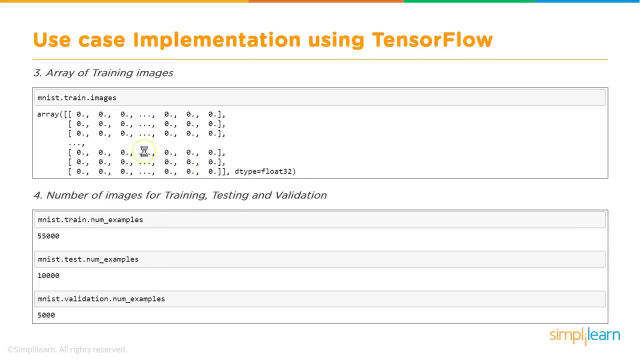 is one, because this indicates number two, and then you have third as zero, and so on. okay, so that is the significance of this: one, hot, true, all right. and then we can check how the data is looking by displaying the data and, as i mentioned earlier, this is pretty. 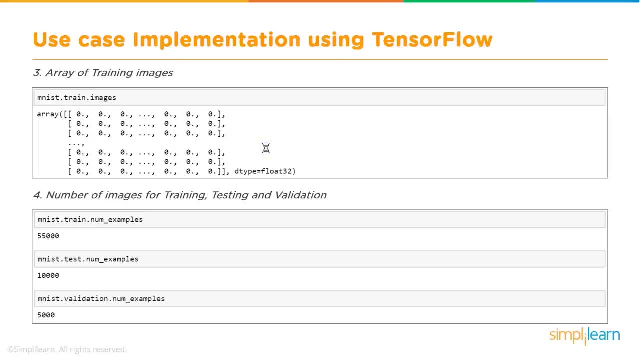 much in the form of digital form, like numbers. so all these are like pixel values. so you will not really see an image in this format. but there is a way to visualize that image. i will show you in a bit and this tells you how many images are there in each set. so the training there are 55 000. 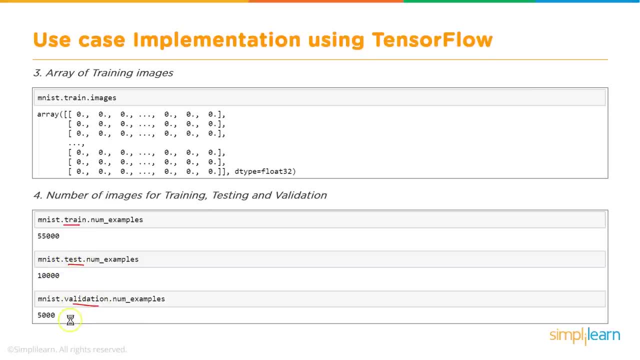 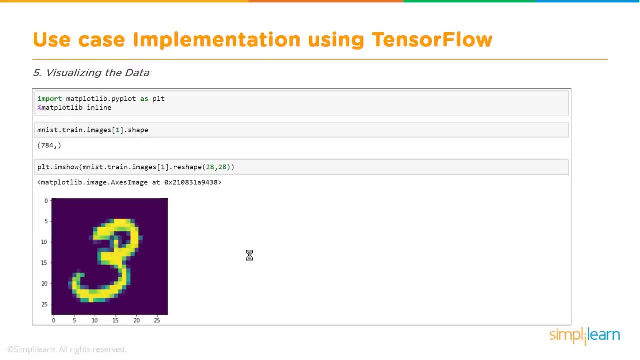 set, there are ten thousand, and then validation, there are five thousand. so all together there are seventy thousand images. all right, so let's uh move on and we can view the actual image by using the matplotlib library. and this is how you can view. this is the code for viewing the images. 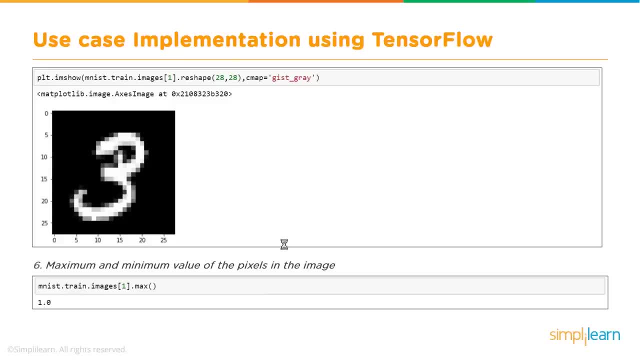 and you can view them in color or you can view them in grayscale. so the cmap is what tells in what way we want to view it and what are the maximum values and the minimum values of the pixel values. so these are the max and minimum values. so of the pixel values, so maximum is one, because this is a 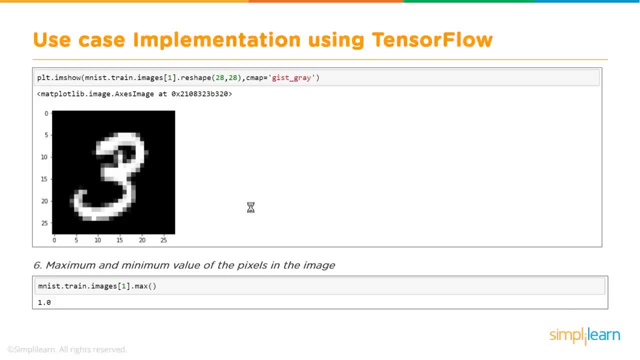 scaled value. so one means it is white and zero means it is black and in between is it can be anywhere in between black and white and the way to train the model. there is a certain way in which you write your model and you can use it to train your model and you can use it to train your model. 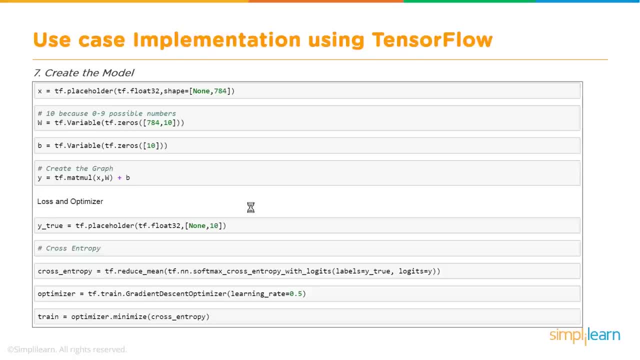 tensorflow code and the first step is to create some placeholders and then you create a model. in this case we will use the softmax model, one of the simplest ones, and placeholders are primarily to get the data from outside into the neural network. so this is a very common 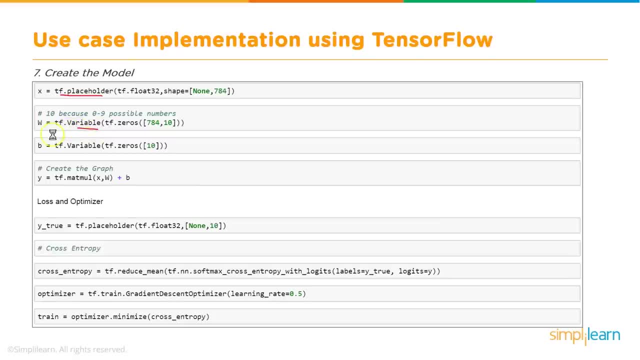 mechanism that is used. and then, of course, you will have variables, which are your. remember, these are your weights and biases. so for, in our case, there are 10 neurons and each neuron actually has 784, because each neuron takes all the inputs. if we go back to our slide, 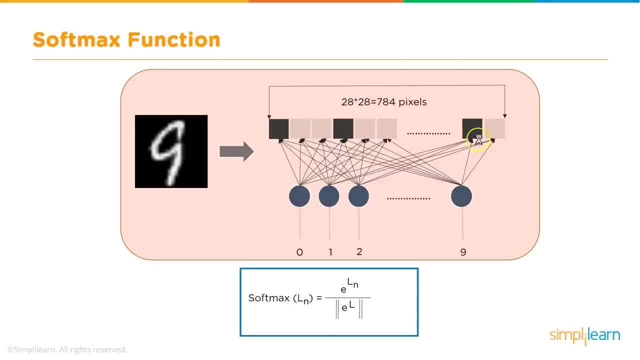 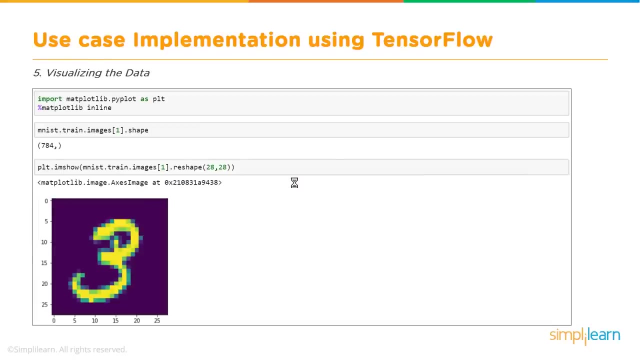 here. actually, every neuron takes all the 784 inputs, right? this is the first neuron. it has. it receives all the 784. this is the second neuron. this also receives all the 700. so each of these inputs needs to be multiplied with the weight, and that's what we are talking about here. so these are 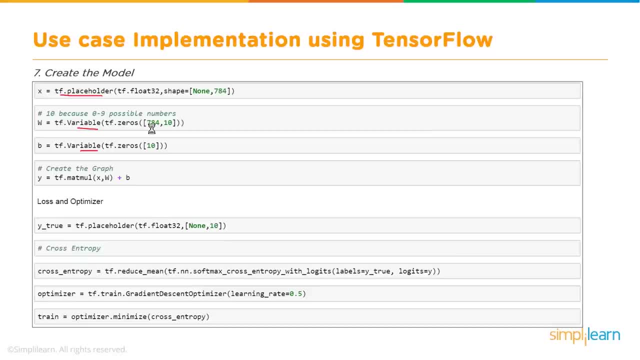 this is a matrix of 784 values for each of the neurons, and so it is like a 10 by 784 matrix, because there are 10 neurons and similarly there are biases. now remember i mentioned bias is only one per neuron, so it is not one per input, unlike the weights. so therefore there are only 10 biases. 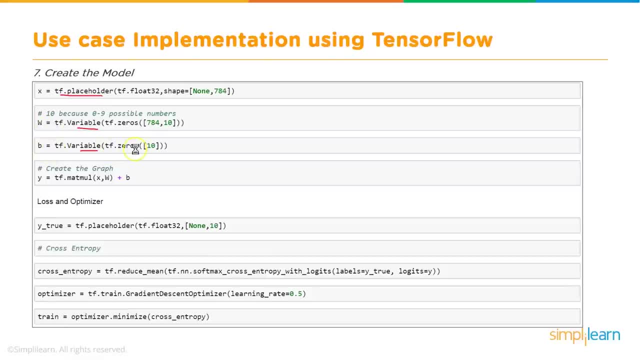 because there are only 10 neurons in this case. so that is what we are creating: a variable for biases. so this is something little new in tensorflow, you will see, unlike our regular programming languages where everything is a variable, here the variables can be of three different types. you have placeholders, which are primarily used for feeding data. you have 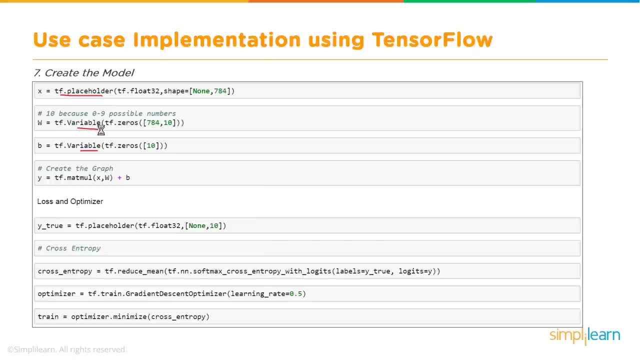 variables, which can change during the course of computation. and then a third type, which is not shown here, are constants. so these are like fixed numbers, all right. so in a regular programming, programming language, you may have everything, as variables are at the most variables and constants. but in tensorflow you have three different types: placeholders, variables and 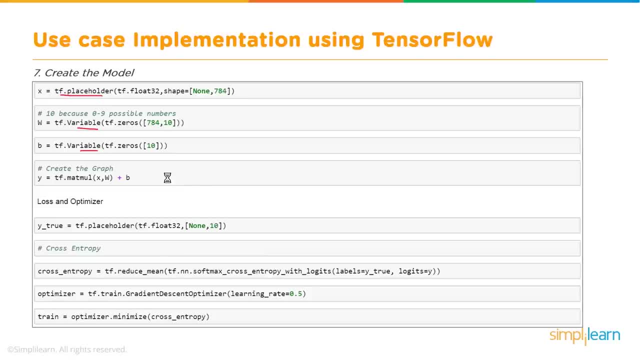 constants, and then you create what is known as a graph. so tensorflow programming consists of graphs and tensors, as i mentioned earlier. so this can be considered ultimately as a tensor, and then the graph tells how to execute the whole implementation, so that the execution is stored in the form of a graph. and in this case, what? for instance, we are using an example豆은илась. for an example, and she. this is just a home element of the program, so this was set up much earlier in the 我們 invent هذه независимость выход. grow on exe377. this is the test, by losing the part number and 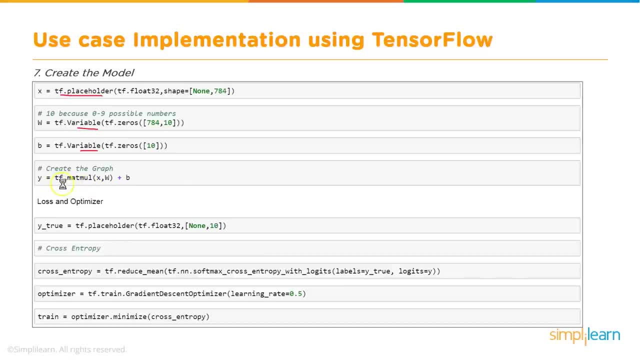 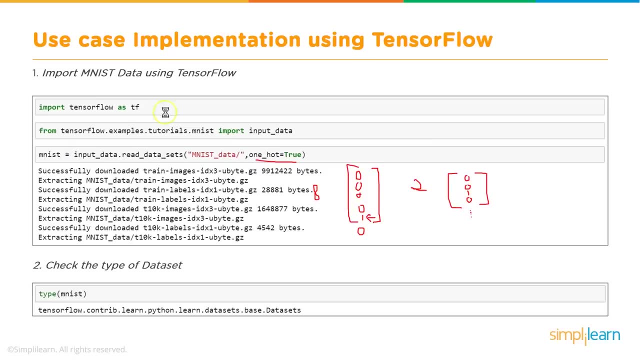 so that the version number of the program that is performed. we have not got this. the destruction for the. what we are doing is we are doing a multiplication tf. you remember this tf was created as a tensor flow object. here one more level, one more. so tf is available here. now tensorflow has what is known as. 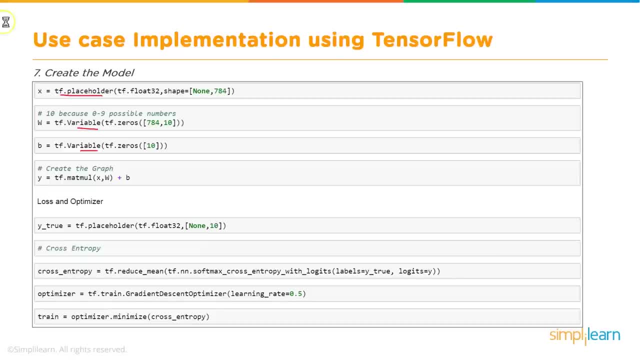 a matrix multiplication or matmul function. so that is what is being used here in this case. so we are using the matrix multiplication of tensorflow so that you multiply your input values x with w. right, this is what we were doing: x, w plus b. you are just adding b and this is in very similar to one. 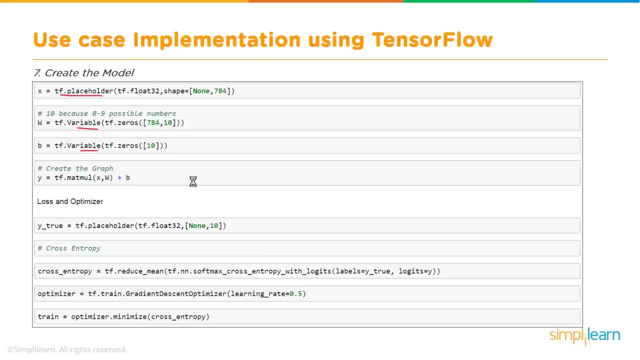 of the earlier slides where we saw sigma xi wi. so that's what we are doing here. matrix multiplication is multiplying all the input values with the corresponding weights and then adding the bias. so that is the graph we created, and then we need to define what is our loss function. 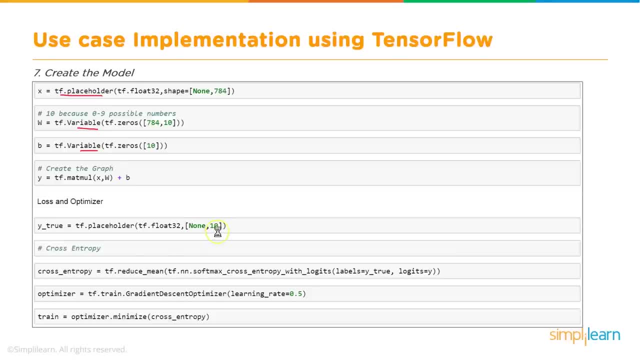 and what is our optimizer? so in this case, we again use the tensorflow's apis. so tf, dot, nn, softmax, cross entropy with logits is the api that we will use and reduce mean is what is like the mechanism whereby, which says that you reduce the error, and optimizer for doing reduction of the error. what optimizer are we using? 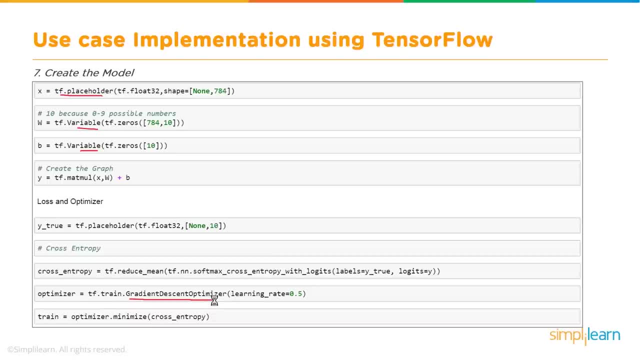 so we are using gradient descent optimizer- we discussed about this in a couple of slides earlier- and for that you need to specify the learning rate. you remember we saw that there was a slide somewhat like this- and then you define what should be the learning rate, how fast. 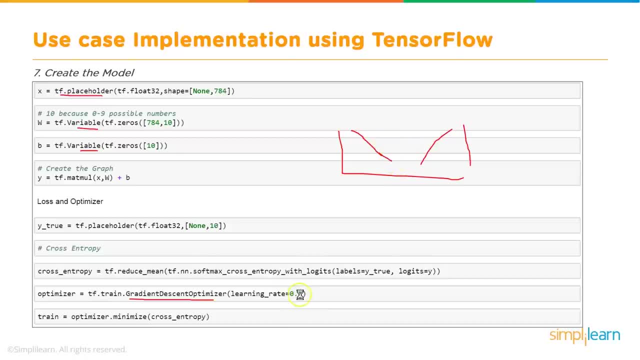 you need to come down. that is the learning rate, and this again needs to be tested and tried and to find out the optimum level of this learning rate. it shouldn't be very high, in which case it will not converge, or shouldn't be very low, because it will. in that case, it will take very long. so you 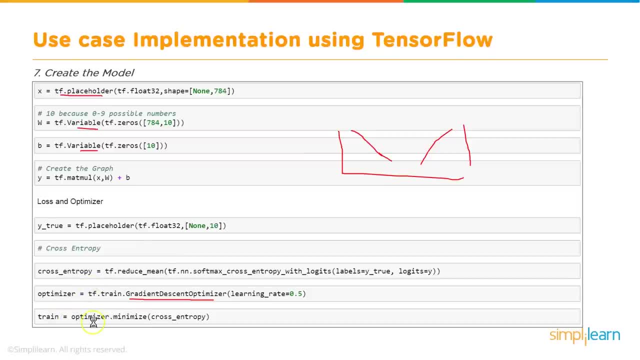 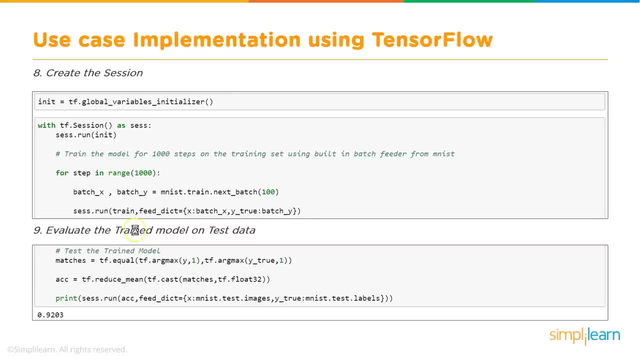 define the optimizer and then you call the method minimize for that optimizer and that will kick start the training process. and so far we've been creating the graph and in order to actually execute that graph, we create what is known as a session and then we run that session and once the training is, 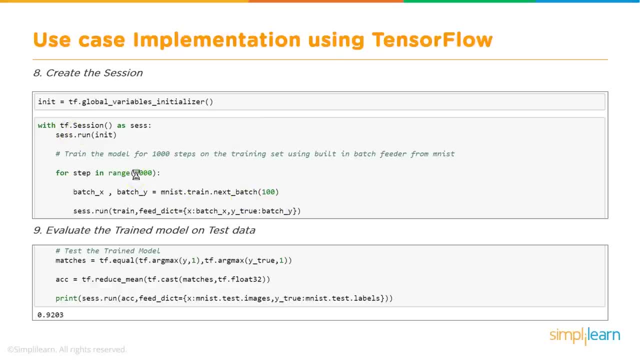 completed. we specify how many times, how many iterations we want it to run. so for example, in this case we are saying thousand steps. so that is a exit strategy in a way. so you'll specify the exit condition. so training will run for thousand iterations, and once that is done, 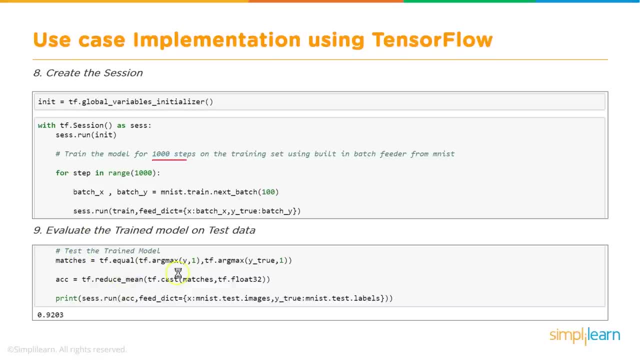 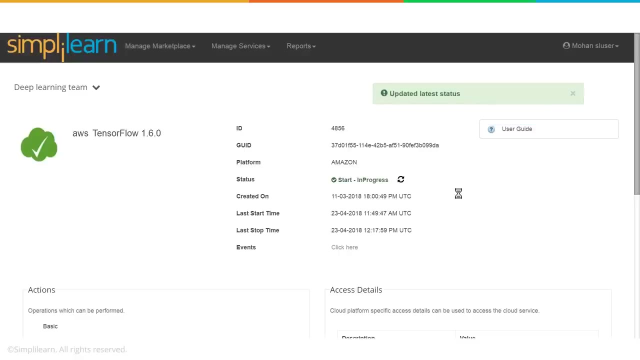 we can then evaluate the model using some of the techniques shown here. so let us get into the code quickly and see how it works. so this is our cloud environment. now you can install tensorflow on your local machine as well. i'm showing this demo on our existing cloud, but you can also install tensorflow. 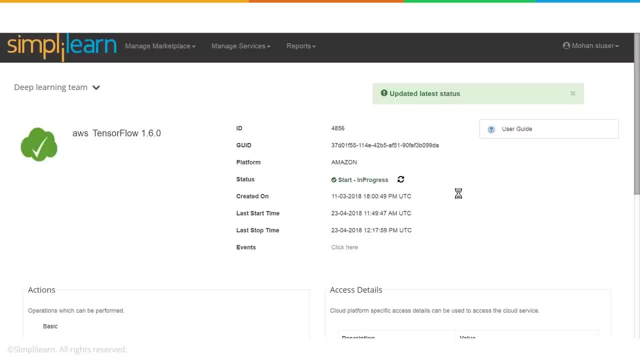 on your machine and there is a separate video on how to set up your tensorflow environment. you can watch that if you want to install your local environment, or you can go for other. any cloud service, like, for example, google cloud, amazon or cloud labs- any of these you can use and 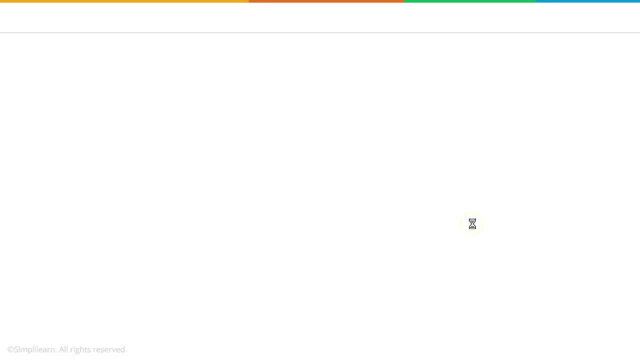 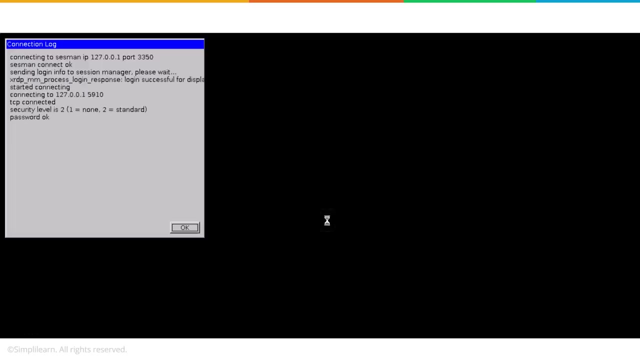 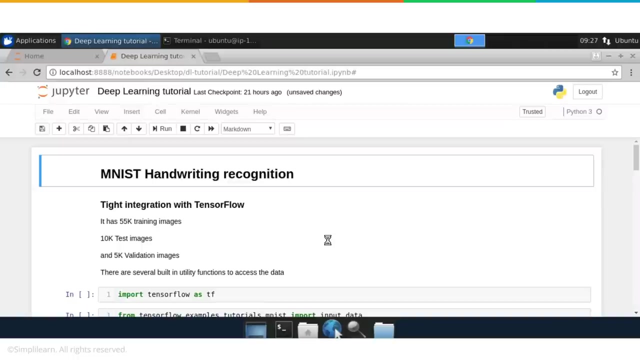 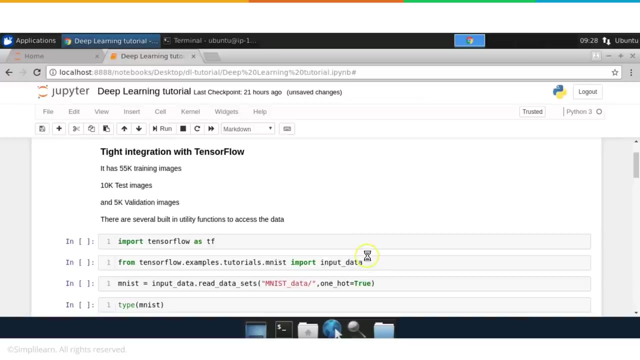 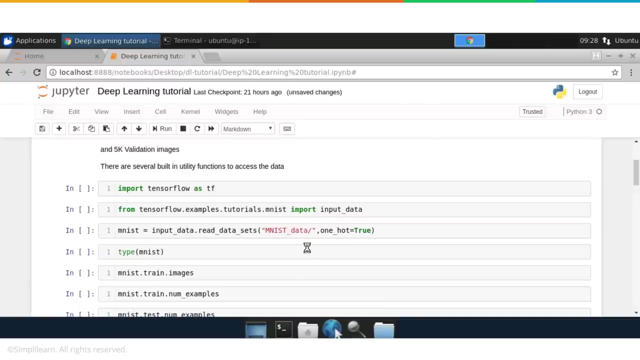 run and try the code. okay, so it has got started. we will log in. all right, so this is our deep learning tutorial code and this is our tensorflow environment, and so let's get started. the first: we have seen a little bit of a code walkthrough in the slides as well. now you will see the actual code in action. so the first thing we 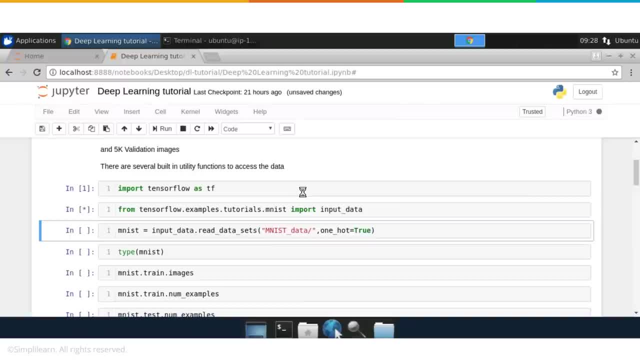 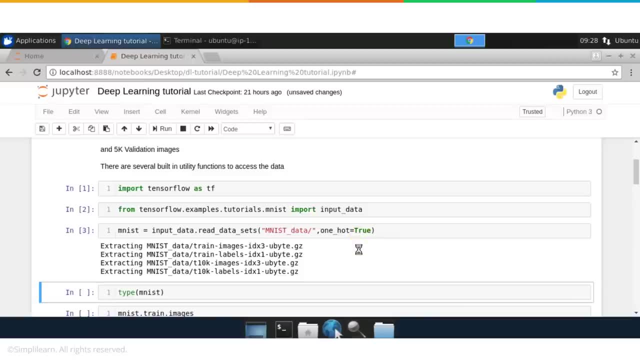 need to do is import tensorflow and then we will import the data and we need to adjust the data in such a way that the one hot is encoding is set to true, one hot encoding right, as i explained earlier. so in this case the label values will be shown appropriately. 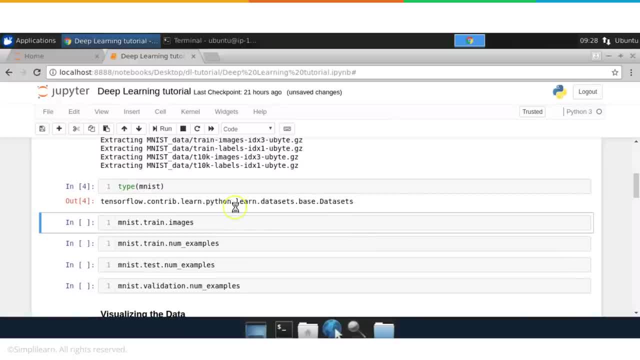 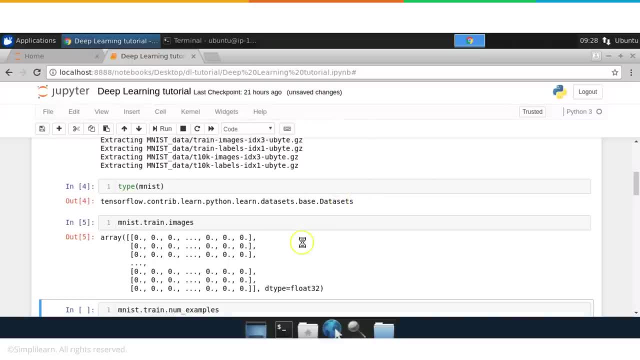 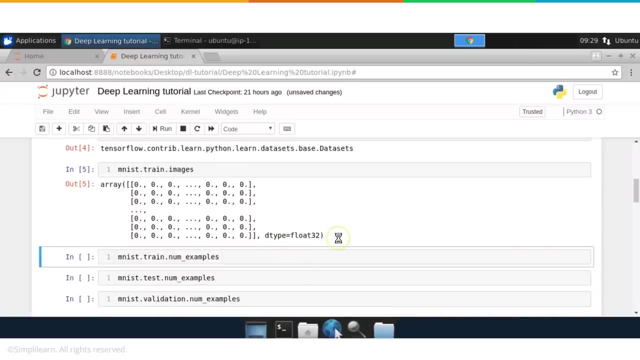 and if we just check what is the type of the data, so you can see that this is a our data sets, python data sets. and if we check the number of images, the way it looks. this is how it looks: it is an array of type float, 32.. Similarly the number. if you want to see what is the. 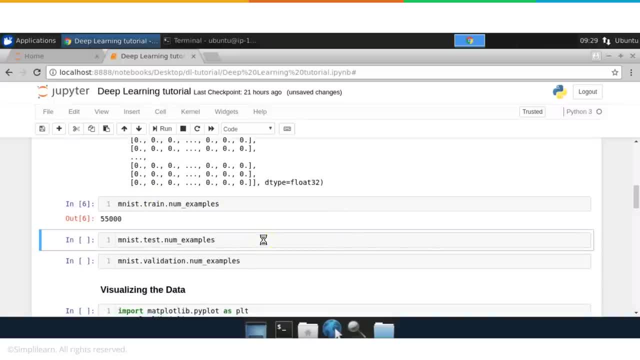 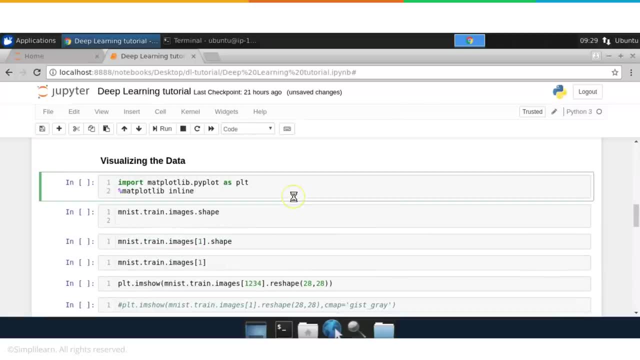 number of training images: there are 55,000, and there are test images- 10,000, and then validation images- 5000.. Now let's take a quick look at the data itself: visualization- So we will use matplotlib for this- And if we take a look at the shape now, shape gives. 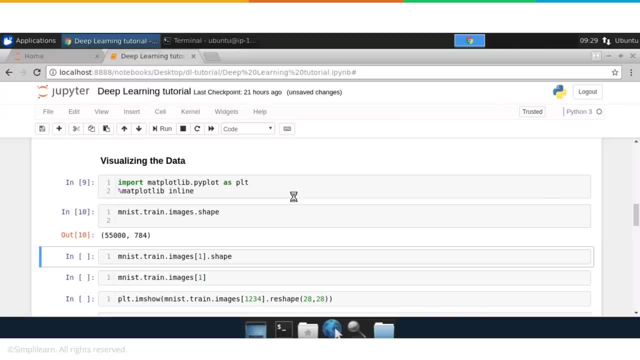 us like the dimension of the tensors, or or or the arrays, if you will, So in this case, the training data set. if we see the size of the training data set using the method shape, it says there are 55,000 and 55,000 by 784.. So, remember, the 784 is nothing but. 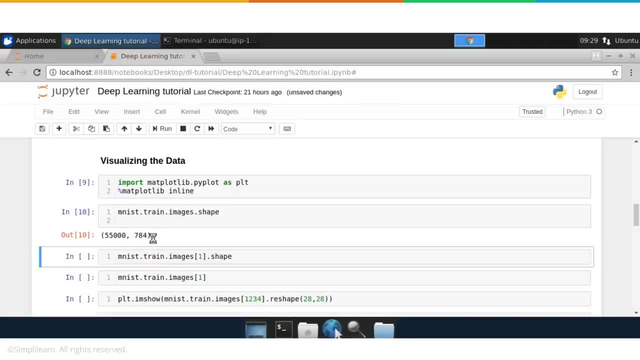 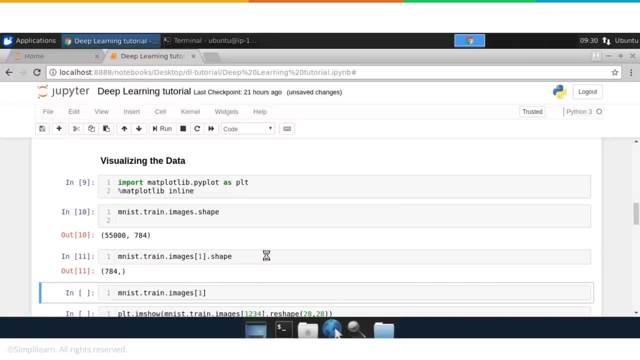 the 28 by 28.. 28 into 20.. 28.. So that is equal to 784.. So that's what it is showing. Now we can take just one image and just see what is the, the first image, and see what is the shape. So again, size obviously. 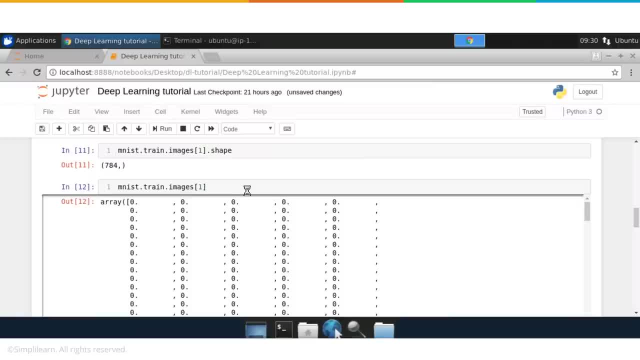 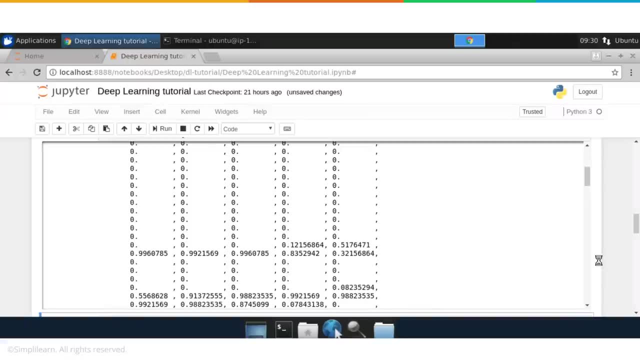 it is only 784.. Similarly, you can look at the image itself, the data of the first image itself. So this is how it shows. So large part of it will probably be zeros because, as you can imagine, in the image only certain areas are written. 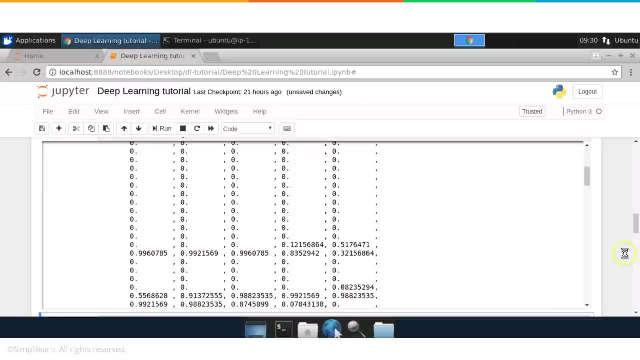 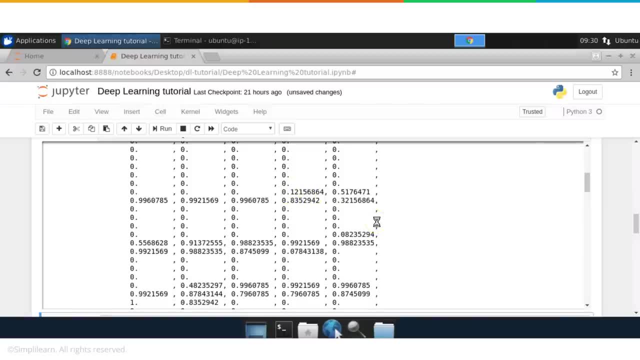 The rest is black. So that's why you will mostly see zero say that it is black or white. But then there are these values are. so the values are actually, they are scaled, So their values are between zero and one. Okay, so this is what you're seeing. So certain locations: 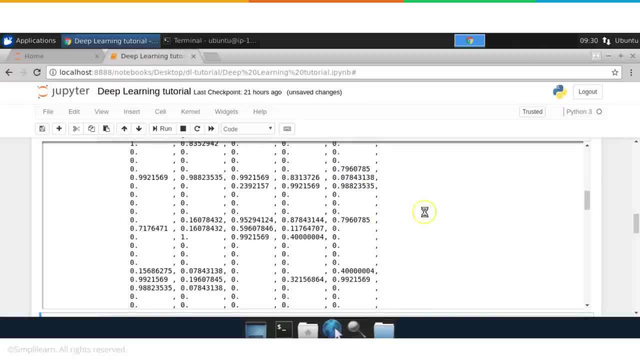 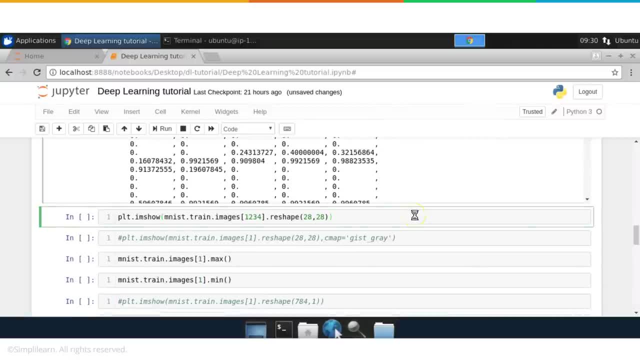 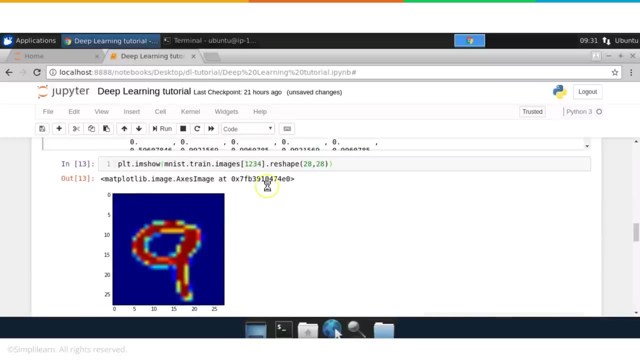 there are some values and then other locations. there are zeros. So that is how the data is stored and loaded, If we want to actually see what is the value of the handwritten image. if you want to view it, this is how you view it, So you create. 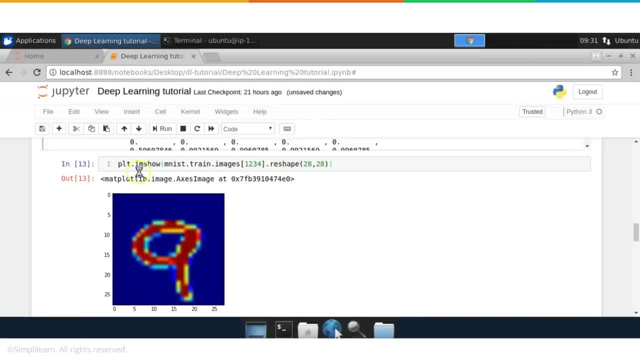 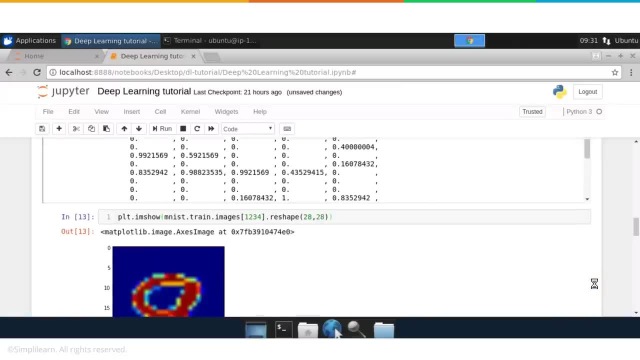 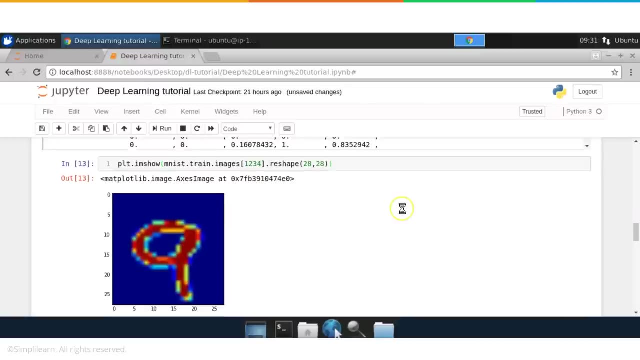 like do this reshape, and matplotlib has this feature to show you these images. So we will actually use the function called I am sure, and then, if you pass this parameters appropriately, you will be able to see the different images. now I can change the values in this position. 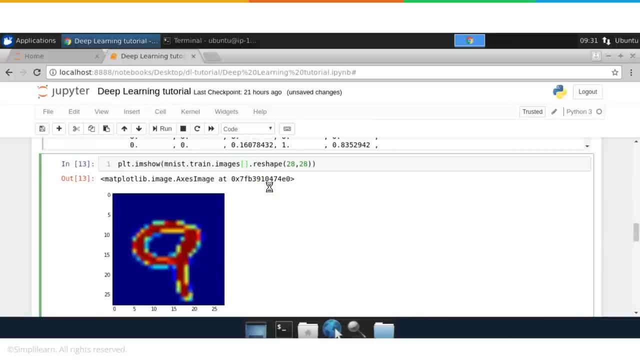 So which image we are looking at? right, so we can say: if I want to see what is there in, maybe 5000.. Right, So 5000 has three. Similarly, you can just say five. what is in five? five as eight. 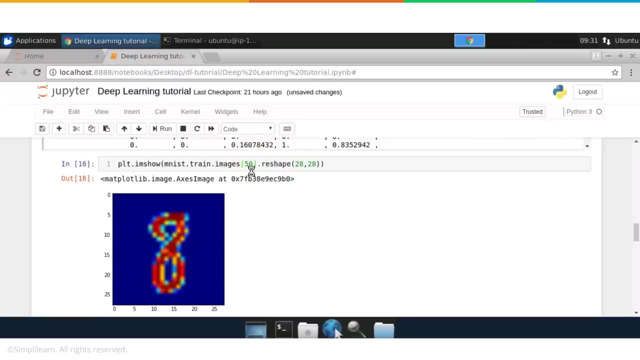 what is in 50?? Again, eight. So basically, by the way, if you're wondering how I'm executing this code, Shift Enter. In case you're not familiar with Jupyter Notebook, Shift Enter is how you execute each cell, individual cell. And if you want to execute, 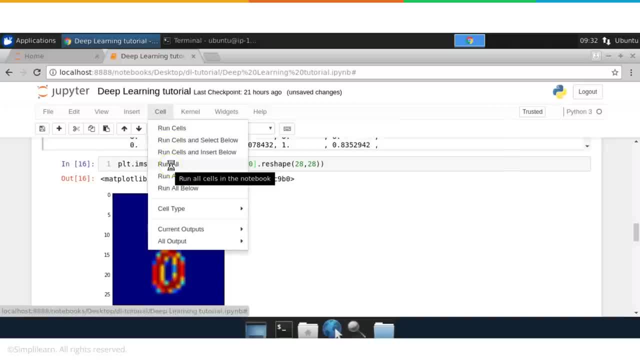 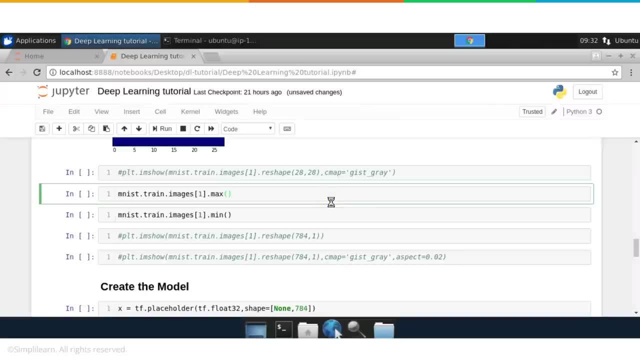 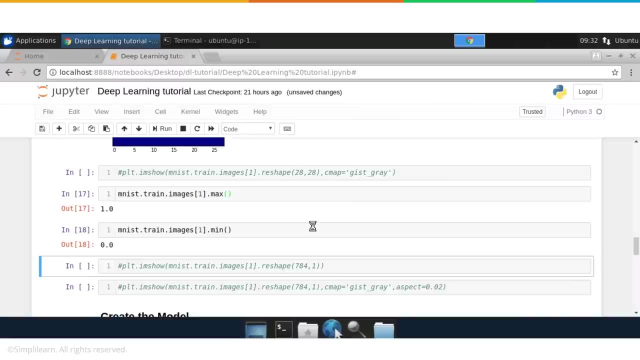 the entire program. you can go here and say run all. So that is how this code gets executed And here again we can check what is the maximum value and what is the minimum value of this pixel values. As I mentioned, this is it is scaled, So therefore it is between the values. 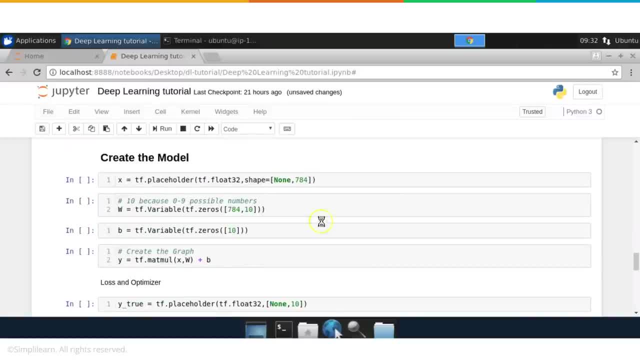 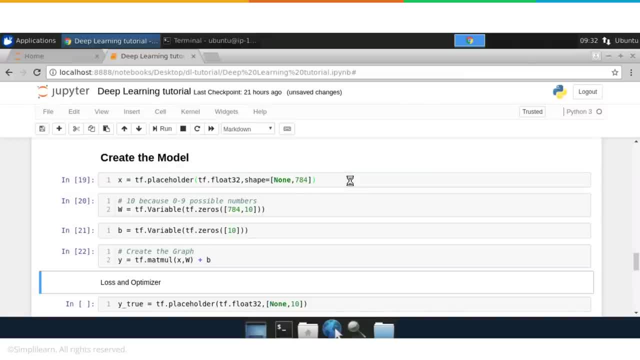 And that's what we are doing here, as we have seen in the slides. So we create one placeholder and we create two variables, which is for the weights and biases. These two variables are actually matrices, So each variable has seven and 84 by 10 cell values. Okay, so one for 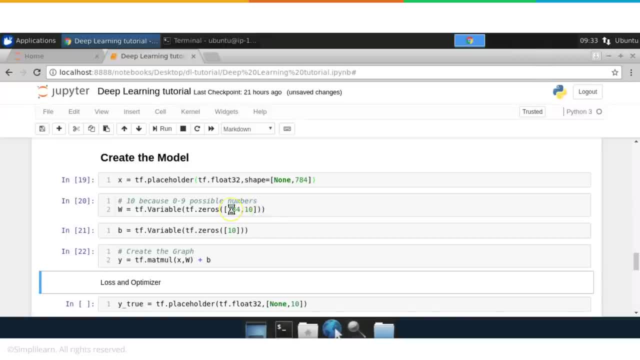 For this, 10 is for each neuron. there are 10 neurons and 784 is for the pixel values inputs that are given, which is 28 into 28.. And the biases, as I mentioned, one for each neuron. so there will be 10 biases. they are: 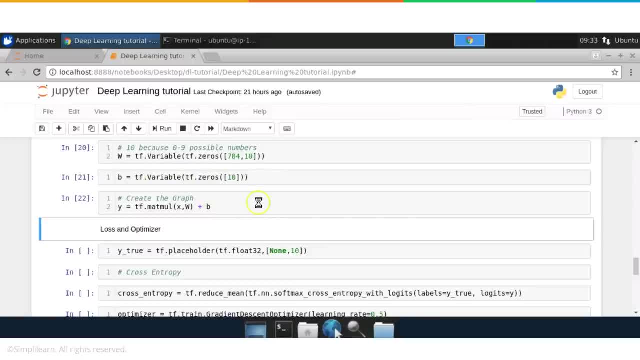 stored in a variable by the name B. And this is the graph which is basically the multiplication of these matrix, multiplication of x into w, and then the bias is added for each of the neurons, And the whole idea is to minimize the error. 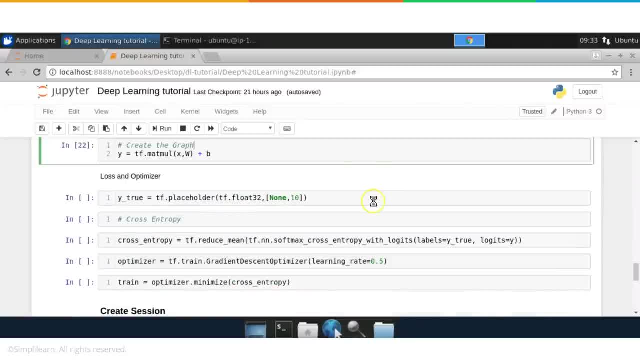 So let me just execute. I think this code is executed. then we define what is our. the y value is basically the label value, So this is another placeholder. we had x as one placeholder and white underscore, true as a second placeholder, And this will have values in the form of 10 digit, 10 digit arrays. 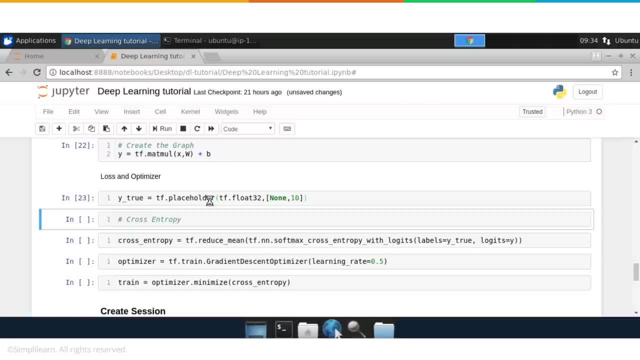 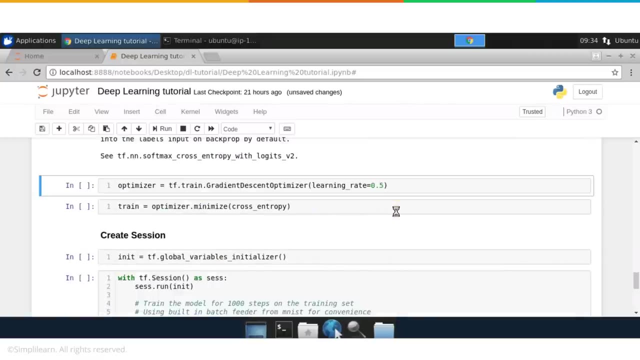 And since we said one hot encoded, the position which has a one value indicates what is the label for that particular number. All right, then we have cross entropy, which is nothing but the loss loss function, And we have the optimizer. we have chosen gradient descent as our optimizer, then the 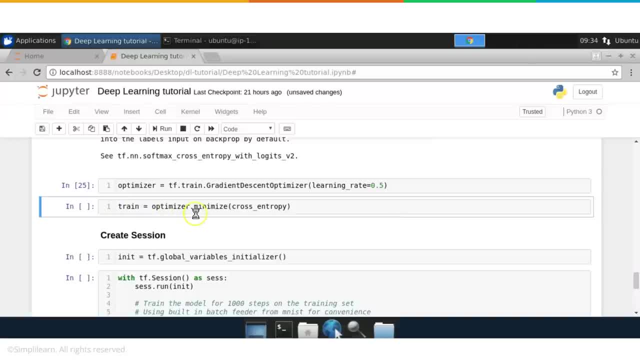 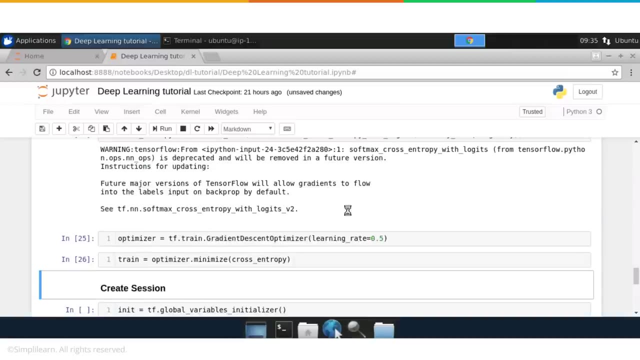 training process itself. So the training process is nothing but to minimize the cross entropy, which is again nothing but the loss function. So we define all of this in the form of a graph. So the up to here remember what we have done is we have not exactly executed any. 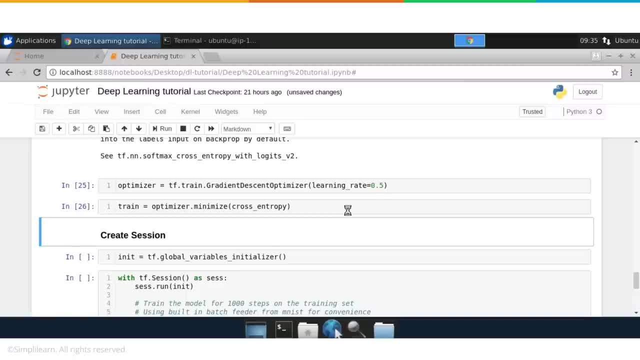 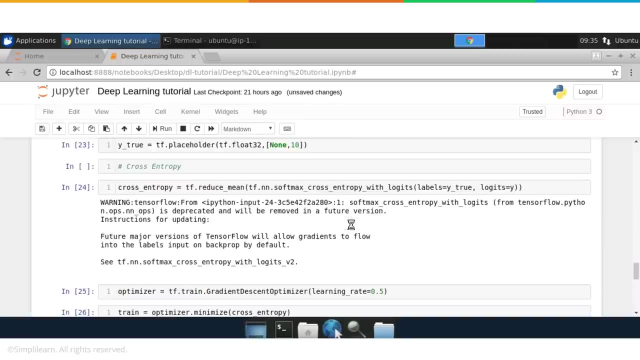 TensorFlow code. till now we are just preparing the graph, the execution plan. That's how the TensorFlow code works. So the whole structure and format of this code will be completely different from how we normally do programming. So even with People with programming experience may find this a little difficult to understand it. 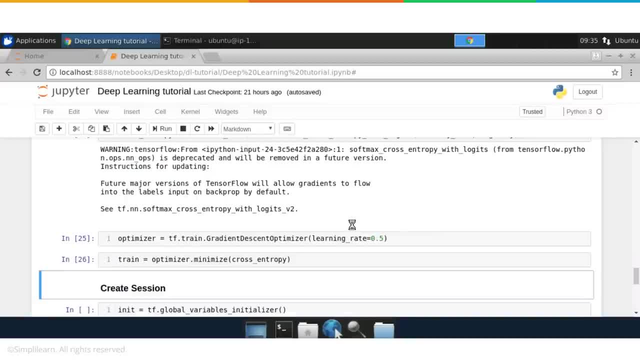 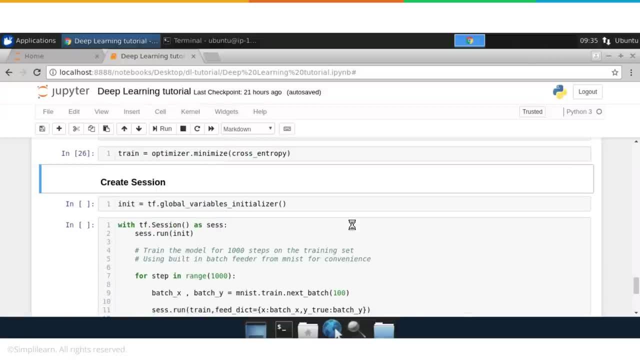 and it needs quite a bit of practice. So you may want to view this video also, maybe a couple of times, to understand this flow, Because the way TensorFlow programming is done is slightly different from the normal programming some of you who, let's say, have done maybe Spark programming to some extent. 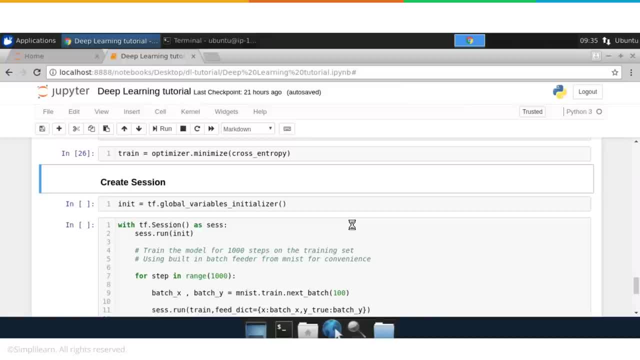 will be able to easily understand this. But even in Spark, the programming, the code itself, is pretty straightforward. Behind the scenes the execution happens slightly differently. But in TensorFlow even the code has to be written in a completely different way, So the code doesn't get executed in the same way as you have written. 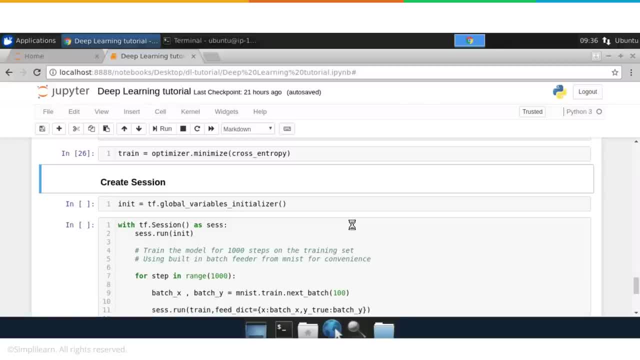 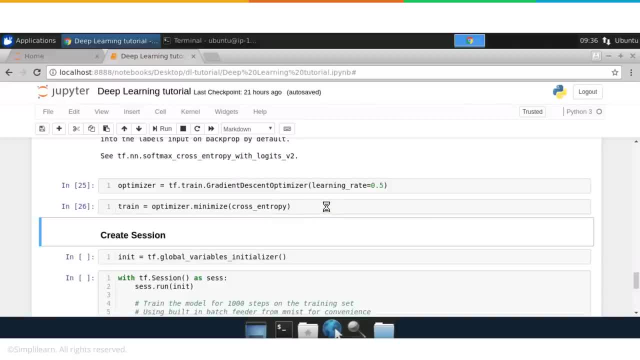 And feeding the variables, and rather not feeding but setting up the variables and the graph. That's all defining maybe the what kind of a network you want to use. For example, we want to use Softmax and so on. So you have created the variables. how to load the data, loaded the data, viewed the. 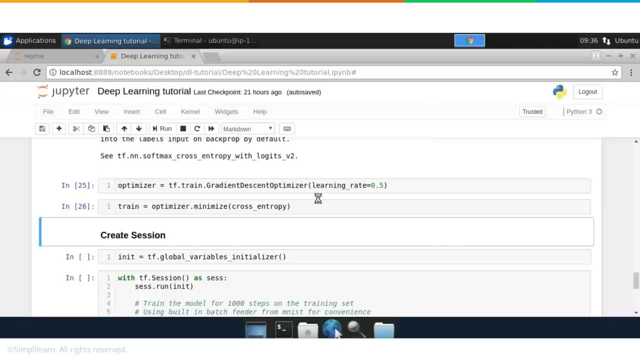 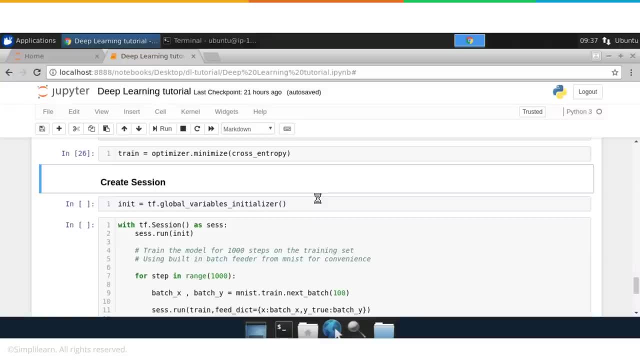 data and prepared everything, but you have not yet executed anything in TensorFlow. Now the next step is the execution in TensorFlow, So the next step is the execution in TensorFlow. The first step for doing any execution in TensorFlow is to initialize the variable. So anytime you have any variables defined in your code, you have to run this piece of. 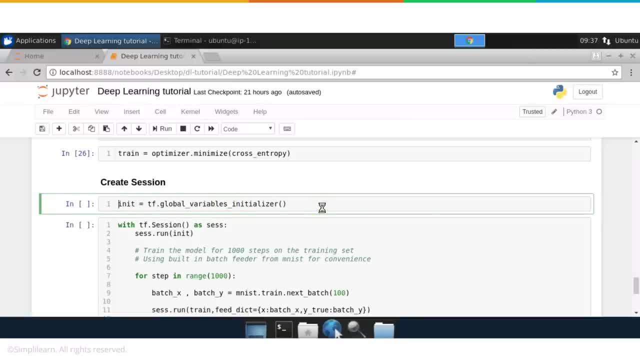 code always. So you need to basically create what is known as a node for initializing. So this is a node. You still are not yet executing anything here. You just created a node for the initialization, So let us go ahead and create that. 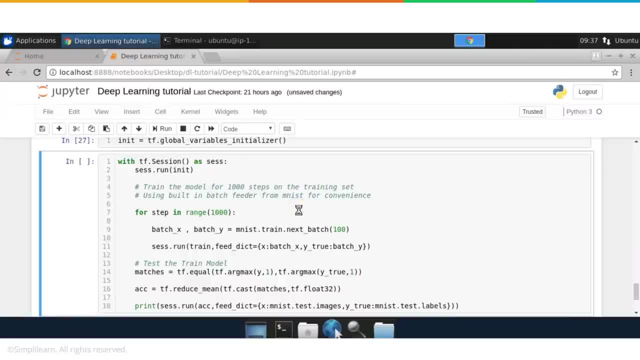 And here, This is where you will actually execute your code in TensorFlow. And in order to execute the code, what you will need is a session TensorFlow session. So tfsession will give you a session, And there are a couple of different ways in which you can do this. 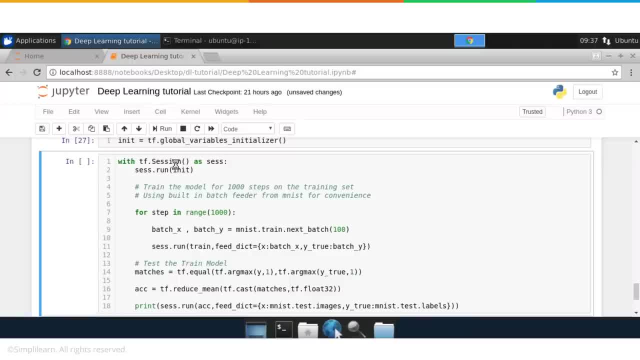 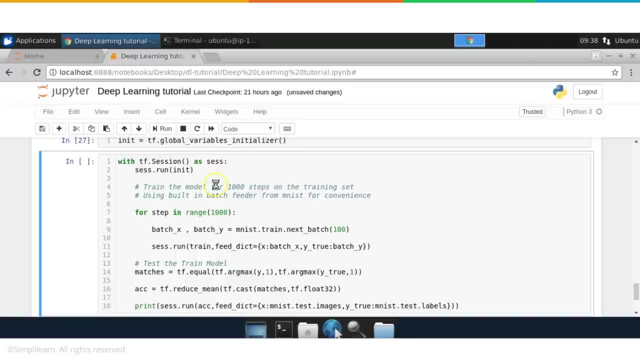 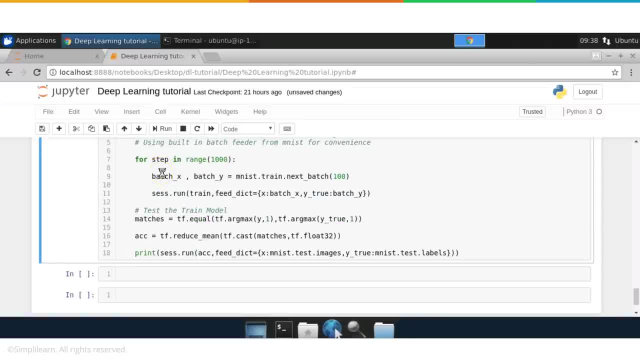 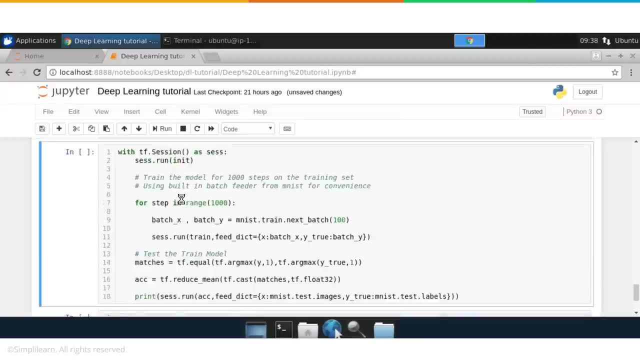 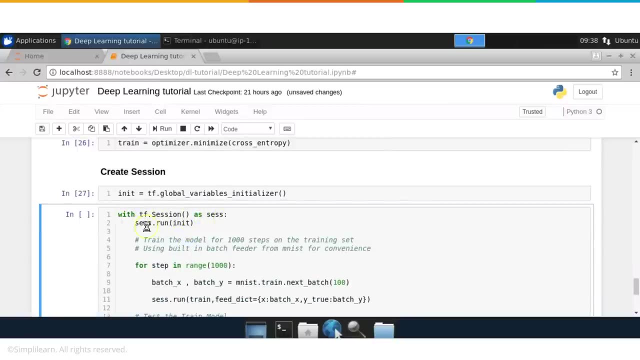 And these indentations tell how far this block goes And this session is valid till this block gets executed. So that is the purpose of creating this with block. This is known as a with block, So with tfsession as sess, you say sessrun init. 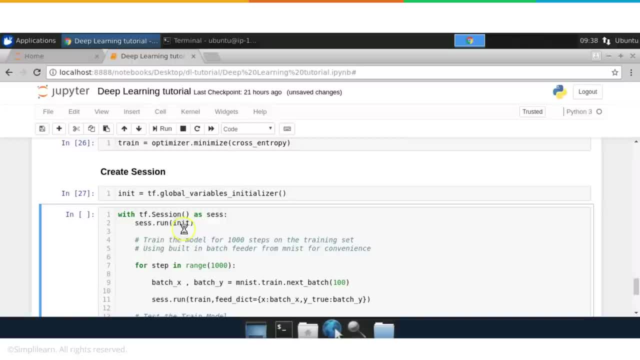 Now sessrun will execute A node that is specified here. So, for example, here we are saying sessrun, Sess is basically an instance of the session, right? So here we are saying tfsession, So an instance of the session gets created and we are calling that sess. 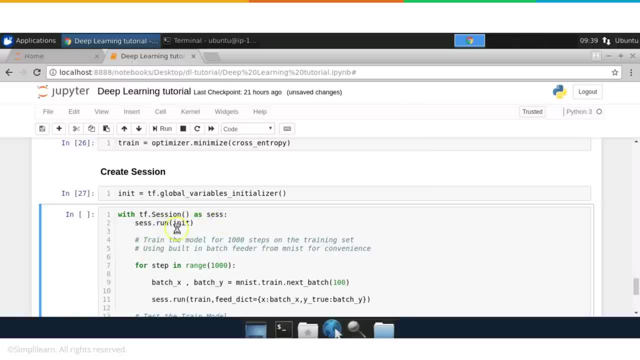 And then we run a node within that, one of the nodes in the graph. So one of the nodes here is init. So we say, run that particular node And that is when the initialization of the variables happens. Now what this does is if you have any variables in your code. in our case we have. w is a. 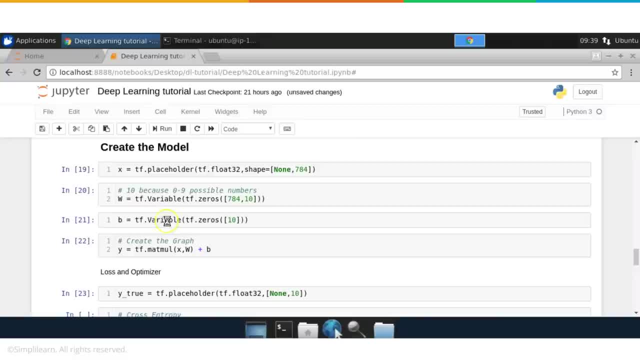 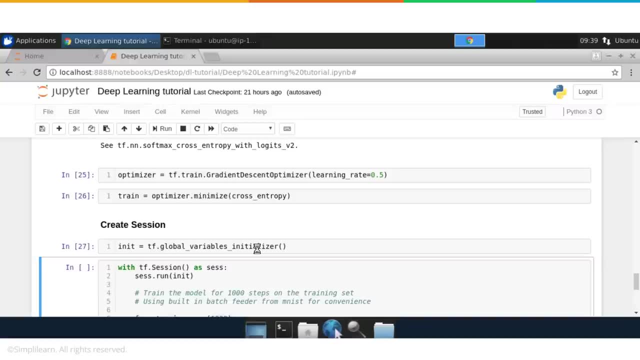 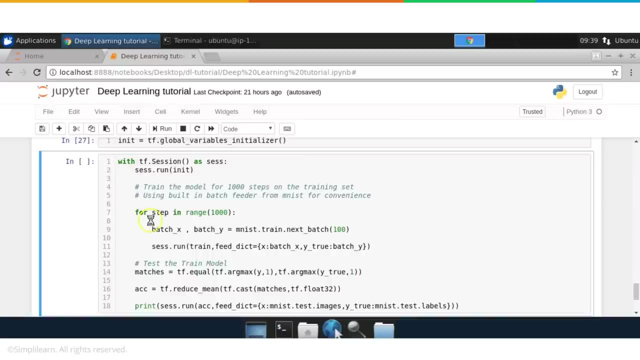 variable and b is a variable. So any variables that we created, you have to run this code, you have to run the initialization of these variables, otherwise you will get an error. okay, So that is the. that's what this is doing. then we, within this, with block, we specify: 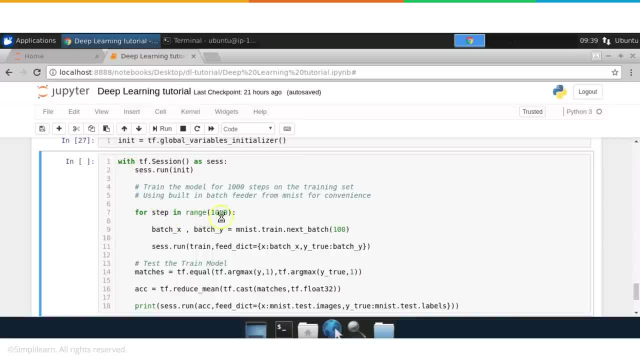 for loop And we are saying we want the system to iterate for 1000 steps and perform the training. That's what this for loop does- run training for 1000 iterations- And what it is doing basically is it is fetching the data or these images. remember there. 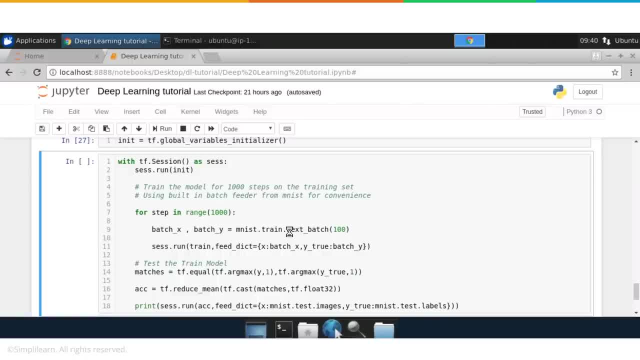 are about 50,000 images, but it cannot get all the images in one shot because it will take up a lot of memory And performance issues will be there. So this is a very common way of performing deep learning training. you always do in batches. 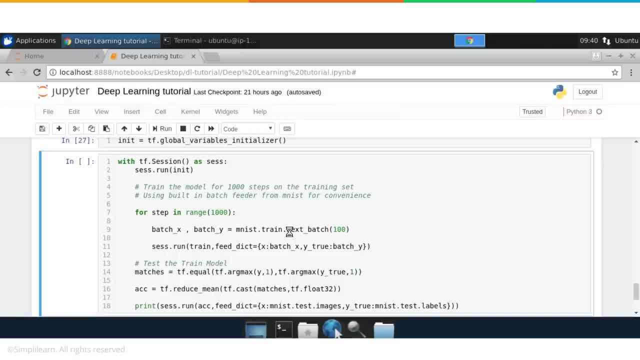 So we have maybe 50,000 images, but you always do it in batches of 100, or maybe 500, depending on the size of your system, and so on and so forth. So in this case we are saying, okay, get me 100 images at a time and get me only the. 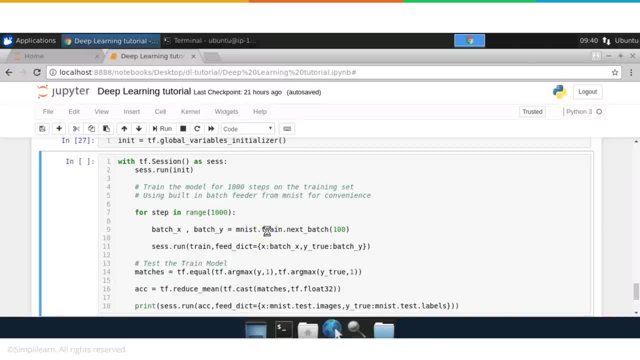 training images. Remember, we use only the training data for training, training purpose, and then we use test data for test purpose. you must be familiar with machine learning, So you must be aware of this. But in case you are not, in machine learning also not. this is not specific to deep learning. 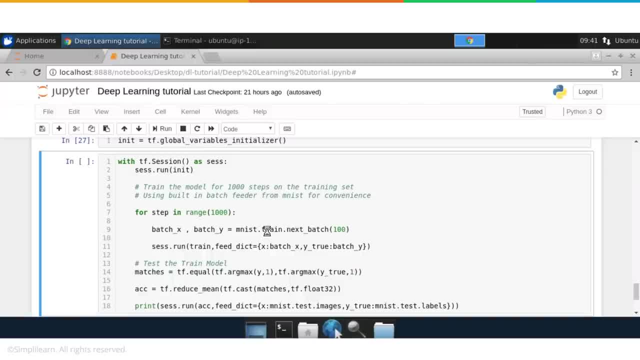 But in machine learning in general you have what is known as training data set and test data set, your available data. typically you will be splitting into two parts and using the training data set for training purpose And then to see how well the model has been trained. 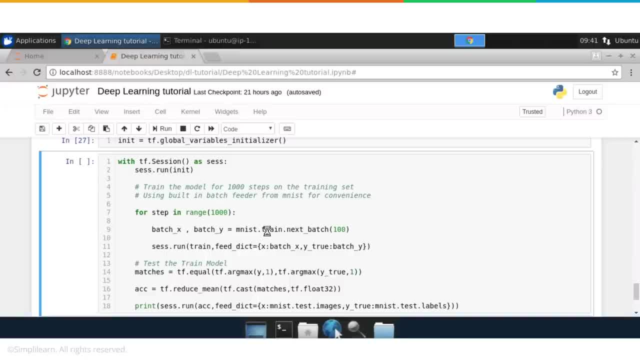 You, You use the test data set to check or test the validity or the accuracy of the model. So that's what we are doing here, And you observe here that we are actually calling an MNIST function here. So we are saying: MNIST train dot, next batch right. 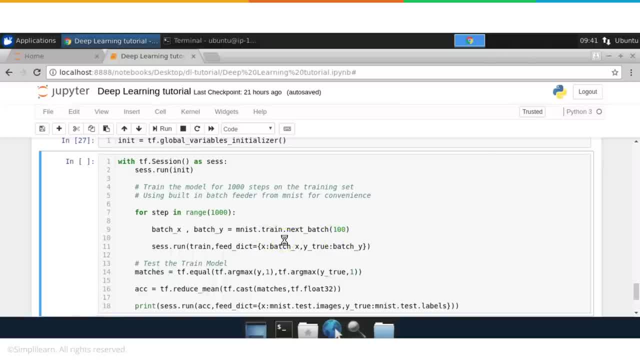 So this is the advantage of using MNIST database, because they have provided some very nice helper functions which are readily available. Otherwise, this activity itself- we would have had to write a piece of code to fetch this data in batches. that itself is a lengthy exercise. 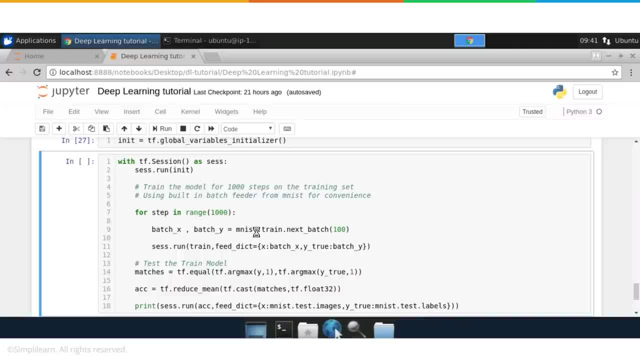 So we can avoid all that if we are using MNIST database, And that's why we use this for the initial learning phase. okay, So when we say fetch, what it will do is it will fetch the images into x and the labels. 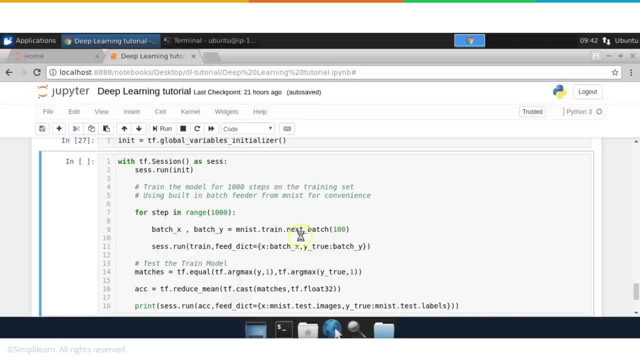 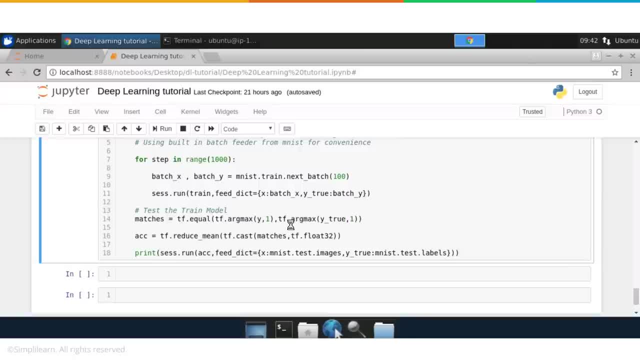 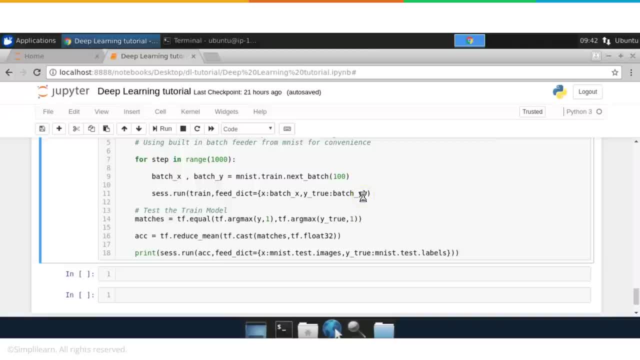 So all that feedback is given back to the neural network And thereby all the W's and B's get updated till it reaches 1000 iterations, In this case with the exit criteria is 1000.. But you can also specify probabilistic. 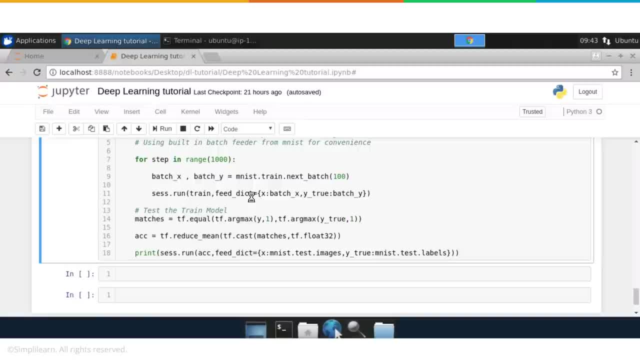 specify probably accuracy rate or something like that for the as an exit criteria. So here it is. it just says that, okay, this particular image was wrongly predicted, so you need to update your weights and biases. that's the feedback given to each neuron and that is run for thousand iterations. 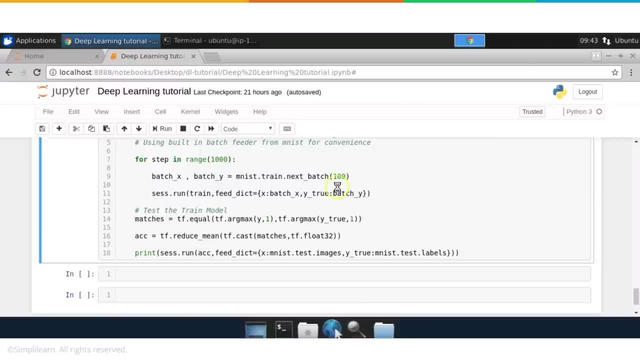 and typically by the end of this thousand iterations, the model would have learned to recognize these handwritten images. obviously it will not be 100% accurate. Okay, so once that is done after. so this happens for thousand iterations. once that is done, you then test the accuracy of 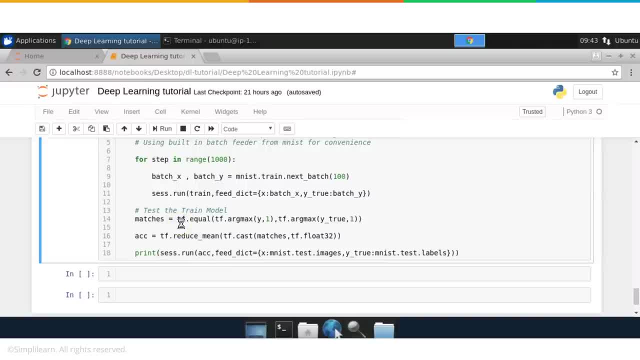 these models by using the test data set, Right. so this is what we are trying to do here. the code may appear a little complicated because if you're seeing this for the first time, you need to understand the various methods. So this is the accuracy of tensorflow and so on, but it is basically comparing the output with